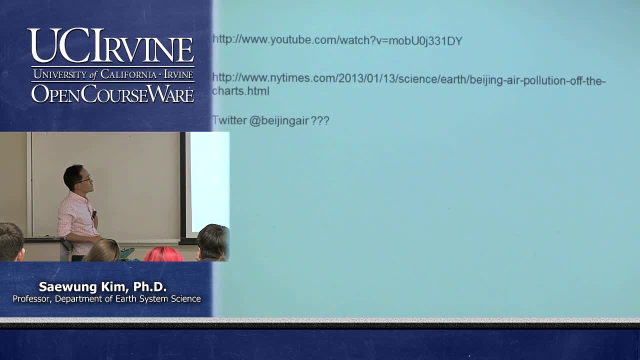 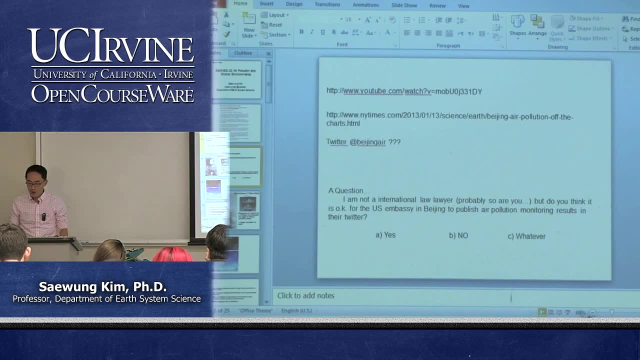 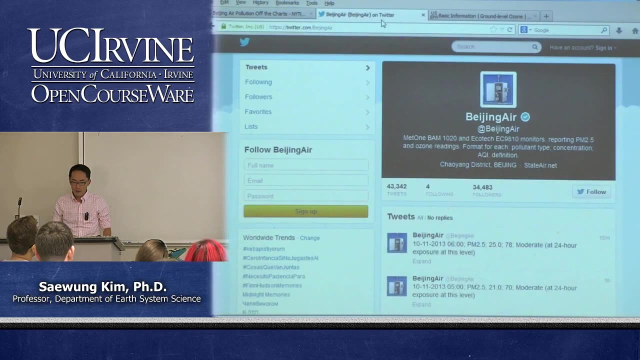 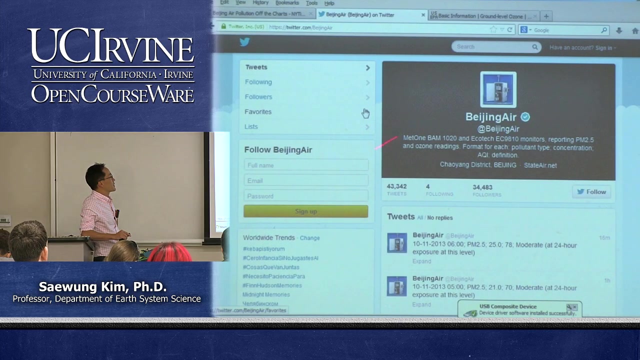 of even the little bit of diplomatic problem. That's because so this is going to be your reading assignment next week, which is a New York Times article. So, basically, what US government, US embassy in Beijing is doing is that they have little of the gadget that can measure particle concentration. 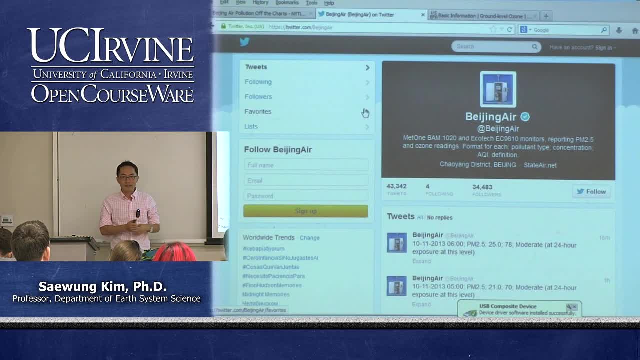 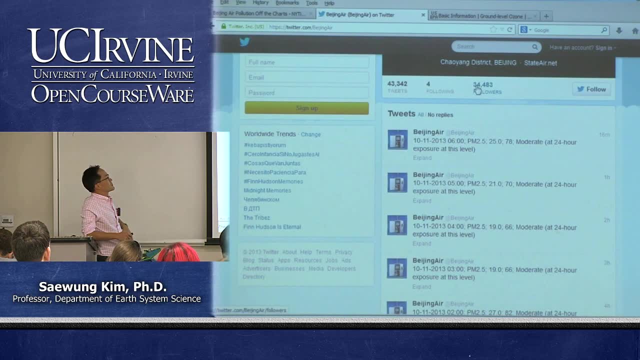 in Beijing And then they tweeted the number of concentration of the particulate matter, basically hourly basis, So this is local time, So I think they are 17 hours ahead of us. No, actually 15 hours, So 6 AM out there. 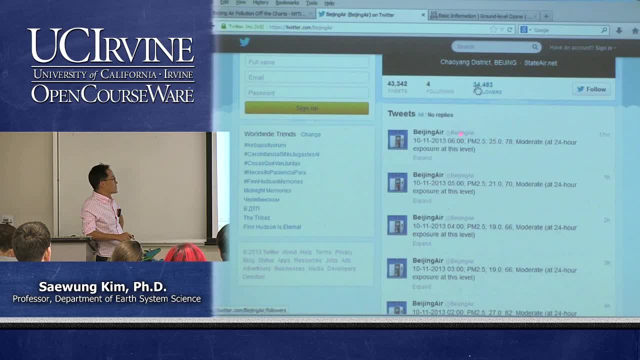 So basically, this is the real time data every hour, 5 AM, 6 AM, October 11.. And then they just put the PM 2.5.. Everybody remember what PM 2.5 means: It's the particulate matter smaller than 2.5 micrometer. 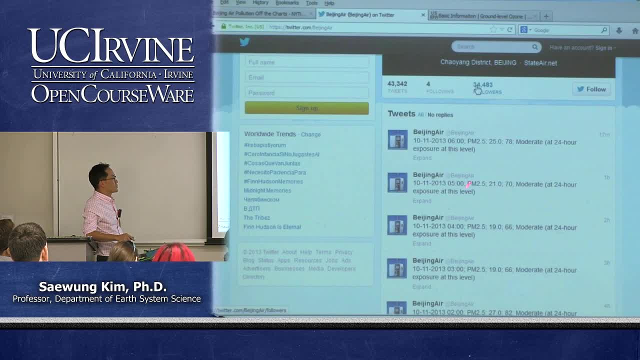 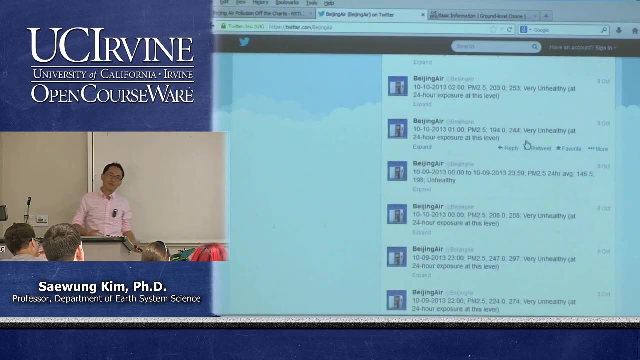 right. So they tweeted the number they observed on top of the US embassy in Beijing And then they published. it's moderate level of the pollution. It's good level, But most of the cases if you go down and down and down, it's unhealthy. 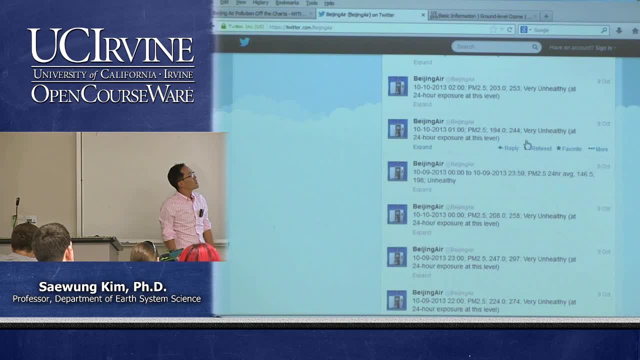 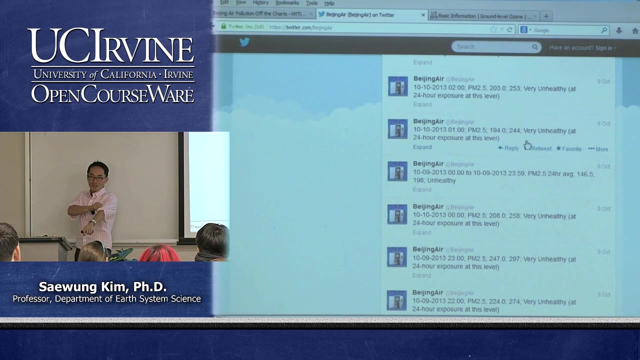 You're very unhealthy, It can be disastrous, whatever. So previously Chinese government closed the data of the air pollutants to public, But obviously people in Beijing and in every place in the world can see the Beijing air quality from data from on top of the gadget instrument that. 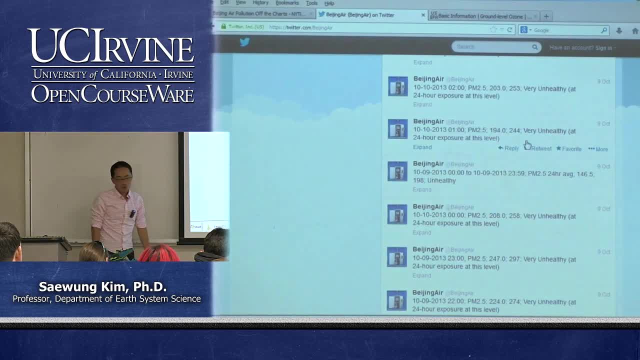 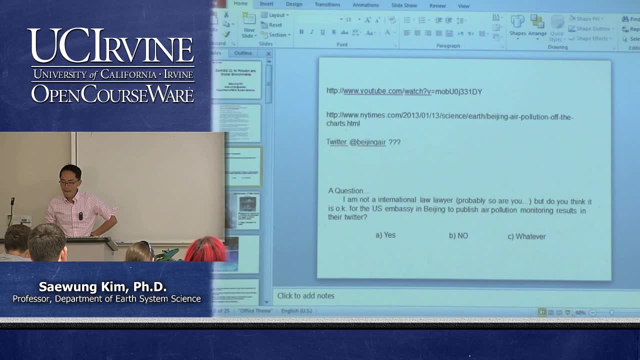 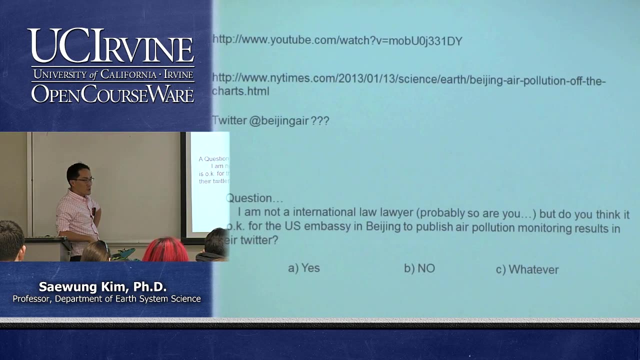 happened to be installed in the Beijing embassy. Beijing, You, The United States embassy. So my question to you is that it's supposed to be a clicker question that this thing is not functioning today also. So three times in the law. 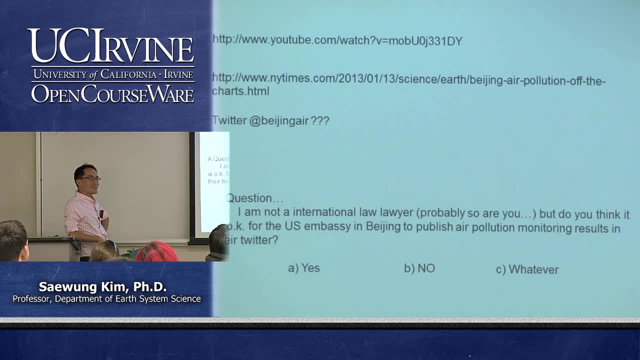 That's a shame. But my question to you is that obviously some students is leaving Immediately. they hear about that news about the not functioning iClicker. But my question to you is that: is that right or wrong that US government actually have a little instrument? 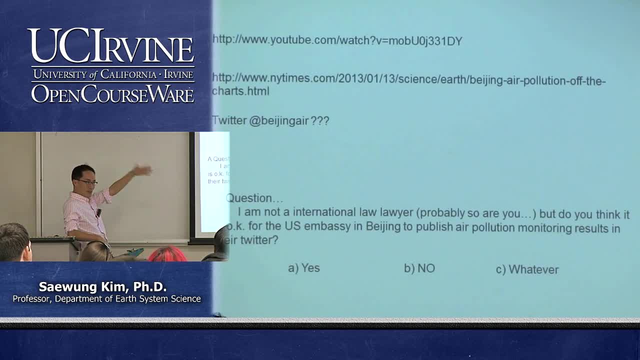 on top of their embassy and then publish that data to public. It can be a little controversy And then this news article is actually talking about Chinese government officials complained about US publishing the data about the air quality, about Beijing. So iClicker is not working. 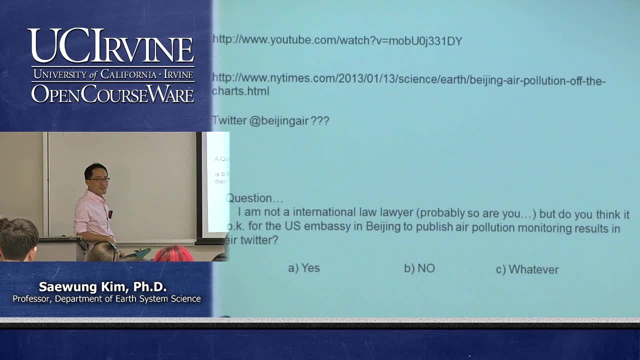 But let's see, Let's see, Let me hear your voice. What do you think It's the right thing to do or wrong thing to do? Anybody want to talk about it? Nope, No opinion, Whatever. Back there. 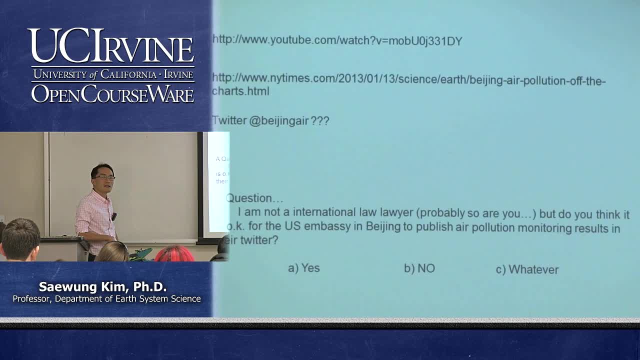 Well, if you guys wouldn't be the one posting, other people would be posting on the internet too, right? That's true. But probably my question is that: is that right that other people from the other country get into China and then doing the you? 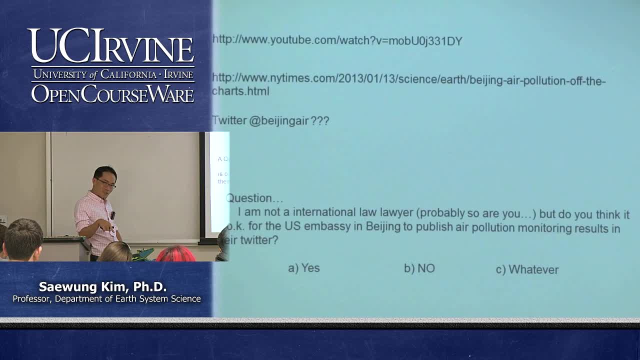 know air quality measurement and then doing the air quality measurement and then publish that data to the internet. probably That's the question. Go for it. Go for it, You can just talk. I think it's okay because it's like: 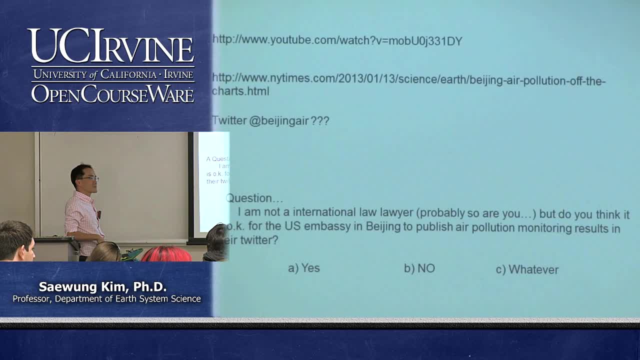 a human health issue. OK, If people say, if people say: are they capable of travelling to Beijing or they deserve to know this before they can make their decision? I'm hoping that's something that will become free in China's phone conversation. 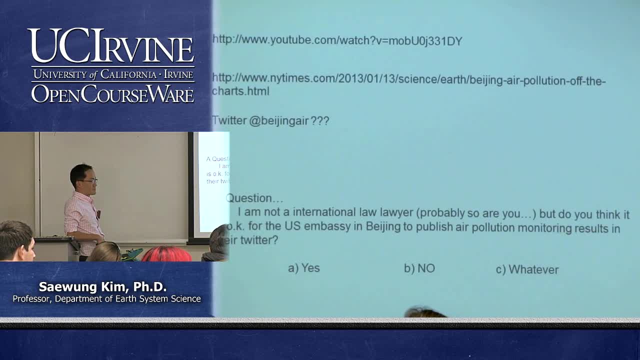 Yeah, thanks, Bill. Yeah, I think that argument behind the US logic behind this Twitter account is that to the other people, so American citizens who travel in China, need to know how bad it is air quality so that they can aware that what they should do on the street, things like that. 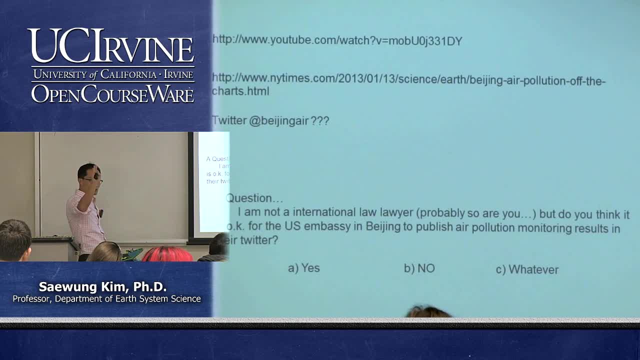 So that's the one argument. actually, Any opposition towards that. that's not the right thing to do. No, So everybody think that that's the right thing to do. Yep, I'm not saying that it's not that it isn't not right, but obviously the US might. 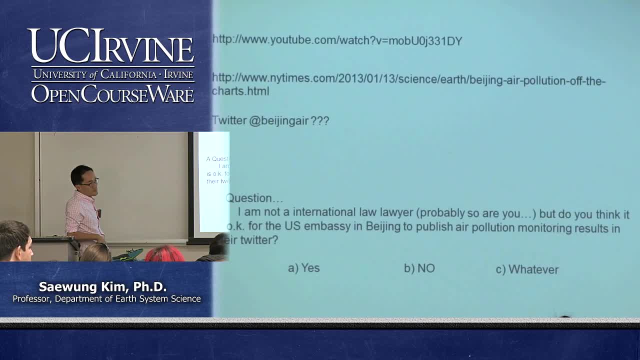 have something behind it doing that, because US and China relations are getting kind of tense and China is a developing country. they're still industrializing, which the US did like 100 years ago and it was posting. you know how bad the air pollution was back then. 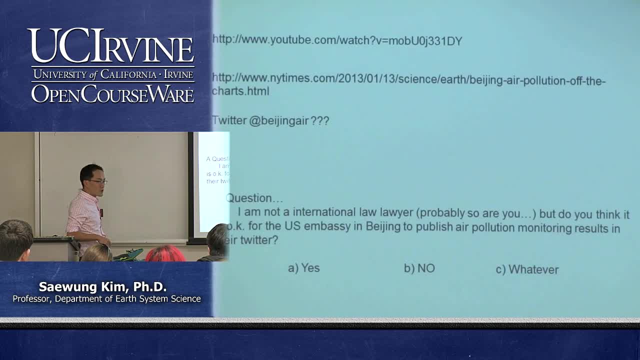 Yep, Yep. So yeah, that's, you can have your own opinion. so there are two scrub thoughts out there. Actually, even bigger problem at that time was that actually the number from this Twitter account, and then what Chinese official number that Chinese government published to the public? 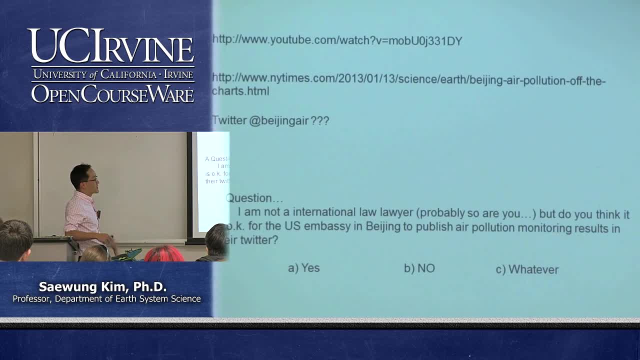 that's the difference. It's actually Chinese. numbers was much lower and then that was the big problem. So you can read this article That I will just put on there for this week's reading assignment And then so think about what's the you know whether it is good thing, right thing to do. 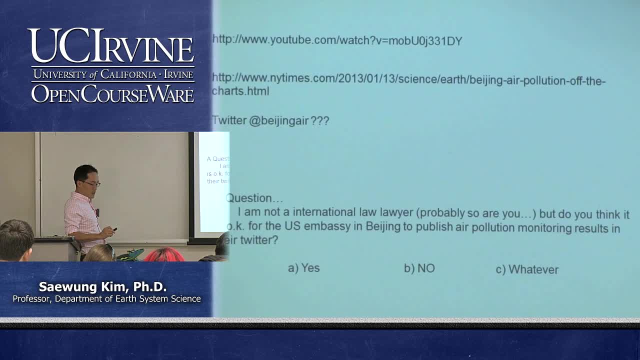 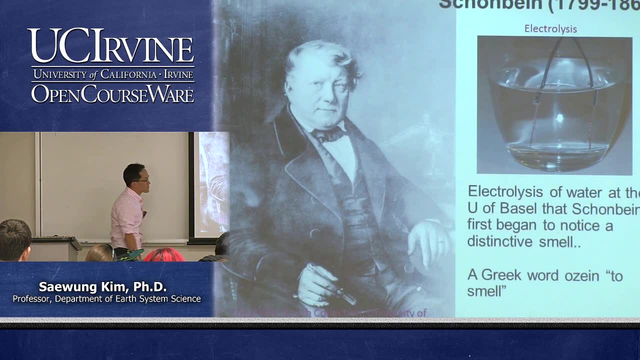 or you know wrong thing to do things like that. So this is kind of a thought, something like something you can think of speculating of that in terms of the science, environment, and then even the little bit of diplomatic issues. 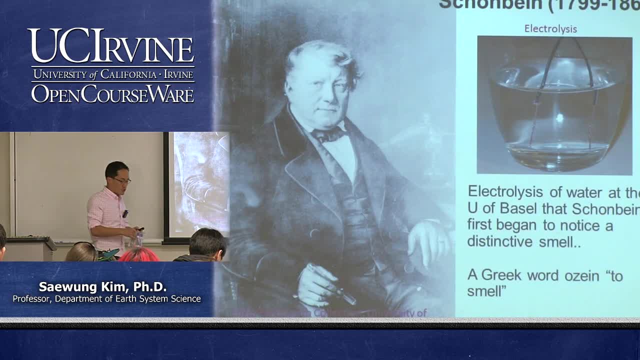 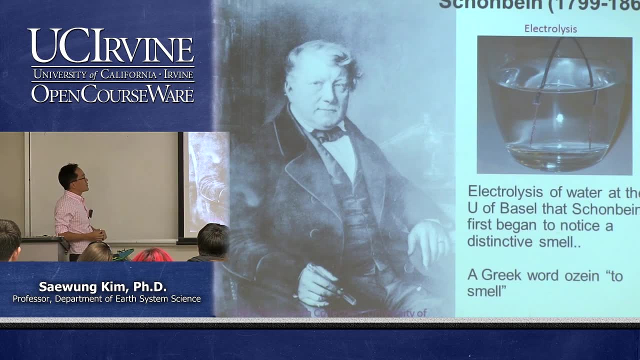 things like that. So today and then next lecture we'll talk about the ozone. So I think during first class I introduced this guy chemist who first found ozone by doing electrolysis of the water and then he just smelled something and then he just first called it ozane, in Greek word to smell. So basically, once ozone concentration gets high, actually you can smell that ozone concentration and then over and over and over again I talked about there are two kinds of ozone in the atmosphere. 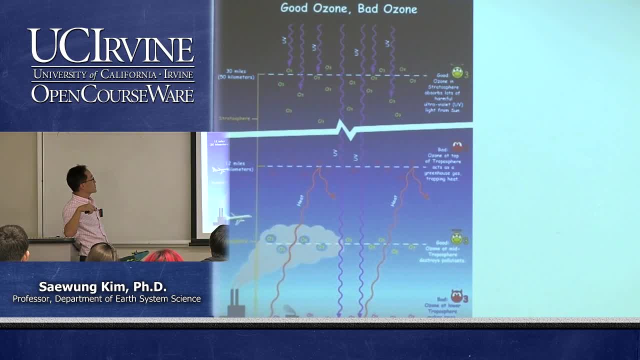 One is the ozone on top in the throughout sphere. That's good ozone because it absorbs UV energy from the sun, so that this layer of ozone protects us from the harmful UV, But once it's formed on the surface, the air we breathe. 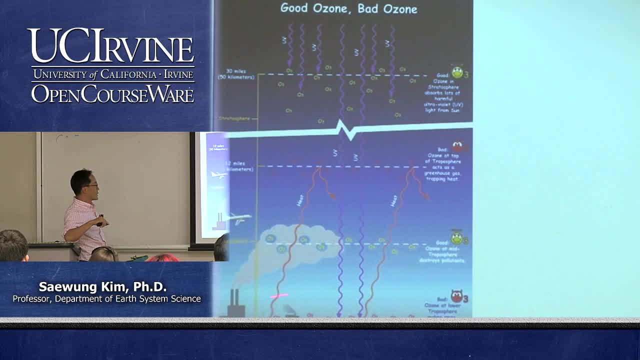 so that's the bad thing. So we'll talk about next two lectures, about this ozone in the lower in the atmosphere, what you call it troposphere- and the chemistry behind of this ozone forming photochemistry. So how many of you actually took the chemistry in high school? 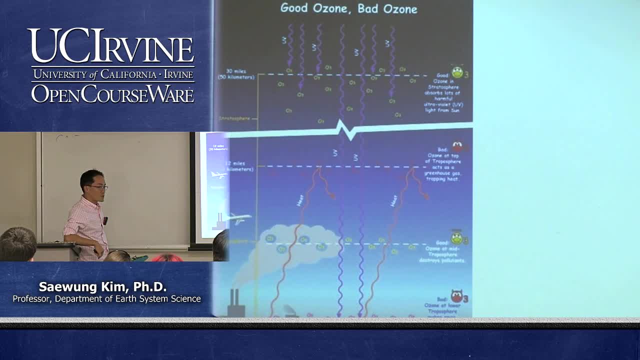 So most of you, How many of you actually heard about chemical bonding? Most of you Covalent bond. So how many of you actually not heard about the covalent bond? I have no idea about the covalent bond or bonding. 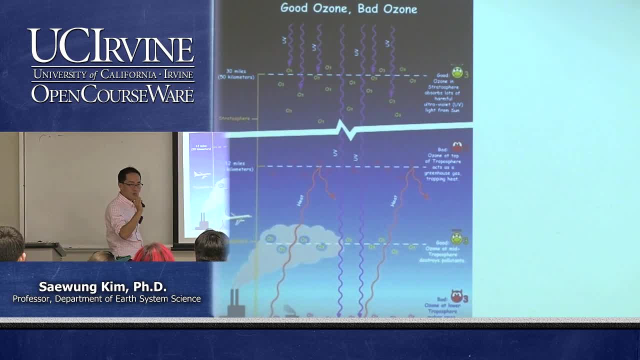 Don't be shy, You're fine. So everybody heard about it. Okay, that's good. So we will talk about mostly chemistry today, But we will go over and over again if you don't have a clear understanding about the reaction that I introduced today. 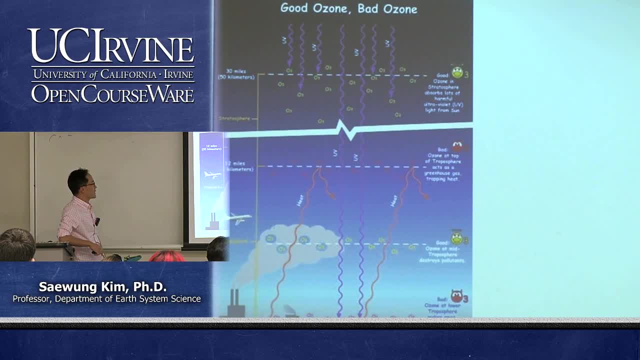 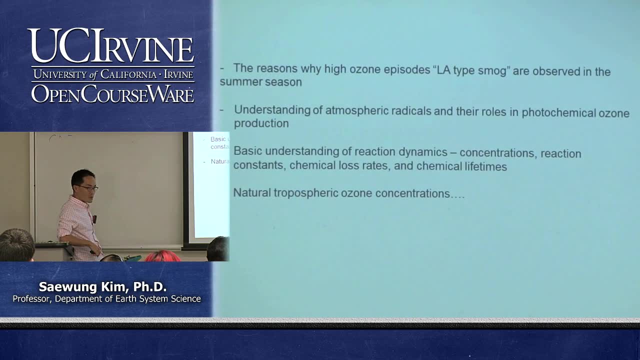 So don't be panicked and freaked out things like that. So last lecture we talked about the London-type smog. right Today we will talk about LA-type smog. It's a completely different thing. And we'll talk about photochemical reactions. 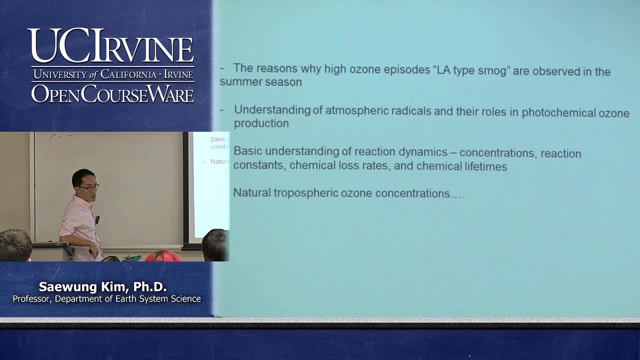 To do that we need to understand rules of radical. So radical by definition it is a very reactive molecule in the atmosphere, And then this triggers a lot of reactions in the atmosphere. Eventually it is forming ozone in the atmosphere. So again, ozone is not directly emitted. 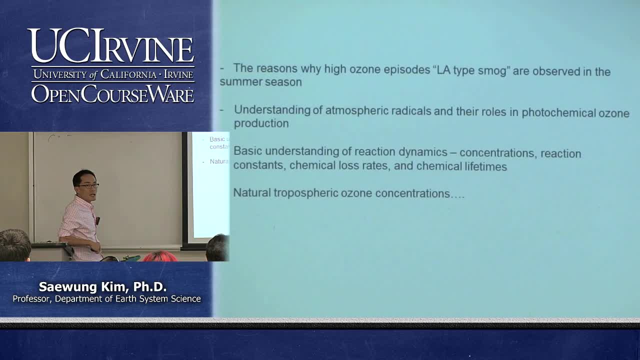 to the atmosphere by human activity, rather formed by the chemical reaction in the atmosphere. So we will talk about, we will kind of discuss about kind of exploring about the chemical reaction in the atmosphere, And then today mostly we will talk about natural tropospheric ozone. 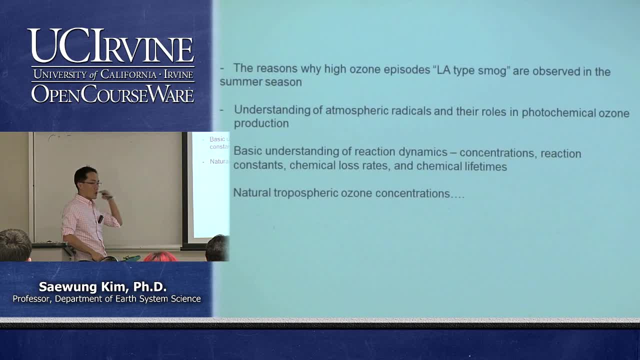 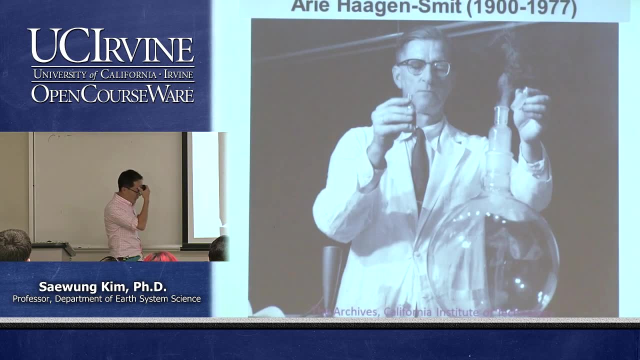 which means that before human perturbation is there? what kind of the ozone concentrations are actually there in the atmosphere? So I showed this photo. This is Ari Huggins-Smith. Actually, he developed the chemical mechanism that ozone is forming in the troposphere. 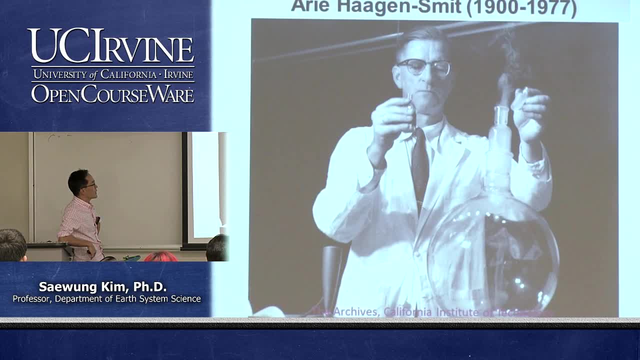 So he was a professor at Caltech And then he actually published the first paper who is kind of explaining that ozone forming photochemistry in the troposphere. So maybe this back in 60 years. this is how people are doing experiments, wearing nice neckties. 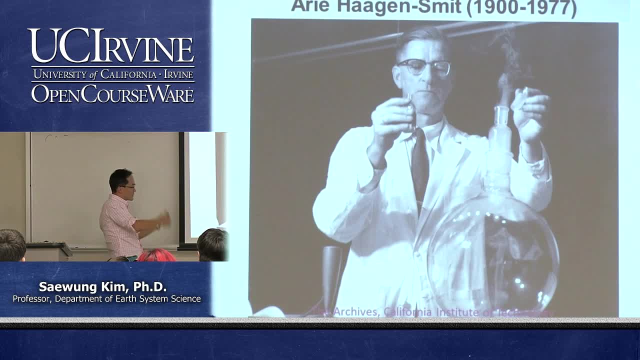 things like that nice gown. But that's the one thing that you can learn from this photo. But the thing that I really want to convey from this photo is that, basically what he's doing, I'll show you. you can see there, this white fume is coming out. 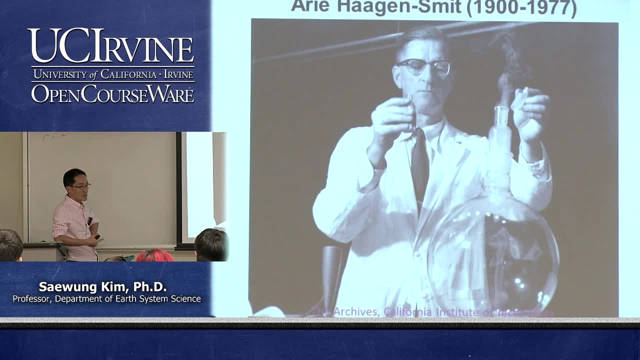 That can be either a particular matter or ozone. If ozone gets very high concentration, actually you can see a little bit of color, things like that. So what he's doing in here is that in this glass jar he's just putting some of the precursors. 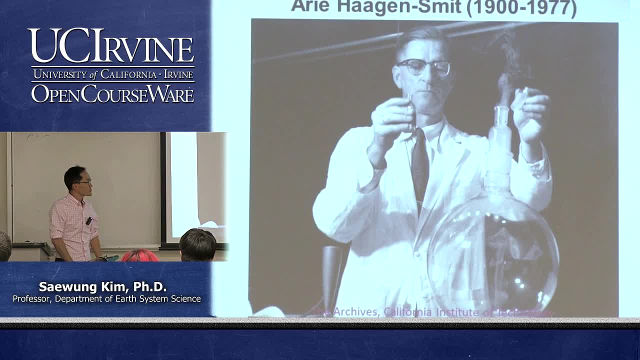 pollutants from the human activity, in this case the exhaust from the cars or the industrial facility. He's putting that thing in here, making some reaction, and then actually the ozone is forming in this glass jar. So this is kind of you can think that this is kind of a mini-atmosphere. 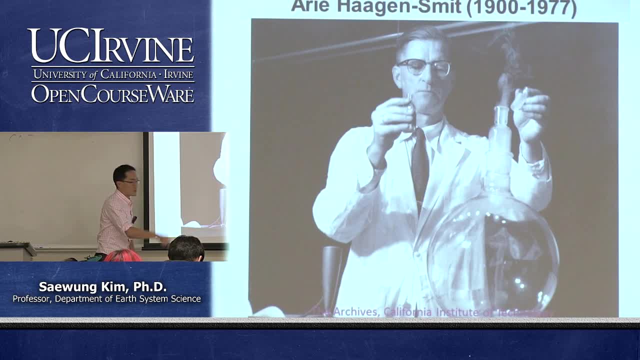 and actually the reaction is happening in here. So again, ozone in the troposphere. it's not directly emitted from the human activity. rather, something is formed in the chemical reaction in the air. So that's one of the messages that I want to convey from this photo. 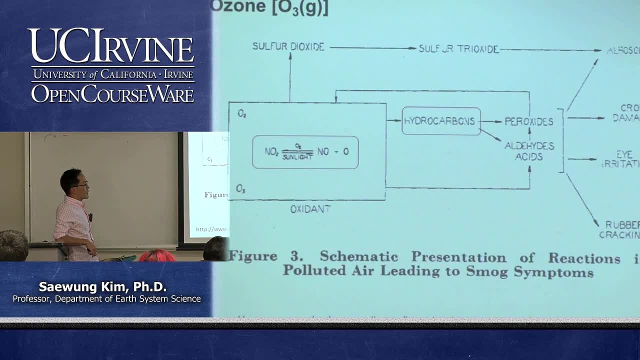 So this is the paper that he published in 1952.. So again he talked about NO and NO2, which is coming from a kite JOST, that we discussed about it, that in the atmosphere there's a major component. 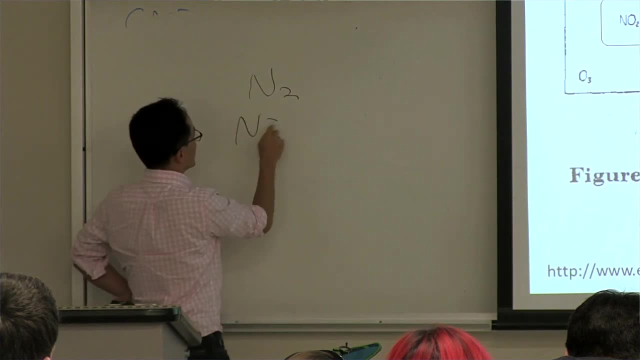 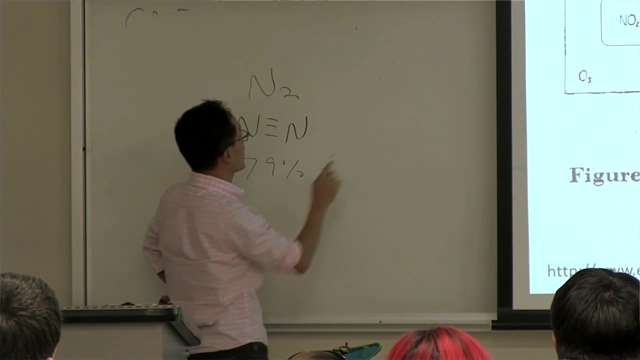 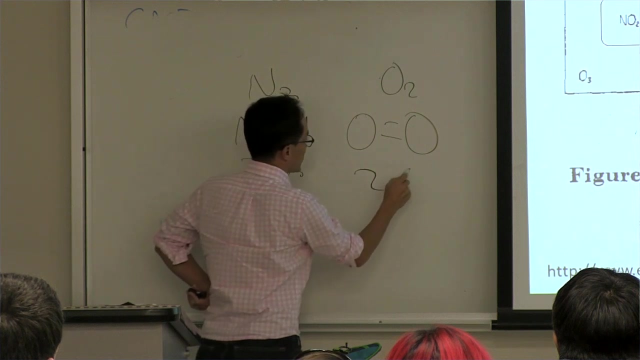 gas molecule is nitrogen, which happens to have triple bonding, which is very stable. So this is about 79% of the air right, And then O2, it's just double bonded like this, which is about 20% of the atmosphere. 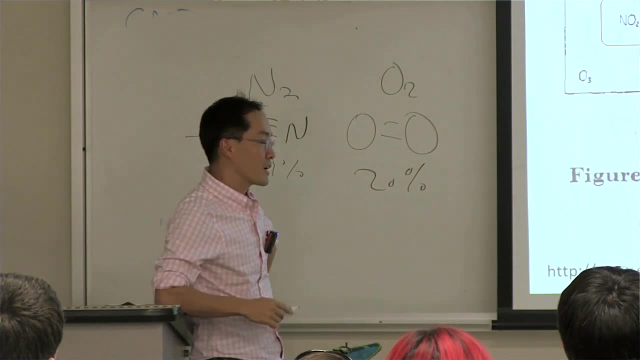 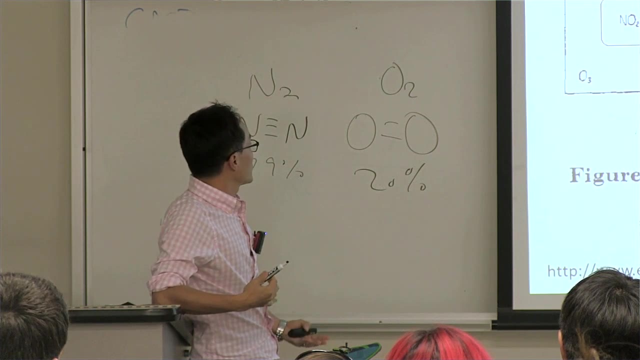 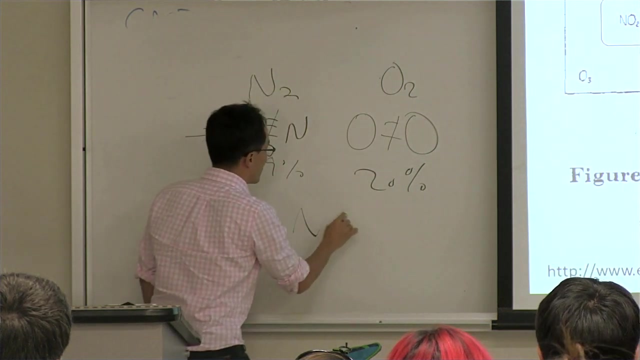 So these are super stable molecules that are not really participated the chemical reaction in the atmosphere. But in the car engine its temperature gets high enough the bonding can get broken up, then make NO. So this is nitrogen oxide. So this is very important precursor. 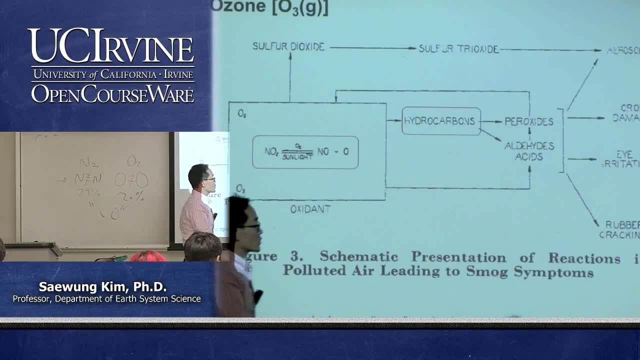 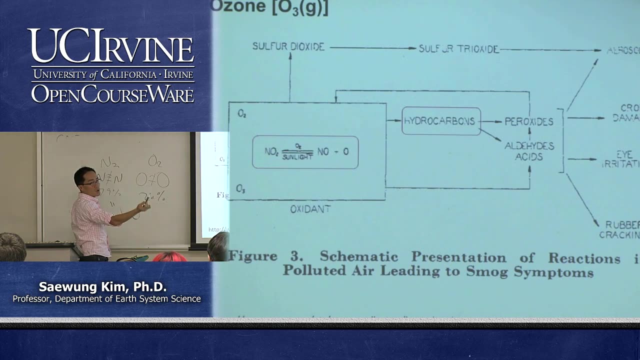 for the ozone formation. And then another important precursor is hydrocarbon. So hydrocarbon, by definition carbon and hydrogen, So we call it the compound composed by carbon and hydrogen. we call it organic molecules, right And then? so this is another word. 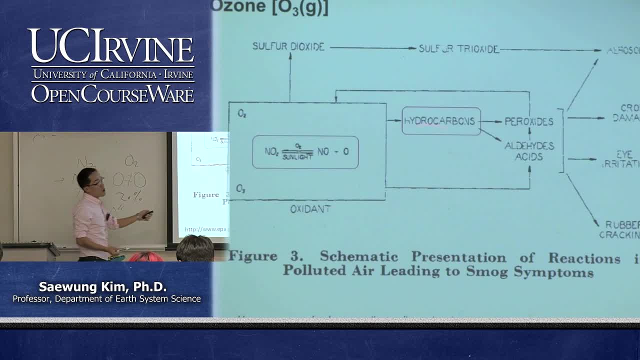 of the organic molecules And then the hydrocarbon in the atmosphere. because it gets in the atmosphere it gets evaporated. that means it's very volatile, right? So from this, from this class, we will call this kind of hydrocarbon. 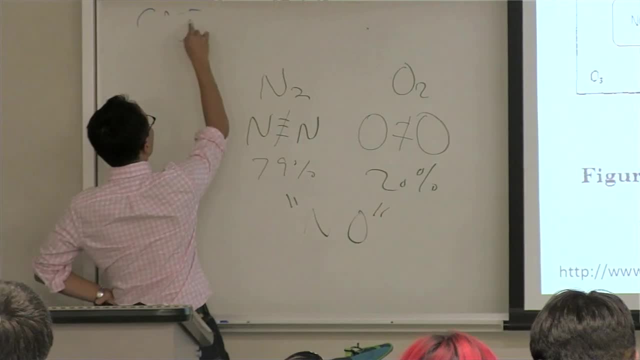 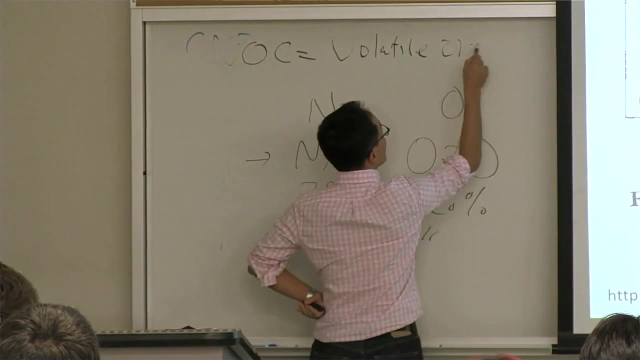 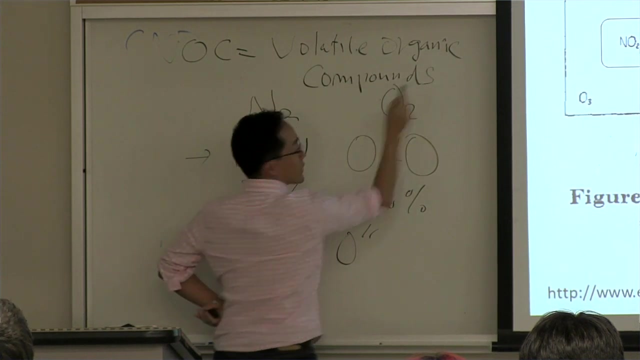 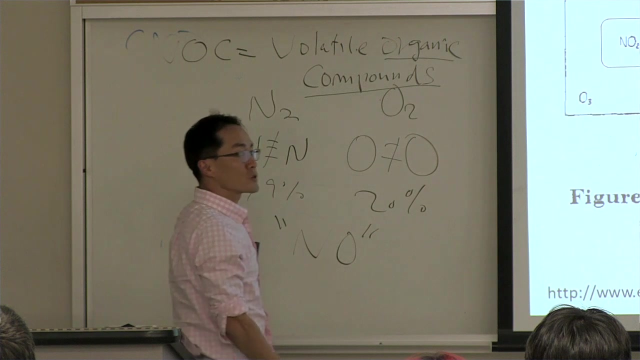 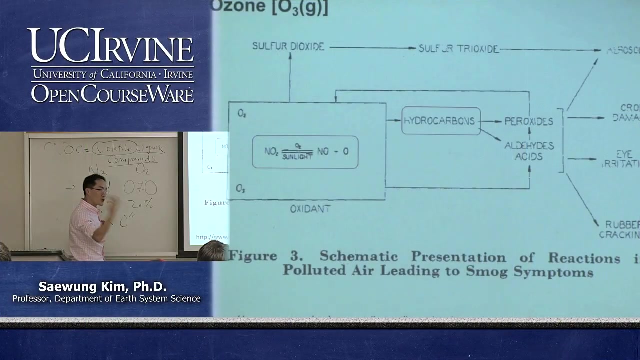 in the atmosphere as VOC, which is volatile organic compounds. Right, So we discussed about what's organic compounds are, which is composed by carbon structure molecule, And then- this is a characteristic of that specific organic compound- happens to be volatile and then gets into the atmosphere. 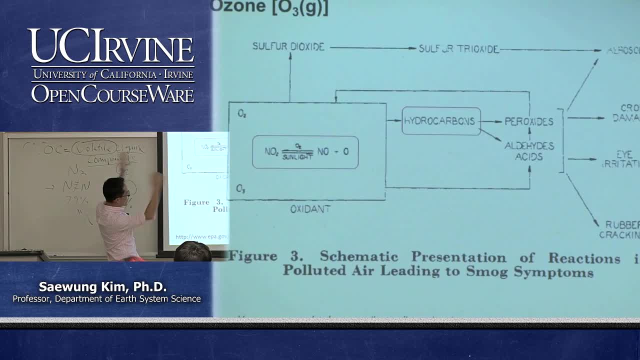 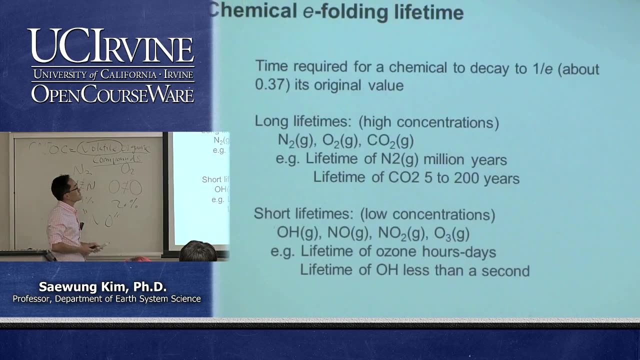 Okay, So basically the and then the reaction is going on, and then these primary emission from the human activity making ozone and aerosol. So that's by definition a late-type smog. Okay, So we briefly talked about chemical lifetime. 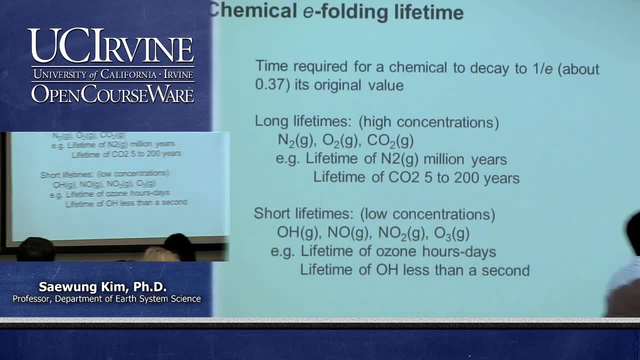 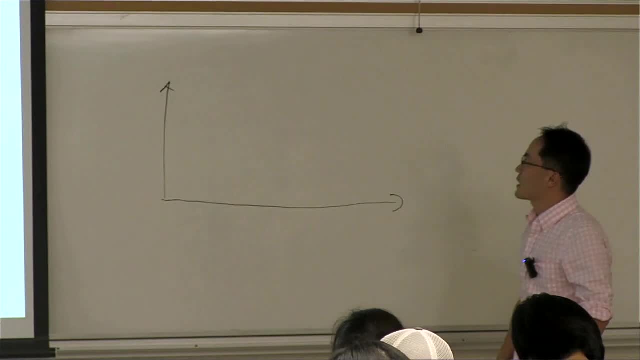 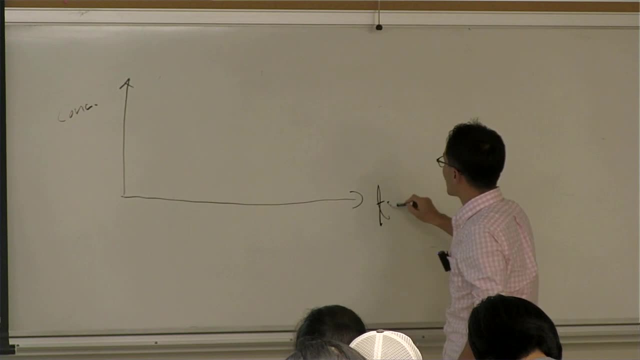 I think for the first class. So we love to make plots, Scientists love to make a plot. So from here let's say: this is concentration of some chemical species, and then this is time Right. So we talked about. 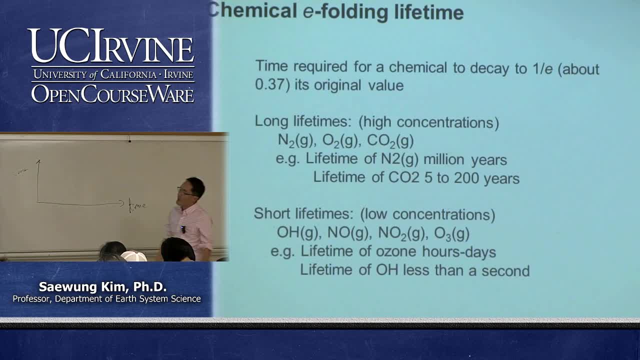 once the pollutants such as NO1, NO2, and then VOCs are emitted to the atmosphere, they are reacting each other, and then they are reacting each other and then forming ozone right. So that means some pollutants that initially people emitted. 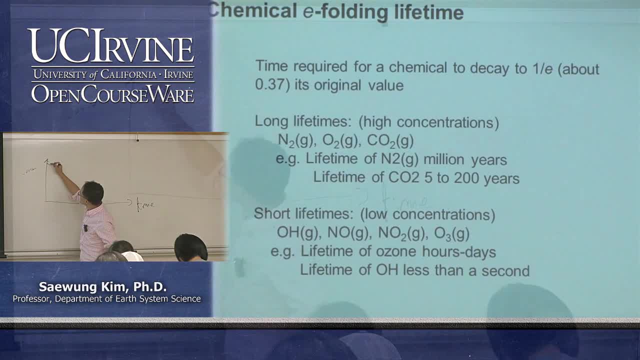 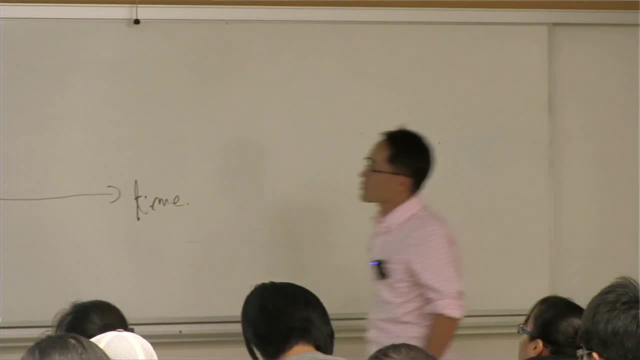 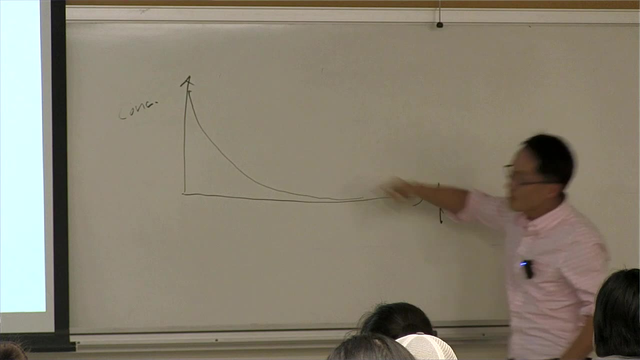 those kind of air pollutants, then concentration is going to be high. Then once it reacts with some other molecule in the atmosphere, then the concentration is going to be decreased, like this right. So eventually, if it is reactive enough, then all the compound. 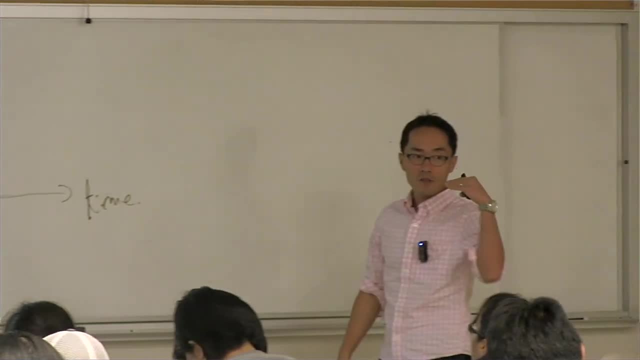 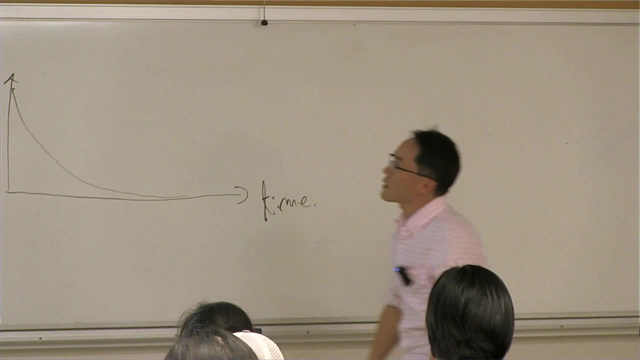 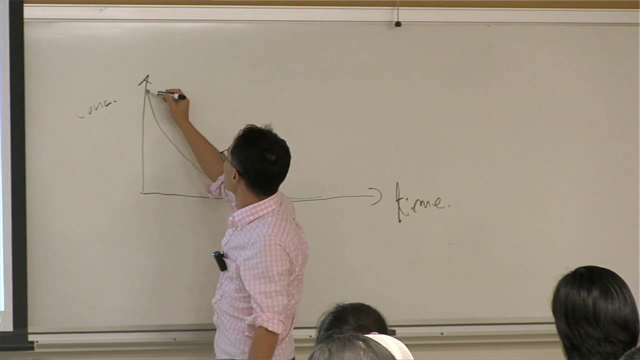 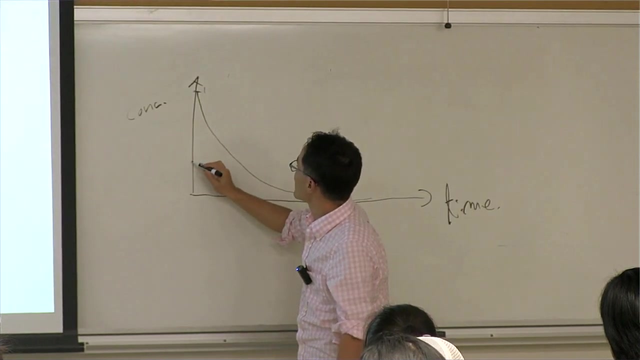 is going to be removed from the atmosphere if emission stopped in some time, point right. So when we call chemical lifetime, that means we just define. the definition is that when let's assume this is concentration of 1, and if it is removed? 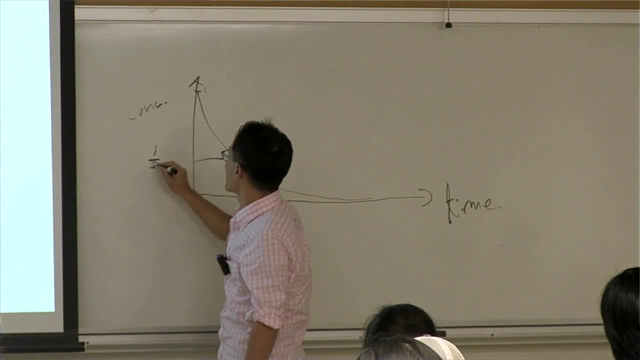 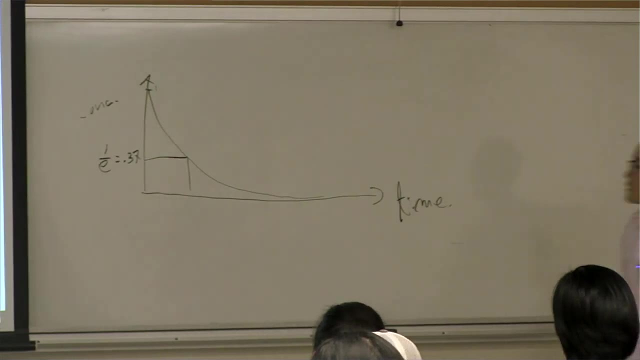 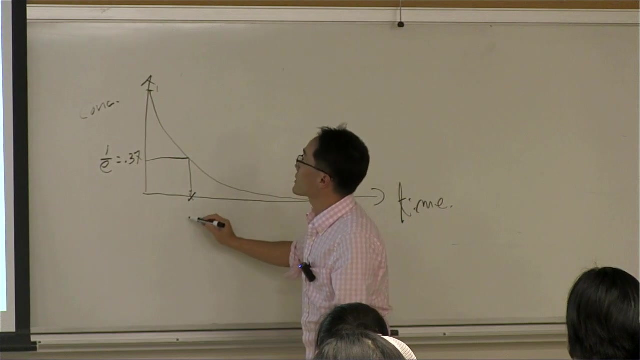 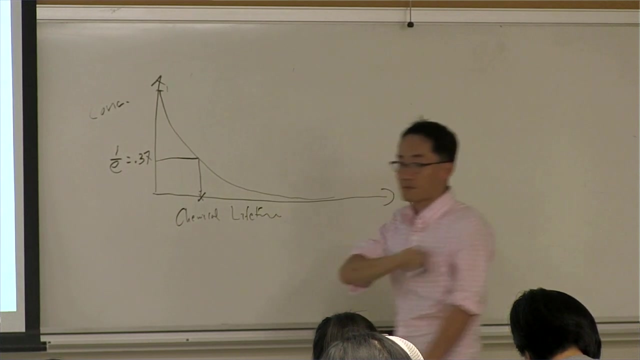 until 1 over E, which is about 0.37.. So if there's a all just reacted away and then 37% left, that time right here we call it chemical lifetime. Okay, That's just definition. 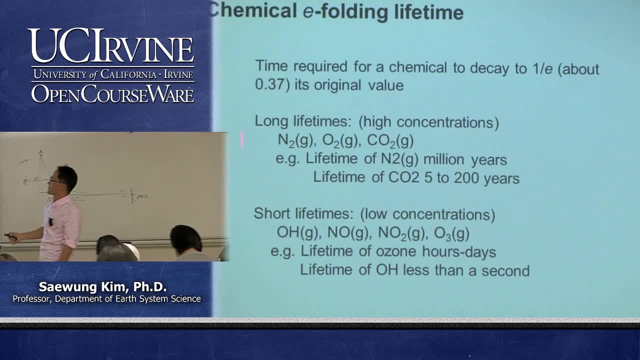 So some of the long lifetime species such as nitrogen and oxygen. then I explained that they are very stable in the atmosphere because those molecules satisfy octet law and then it has triple bonding and double bonding. they are super stable. So that means they have a long lifetime. So, for example, nitrogen- nitrogen lifetime in the atmosphere. So if there's a process just producing nitrogen, just stop and then it takes about million years to about 63% of nitrogen is going to be removed. 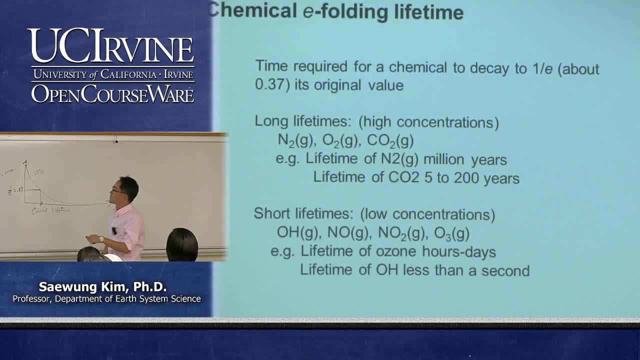 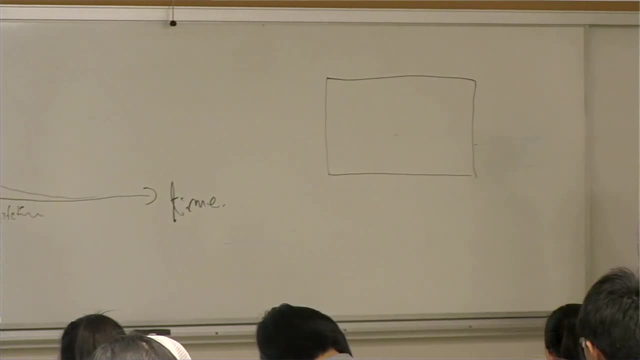 from the atmosphere. That's by definition of the chemical lifetime right. So so these compounds, the long lifetime compounds, a stable compound, and then again, the other thing we talked about is that we atmospheric chemists love to kind of conceptualize. 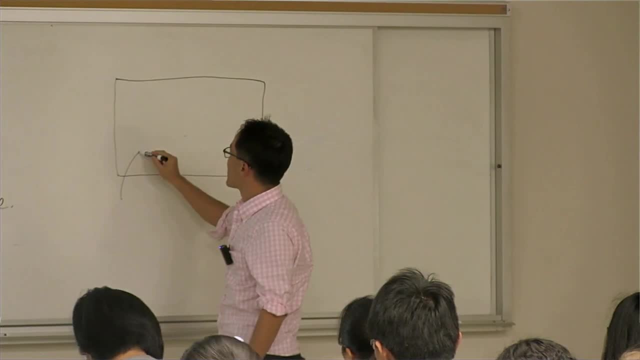 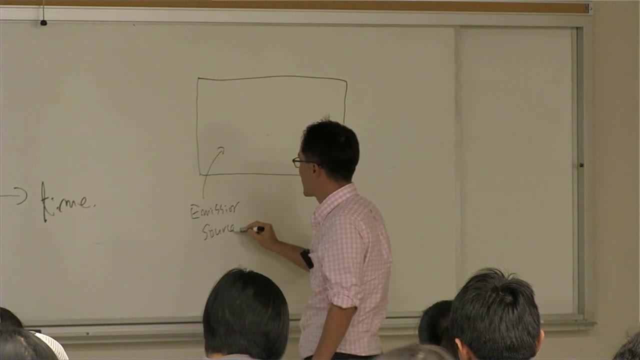 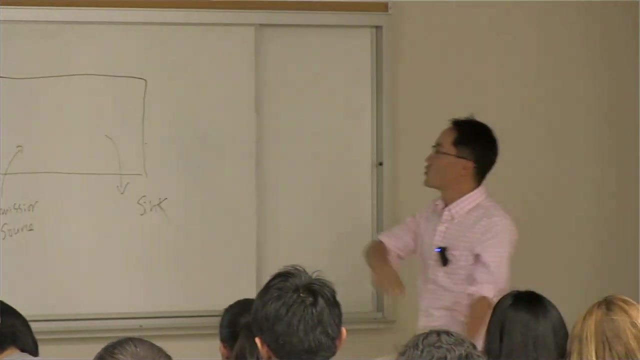 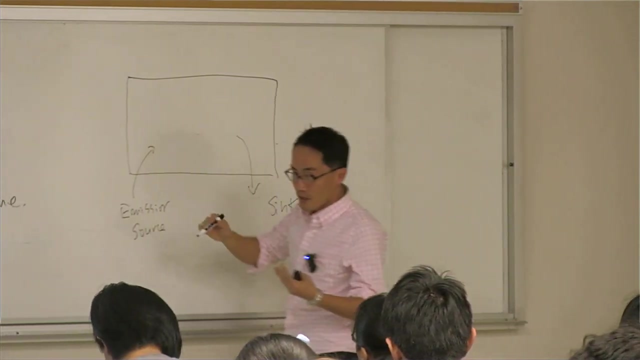 atmosphere as a box, and then there's emission or source, and there's a sink. Some of the gas pieces should be removed from the atmosphere, the box in here. And then the thing we are going to discuss about, we are going to discuss about today: 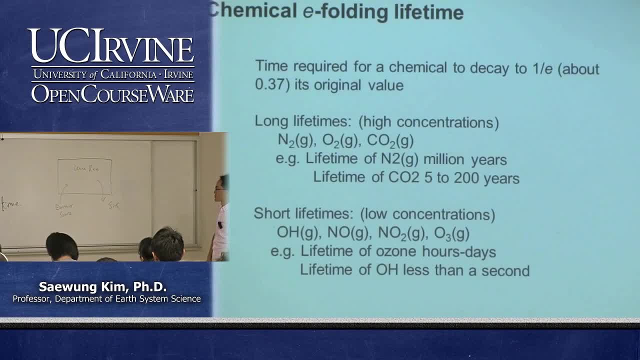 is the reactions. So basically, if you have a very stable compound, long lifetime compound, that means that it's going to be accumulated in the atmosphere for the long time, because this process that removes that specific chemical compound from the atmosphere is very slow, right? 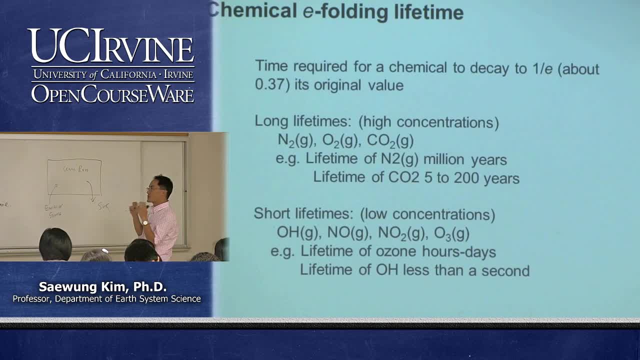 So you can think that it's the same thing By definition. when compounds are very stable, then its lifetime is going to be very long and then the concentration of that specific compound is going to be very high in the atmosphere, right? 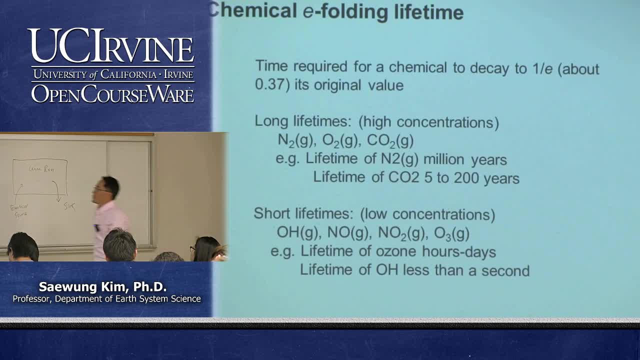 So they're all the same concept, But in terms of the, in terms of the air pollution perspective or atmospheric chemistry perspective, these are not really important because, by definition, they are stable, right. So short lifetime species. 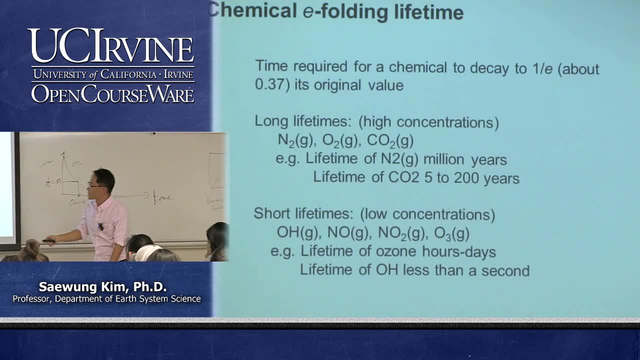 like NO and NO2 that we talked about here. the NO is coming out here, So NO and NO2 kind of interconverted each other. That's something we are going to discuss today. And then ozone has. they have a relatively short lifetime. 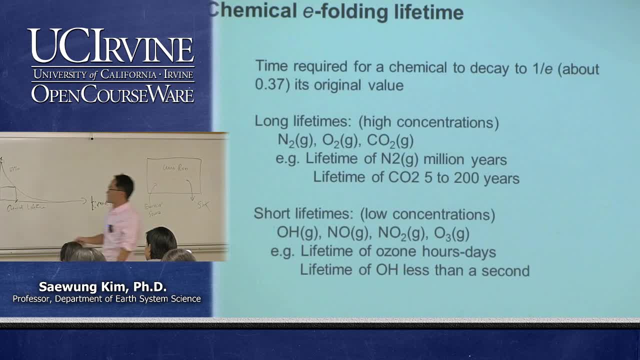 from hours minutes. Some of the species which we call it radical has a lifetime less than a second. So these compounds have short lifetime, which means they are reactive, and then the and then the atmosphere concentration is very small because 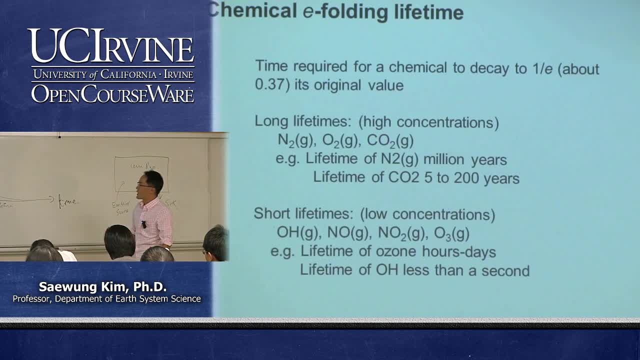 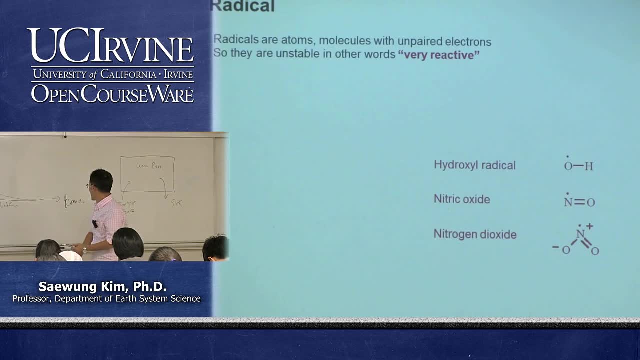 they are quickly reacted away in the atmosphere with the other molecule in the atmosphere. So that's the concept, right? So radical, Ooh, it's actually sliding. So you can basically think radical is very reactive species. So the chemical background. 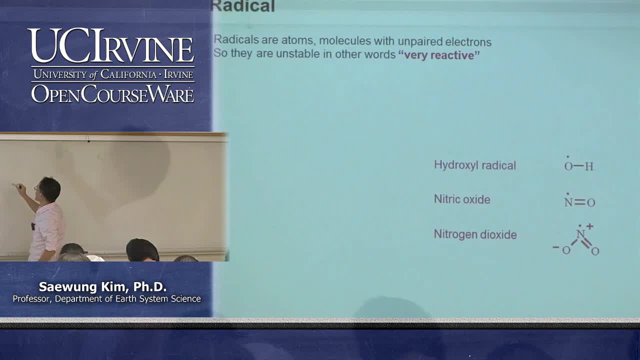 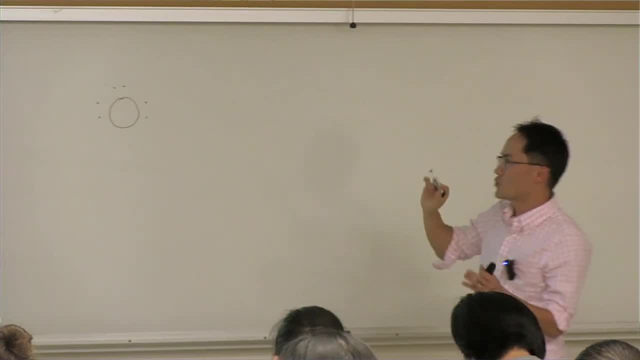 why they are very reactive is that, for example, the hydroxyl radical, so it has six electron outer shell. but you don't need to, you don't need to know about the, this chemical, actual background of of this radical. 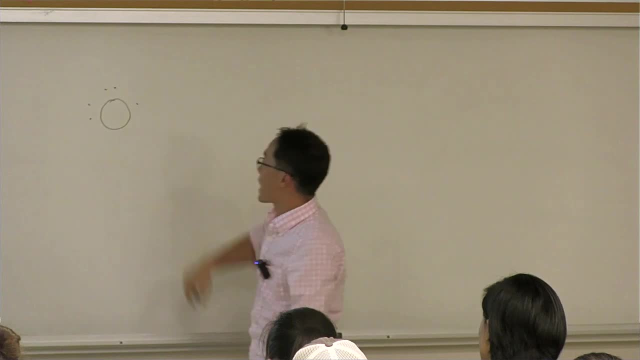 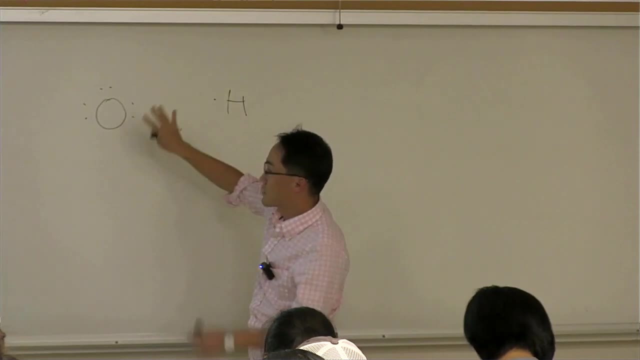 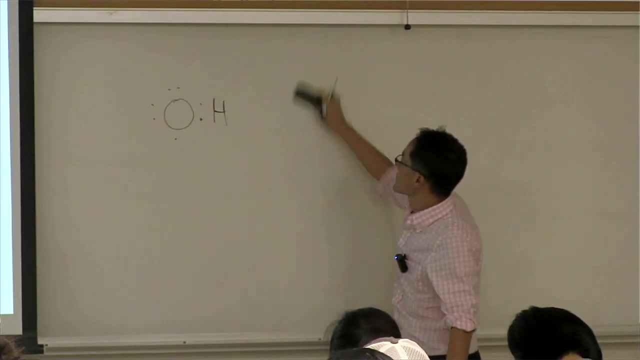 but if you are a chemically inclined person, this is the why they are very reactive, And then hydrogen has one electron here, And then let's make some bonding. Then the way we can make bonding is like this: right, 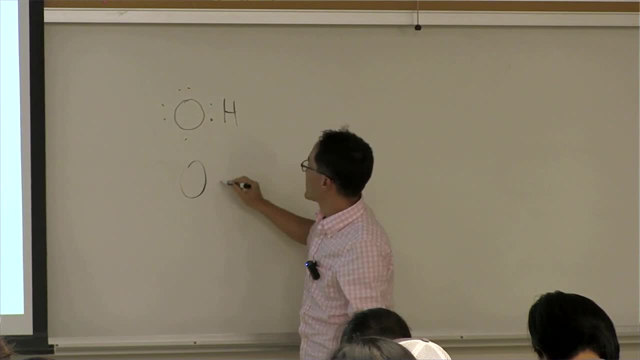 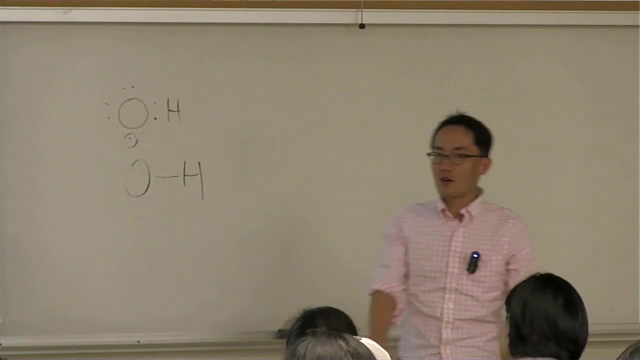 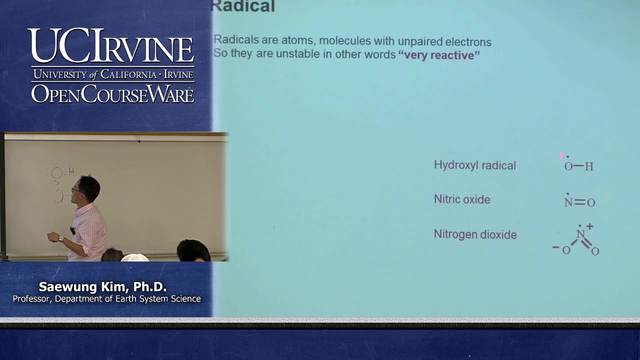 So this two electron shared by two atom is like this. But there's unpaired electron right here. This cause all the reactivity of this compound. So any gas molecule has this unpaired electron. We call it radical. Then they are very reactive, right? 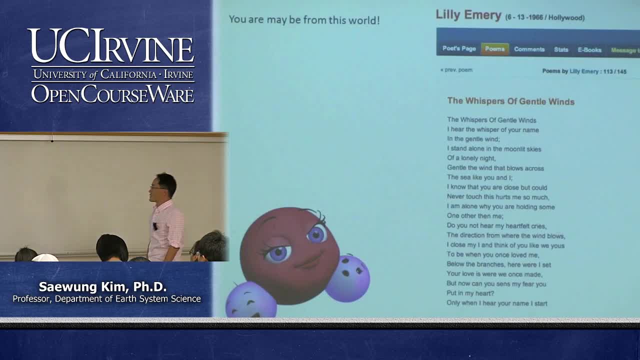 This is, this is a definition. So maybe a lot of students, you guys coming from the literature world, things like that, if your background is drama or something like that, then you may think that you know, wind is gently. 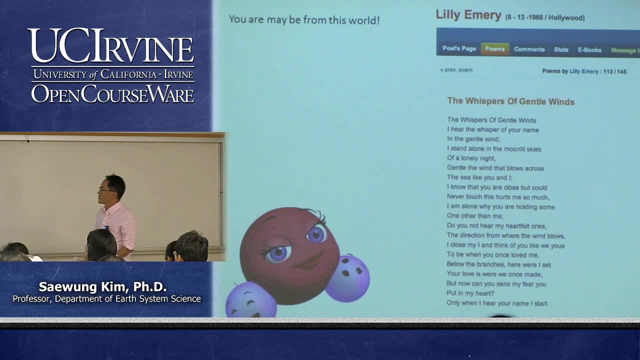 you know, kind of touching your skin, things like that. You may think that air molecule is very kind of a gentle moving kind of thing. Maybe that's your kind of world, But my kind of world is very different. So my imagination. 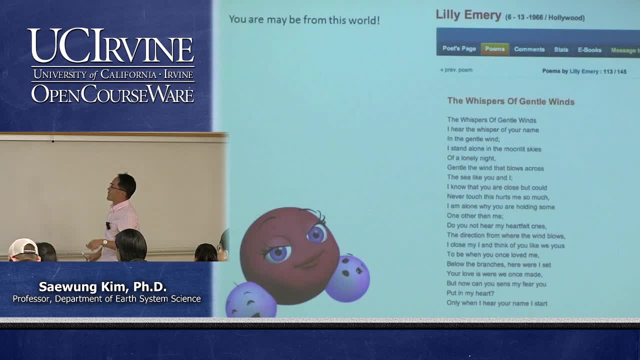 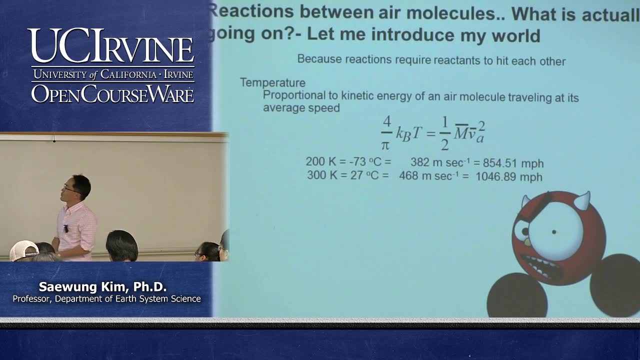 about the air molecules are very different from the this previous kind of literature or gentle wind kind of the world. So my kind of world is just like this, So you don't need to remember again this equation. But from this equation 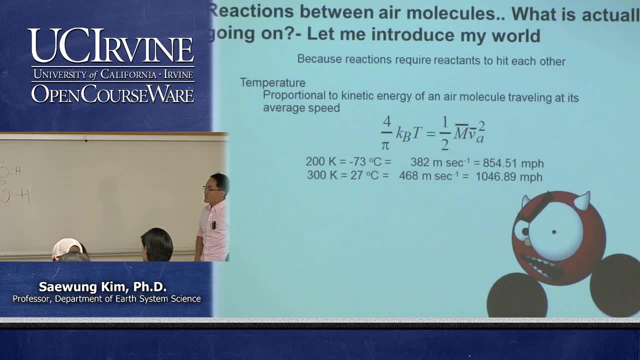 you can actually calculate the speed of the air molecule. So this, each nitrogen and oxygen are air molecule. And then air molecule is not just staying right here, Rather it's just moving along. And then the speed of the air molecule. 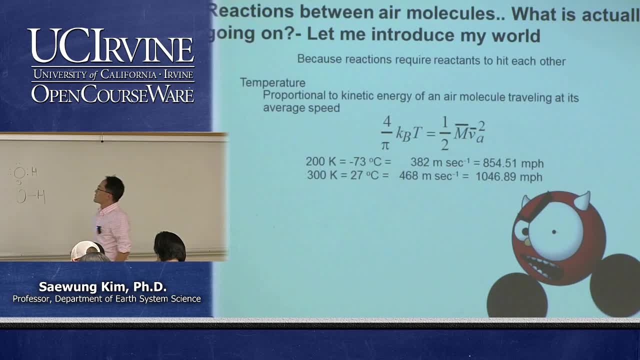 pretty much determined by the temperature. So in the room temperature, a little higher than room temperature, 27 degrees Celsius, this should be about 85,, 80 or 85 Fahrenheit. The speed is about 1,000 miles per hour. 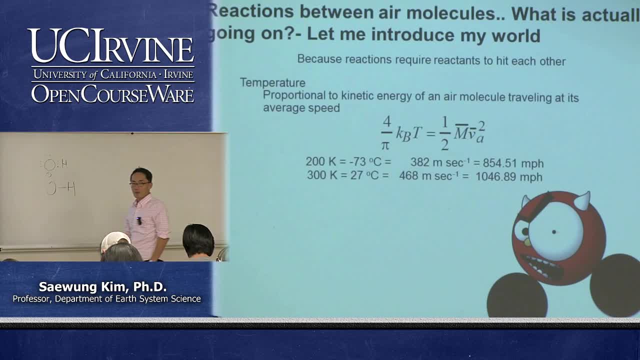 In terms of second. it travels about 500 meters Basically in the one second from here. it cannot cross the whole campus. It may get to the university town center. It's that fast, right? So this kind of angry molecule? 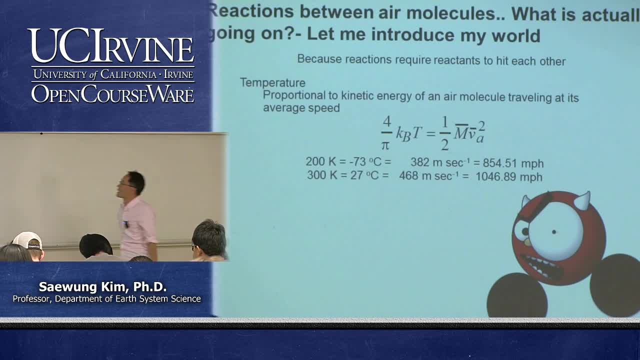 is kind of moving along in the atmosphere. That's how you can imagine about the air molecule. That can be nitrogen and oxygen, This OH, radical or NO, and then organic compound, volatile organic compound. they are all moving very, very fast fashion in the atmosphere. 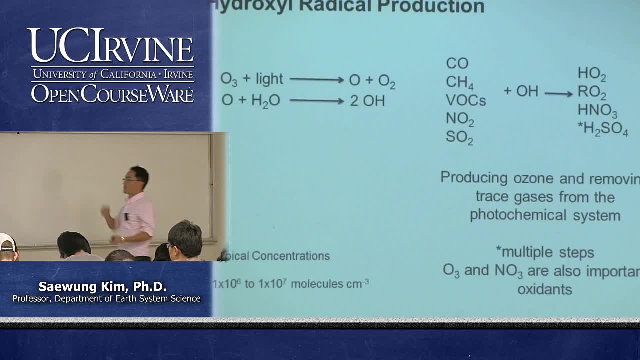 All right, Then what's going to happen? if they are just moving that fast in the air, Then they are going to hit each other eventually, right? Because there's a lot of molecule in the air. Then they are just moving very fast. 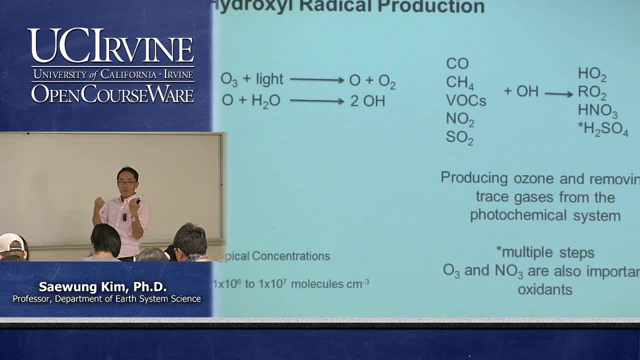 and they just hit each other, Then they will. Then that's the reaction. We will discuss about a little deeper about this reaction, But basically you can think like that way that air molecules are traveling very fast way And then there's a lot. 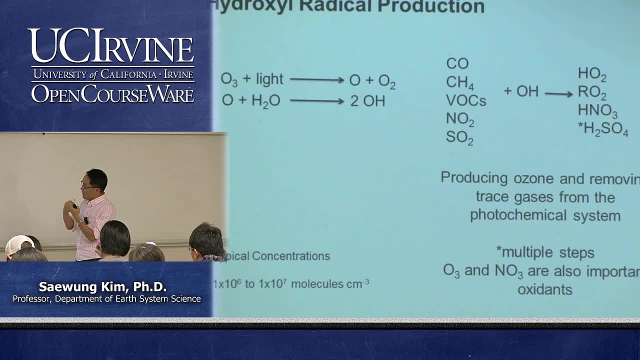 of air molecule in the air And then, once they have, Once they just hit each other, it can actually cause the reaction. So there are two. We will discuss about two kinds of reaction during this class. One is the what we call. 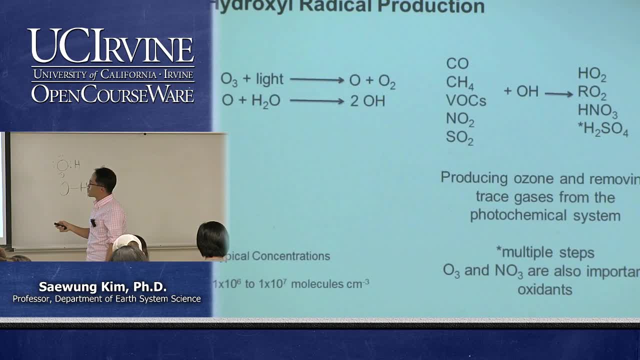 potholisis. So potholisis by definition it means that So this, For example this other ozone molecule once it gets light. So I think during the second class we talked about a wave. 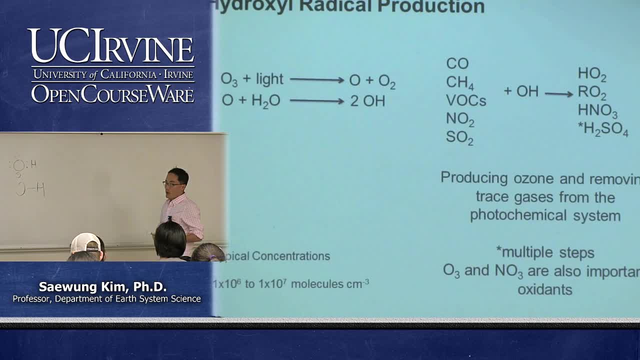 and then a particle duality of electromagnetic wave right, For example, the the energy from the sun. it has the energy from the sun, it has the energy from the sun, it has characteristics of the wave and then also that visible light. 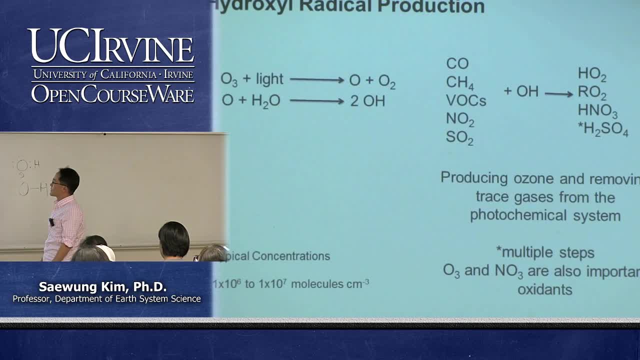 or UV also has characteristics of the particle. So let's, In this case, let's just think about the particle characteristic of solar radiation from the sun. So those energy, light particle from the sun hits the ozone molecule and then it can decompose. 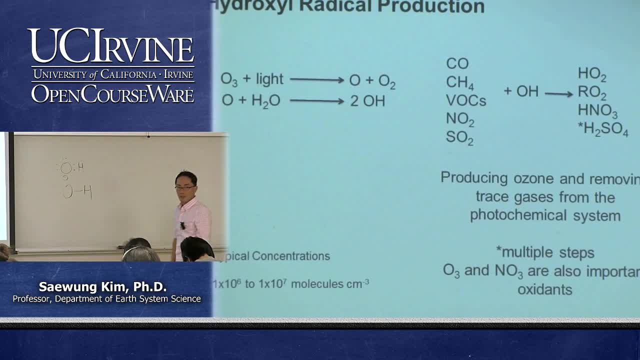 oxygen atom and then molecular oxygen, just like this. So the reaction that involves this light in the atmosphere, the light from the sun- we call it photolysis- or this oxygen atom can react with some other molecule in the atmosphere, in this case, 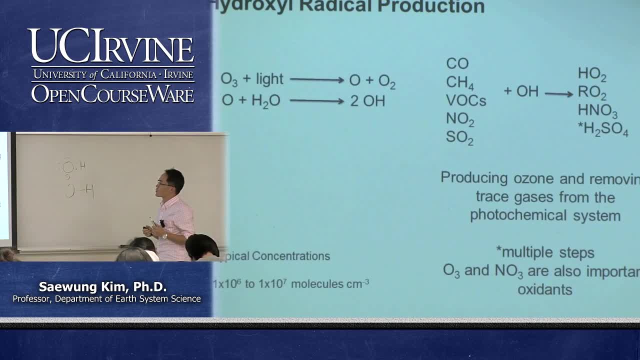 water vapor. we call it a biomolecular reaction. So this is how atmospheric OH, which is very energetic, radical in the atmosphere, generated in the atmosphere, So basically ozone get photolyzed and then this oxygen atom is reactive enough to react. 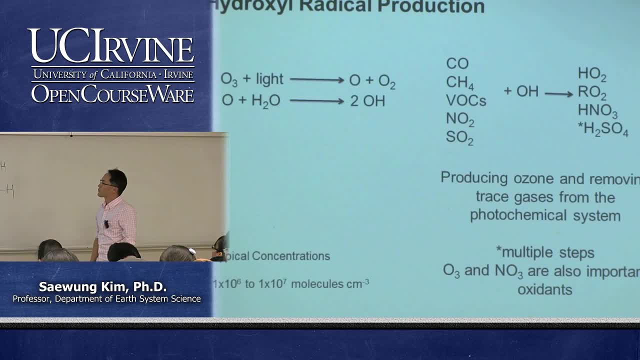 with the water to the atmosphere. pollutants in the atmosphere. So we talked about CO, which is EPA-designated criteria. air pollutants, NO2, also EPA-designated air pollutants, SO2, also EPA-designated air pollutants. So, and then VOCs. 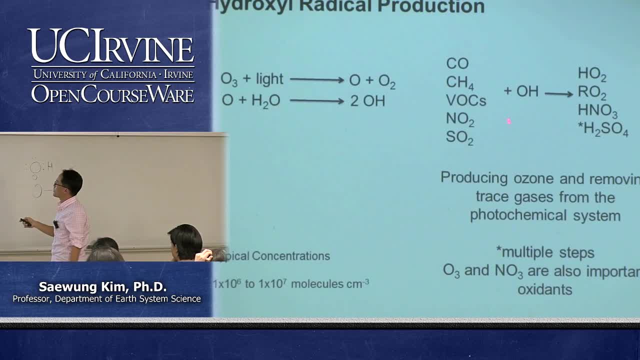 this is volatile organic compound, organic gases in the atmosphere and then removed from the atmosphere, So basically OH, because it is very, very reactive, that concentrations are very small. So it is the notation of this concentration might be a little. 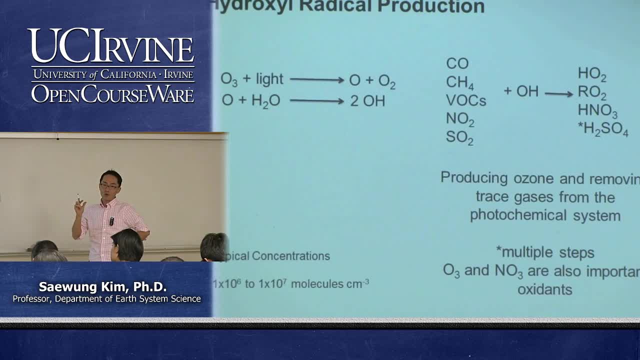 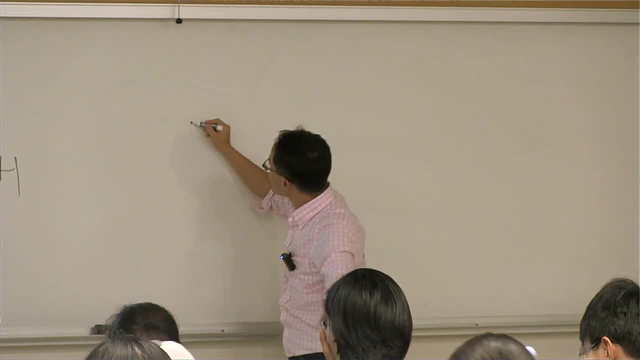 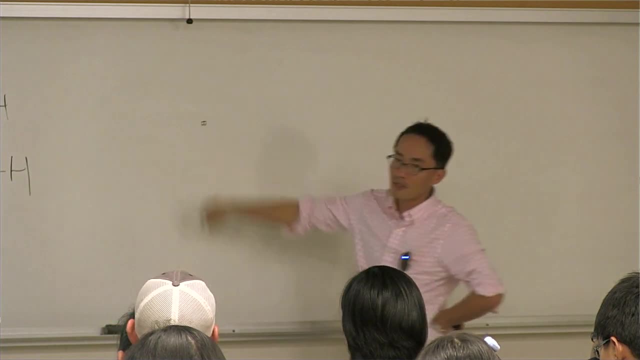 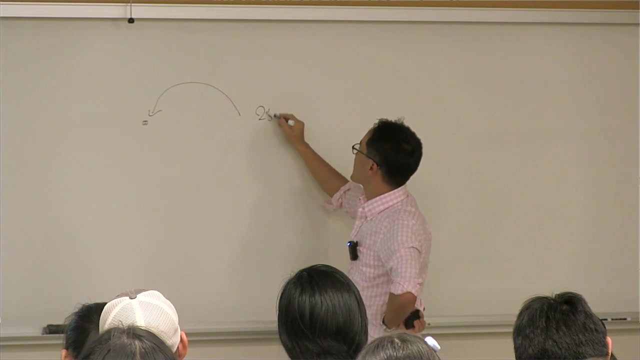 confusing, maybe a lot confusing, to you. So this is about this low. So one cubic centimeter is like this, right? So I'm not really artistic guy. So this is basically one cubic centimeter, right? So 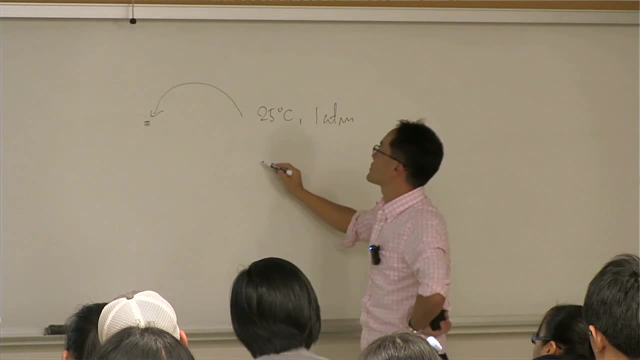 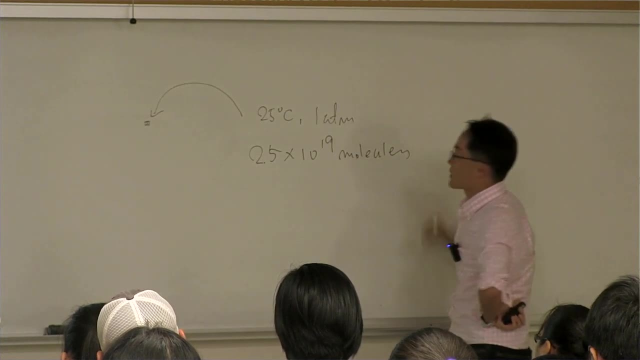 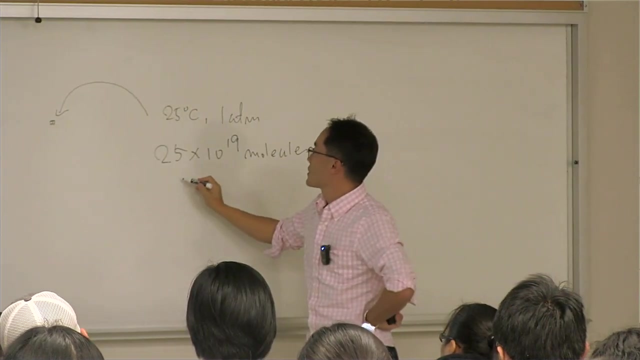 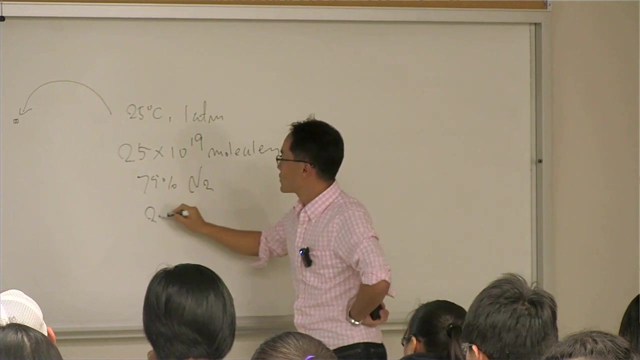 number of gas molecules in 25 degrees Celsius, and then molecules per cubic centimeter. And then what's the composition of the? So, out of this, about 79% is what? Nitrogen, right, And then 20% oxygen and 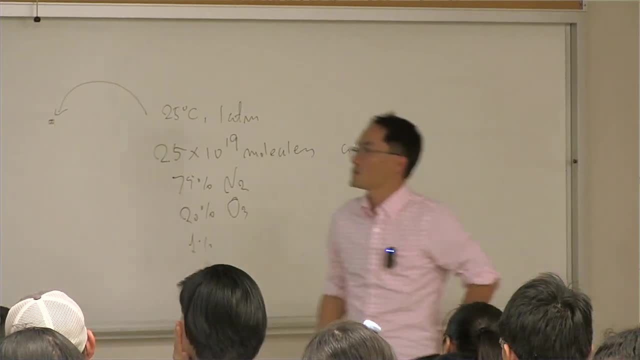 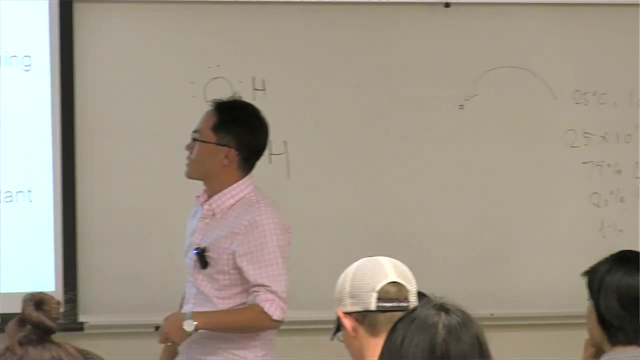 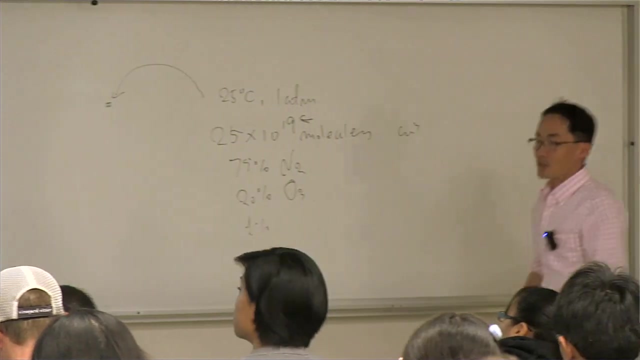 then about 1% are some other species. So probably it is somewhere between 10 to 6 to 10 to 7 molecules per cubic centimeter. So out of this, so in terms of fraction, then 2.5. 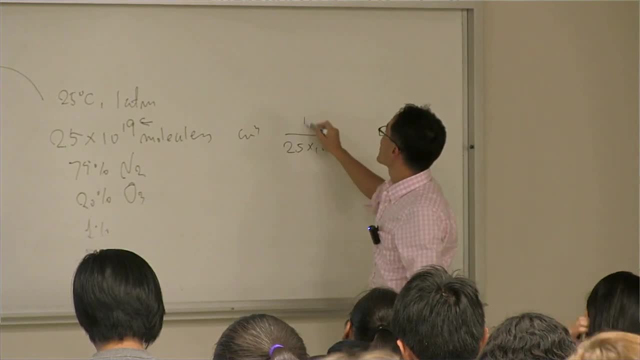 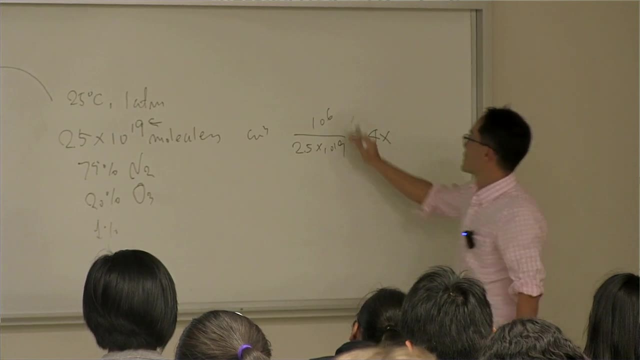 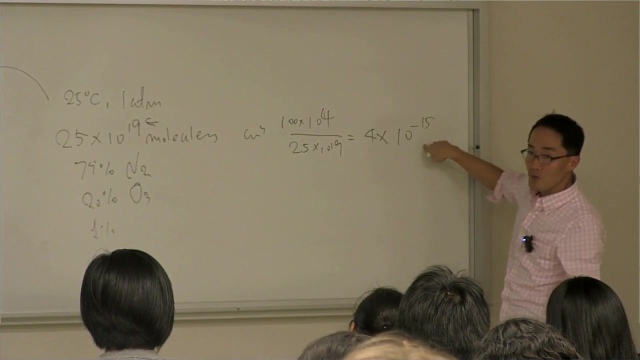 times 10 to 19, and then 10 to 6.. So this is about 4 times. so give and take 100, 4, 10 to 15 in terms of mixing ratio. So this is really tiny, tiny, tiny fraction. 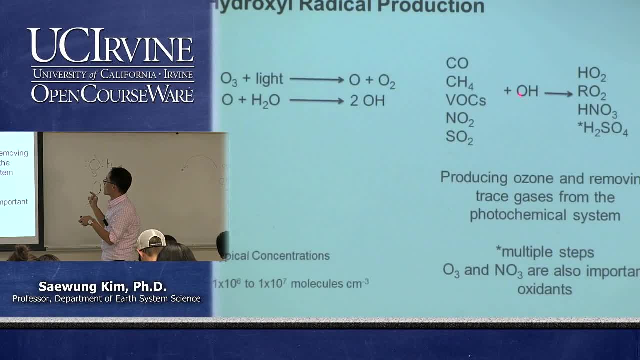 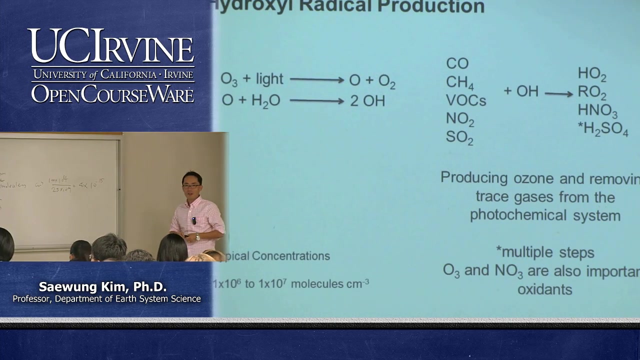 but still, this small fraction of the radical in the atmosphere removes chemically, removes most of the pollutants in the atmosphere. So we call this OH radical as atmospheric puriclinger. Anybody has any question about OH? Okay, so you can. 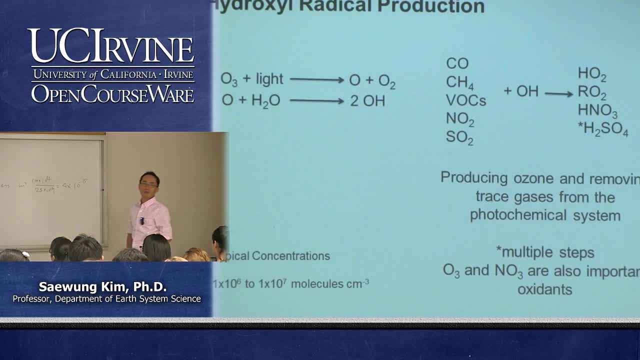 go over again. You want me to go over? Yeah, go, I was going to clarify. so the OH is good in this. Yeah, Okay, So you want to maintain small concentration in the atmosphere. So that's all you need to. 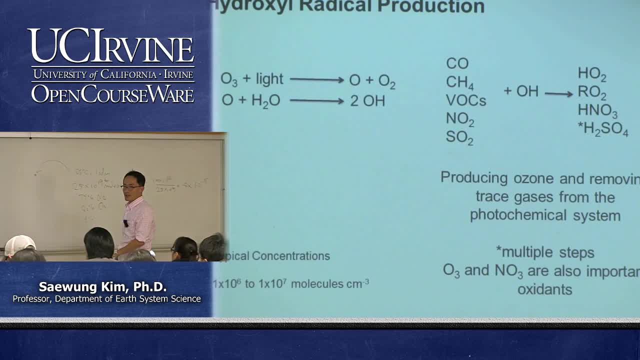 know, But if you want to know a little more, you can study about this, chemistry and things like that. So I think last time I warned you that today is going to be the most difficult class ever. So, okay, Any question. 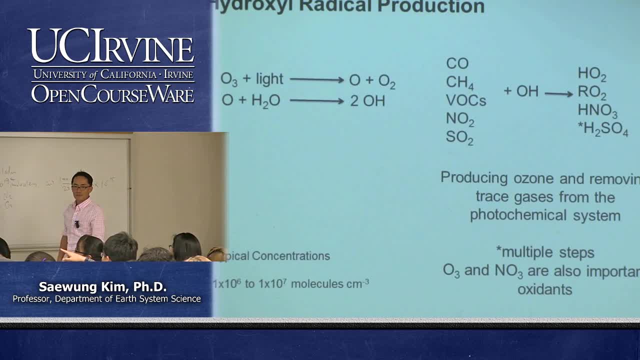 Any more questions about this so far? Isn't the product made by? Yeah, It's a very sulfuric acid. Yeah, It's also harmful. They are harmful, but for the water quality, in terms of the air quality, that's a. 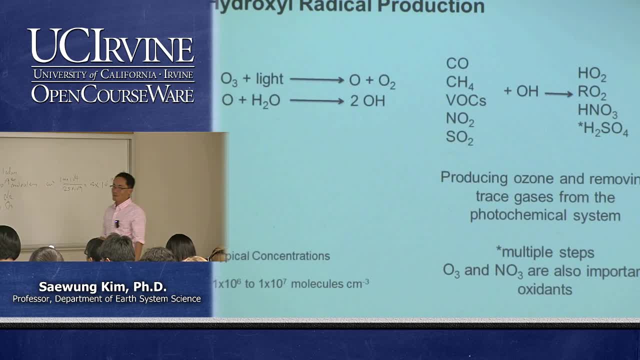 good thing, But we are going to talk about air pollution. So for the air pollution perspective, that's a great thing, but we'll talk about some bad thing that this sulfuric acid has been doing the past 50 or 60 years. 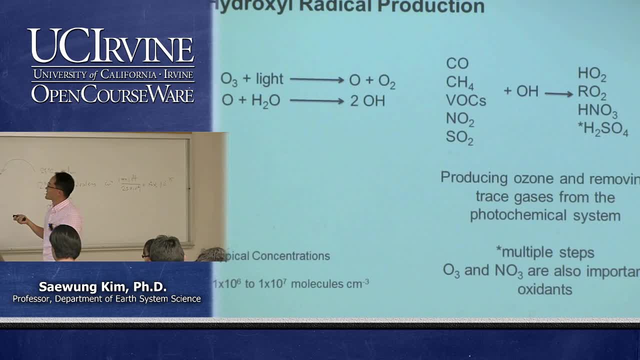 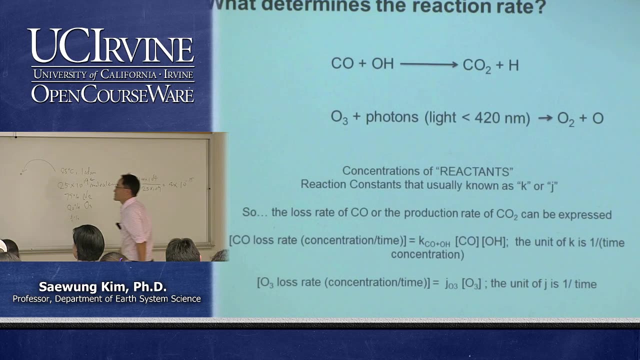 when you talk about sulfuric acid. So what we need to know at this time is that OH radical has a very small concentration in the atmosphere, and then it can remove all the air pollutants from the atmosphere. Let's go So this. 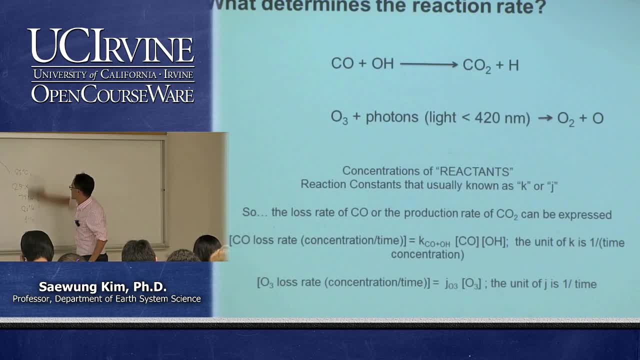 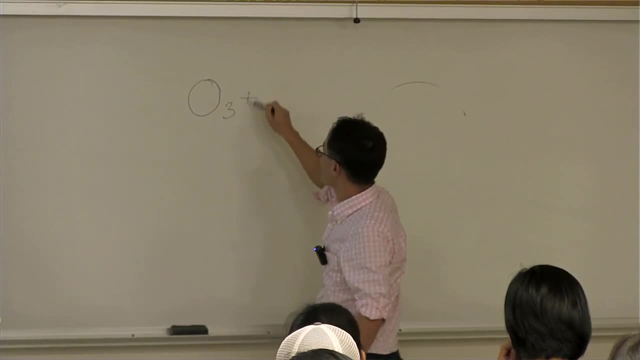 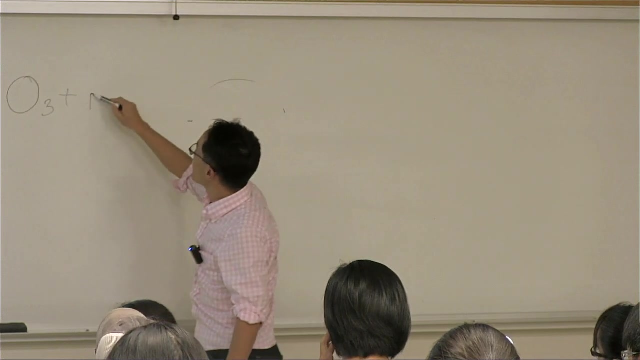 is kind of an introduction to the reaction in the atmosphere that at least we are going to. that's something that we are going to discuss during this class. One is whatever molecule it is, for example ozone, and then, once the sunlight's coming along, 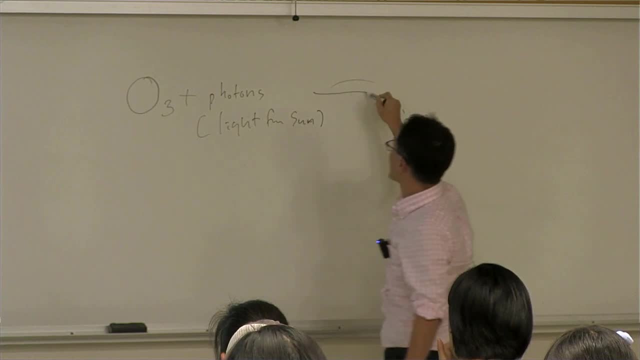 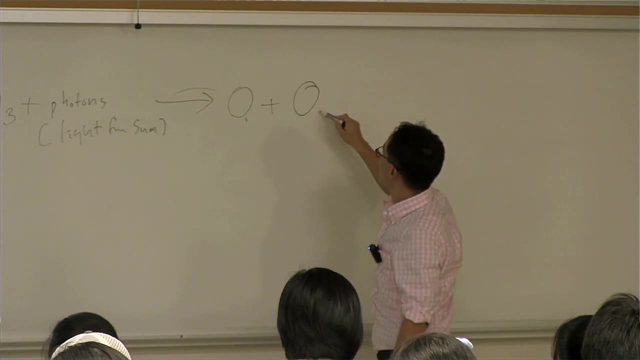 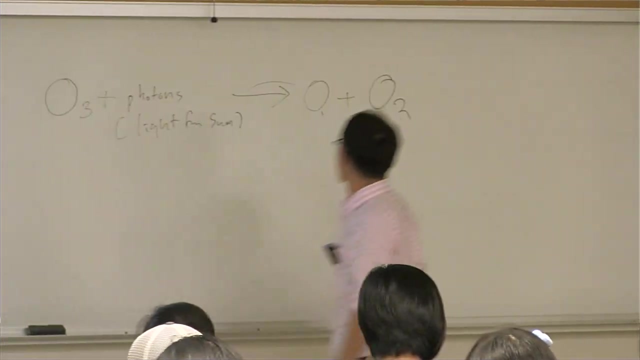 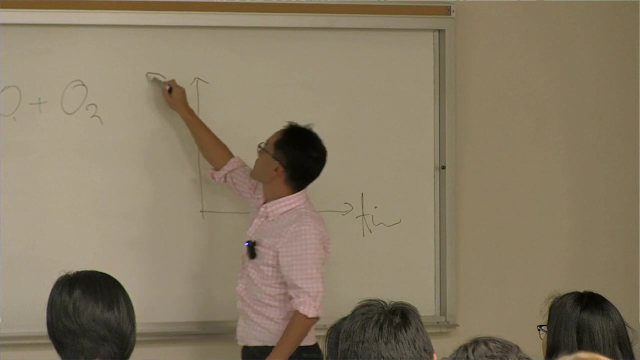 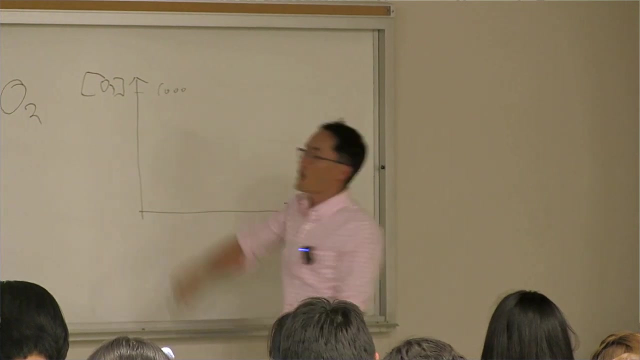 and the sunlight is strong enough, and then this guy's going to decompose as atomic oxygen the molecule oxygen, something like that. Then let's think about- we talked about time- and then concentration of ozone. right, Let's say there's. 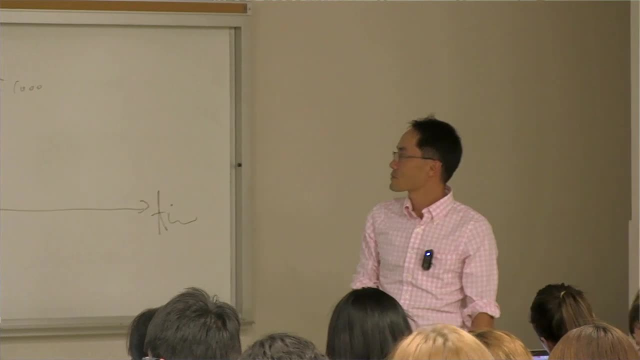 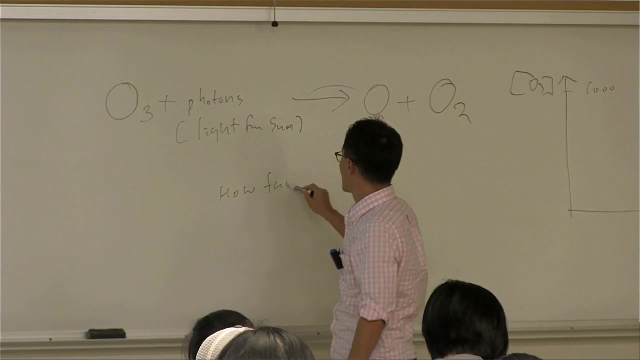 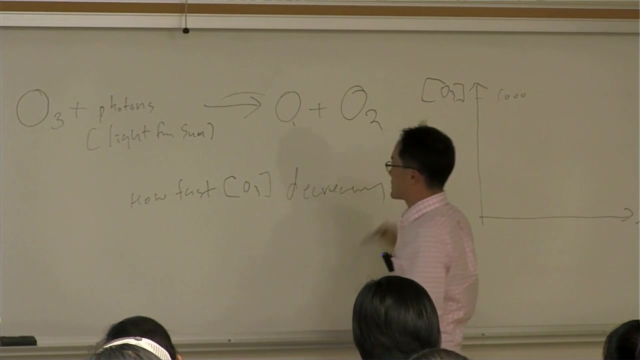 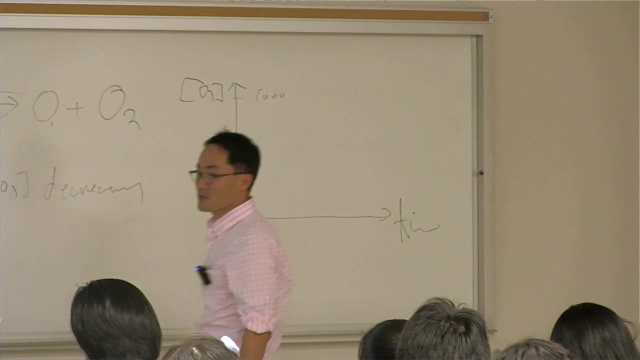 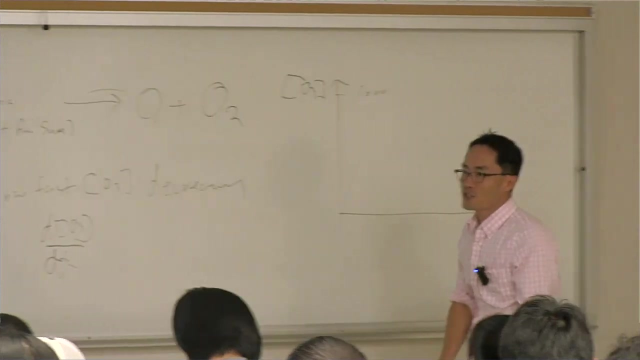 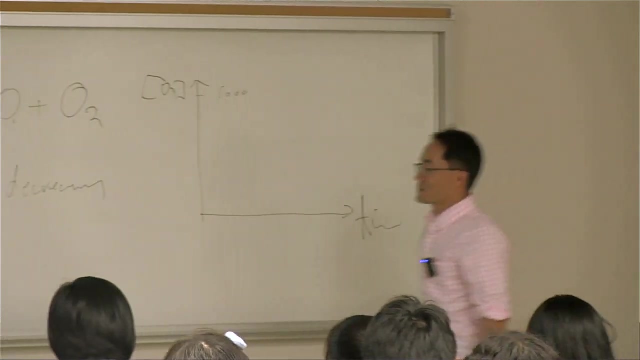 a molecule here, right. Then we want to know about how fast ozone concentration decreases. And then we scientists hate to write sentences on the board, so what we usually do- this is, by definition: ozone concentration change over time. okay Then. 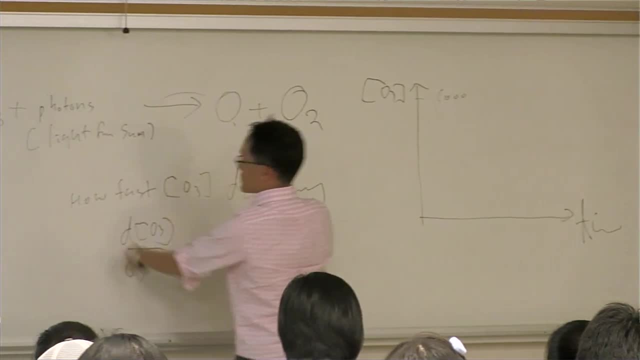 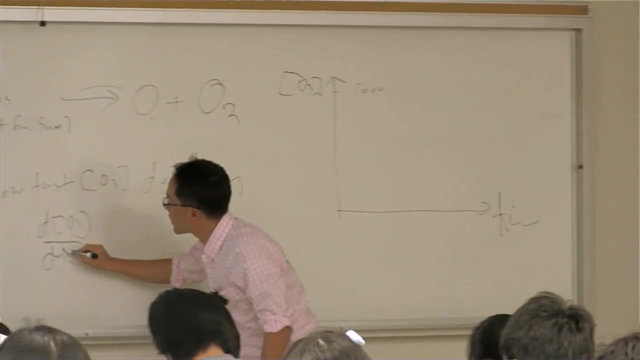 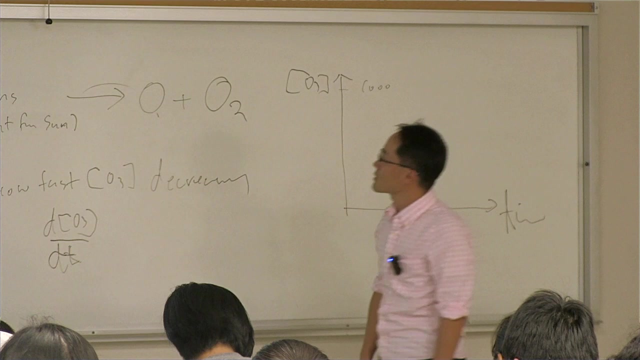 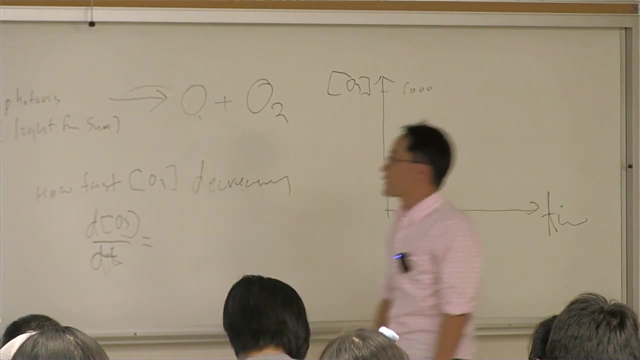 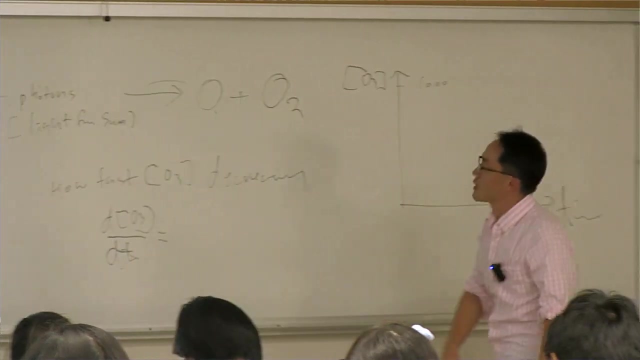 we can just make this long sentence this simple notation, all right. So basically, this is notation of how fast ozone removed from the atmosphere by this molecule, right? And then there are two factors determining this removing speed of the ozone in the 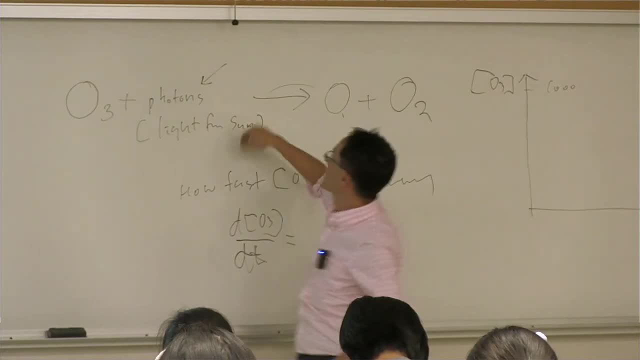 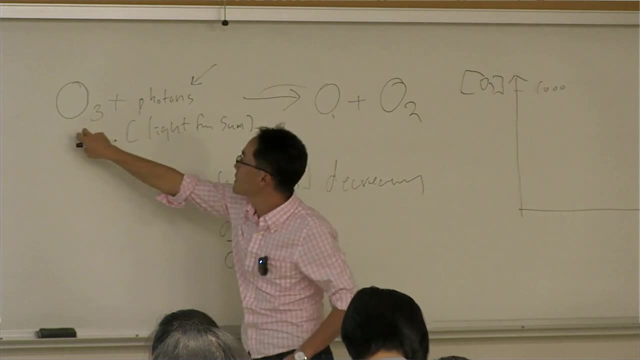 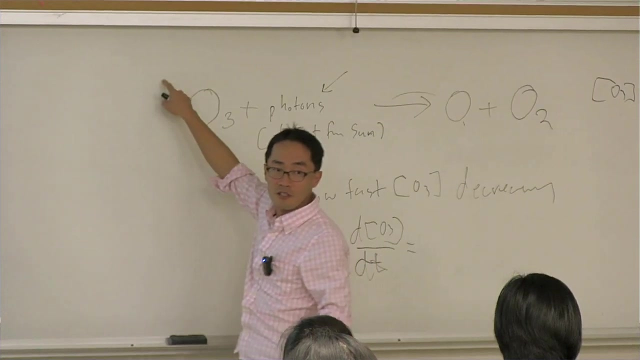 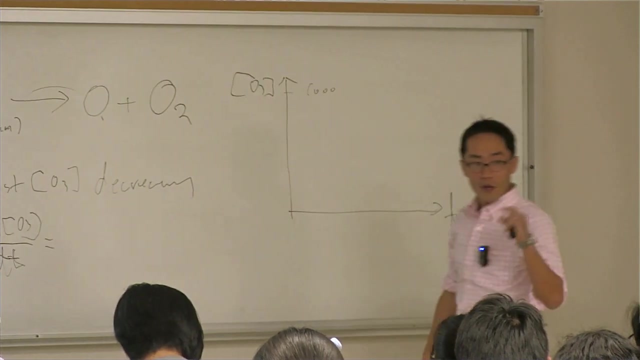 atmosphere. right One is this: photons. if there's more photons in the atmosphere, then the removing speed of the ozone concentration itself right. If ozone concentration is high, then removing rate is going to be faster than when ozone concentration is lower. 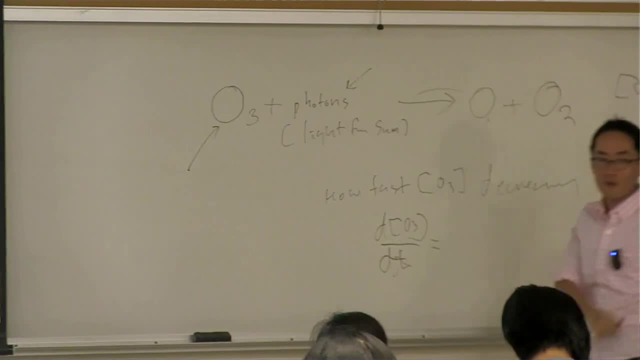 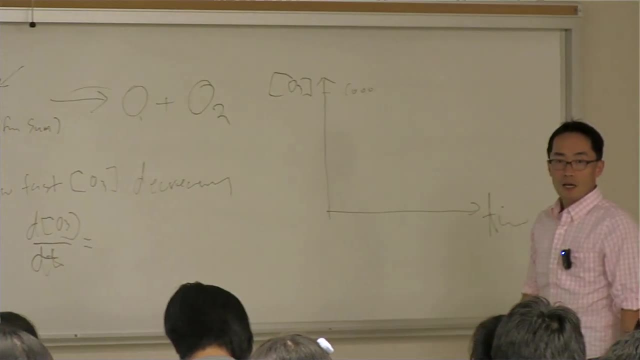 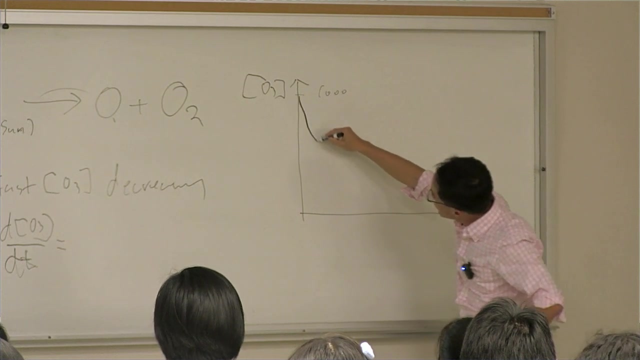 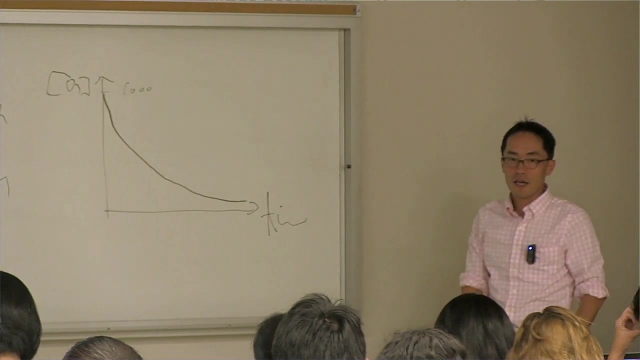 right. Does that make sense? So there are two independent things: ozone concentration and number of photons. So basically you can. basically it's going to be removing from the atmosphere as time going by if there's light in the atmosphere. 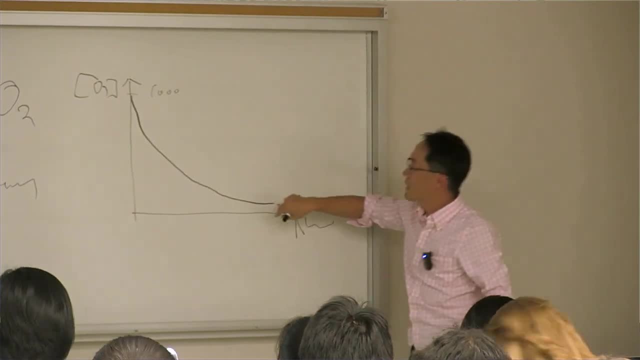 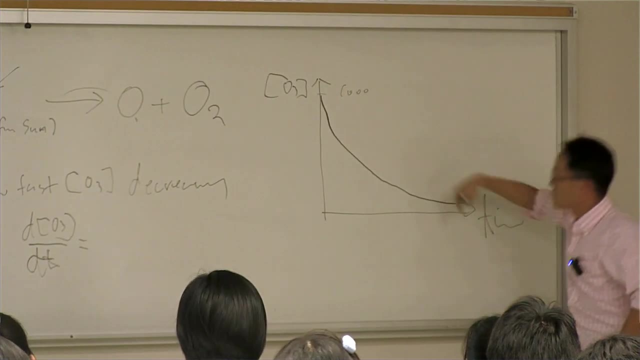 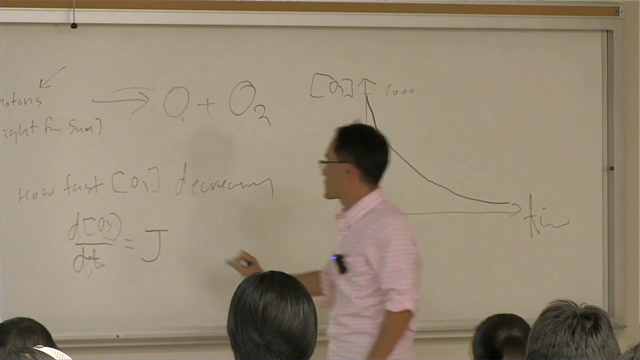 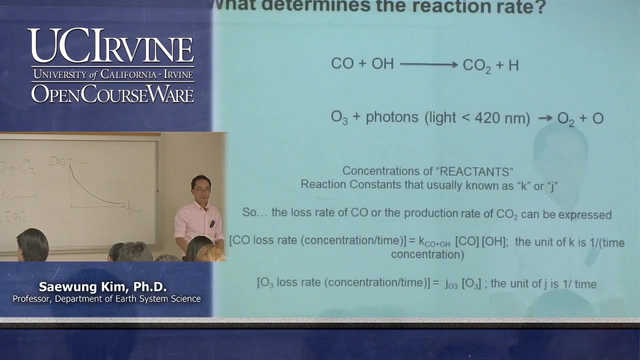 right, So it's going to go away. and then we mathematically express this decay of ozone concentration as J, we call it ozone and then ozone concentration. Okay, this is again definition. So this is photolysis. 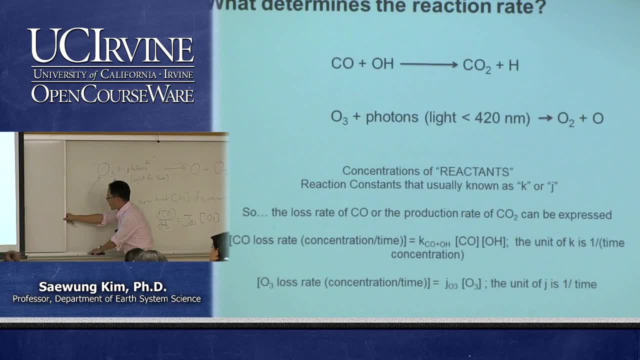 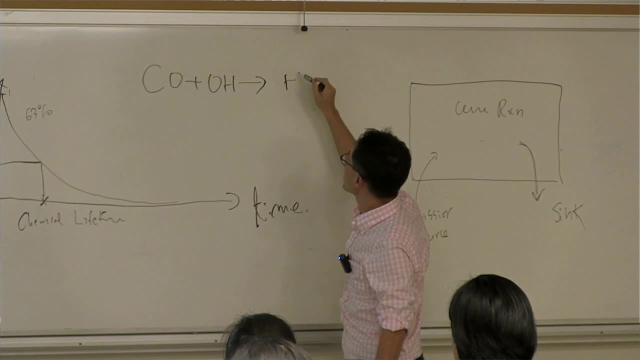 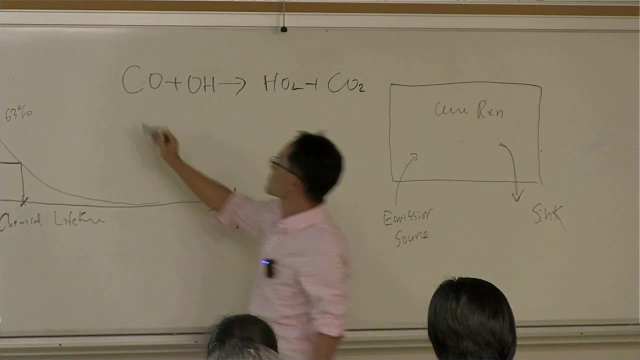 reaction in the atmosphere. Then another thing- this is definition again. For example, CO plus H, then HO, HO2? No, Yeah, HO2 plus CO2.. So let's talk. let's talk about the CO perspective. 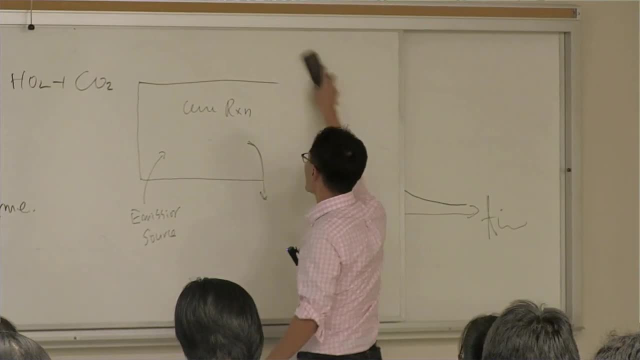 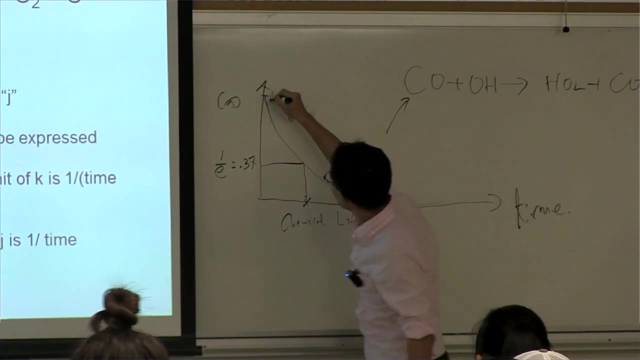 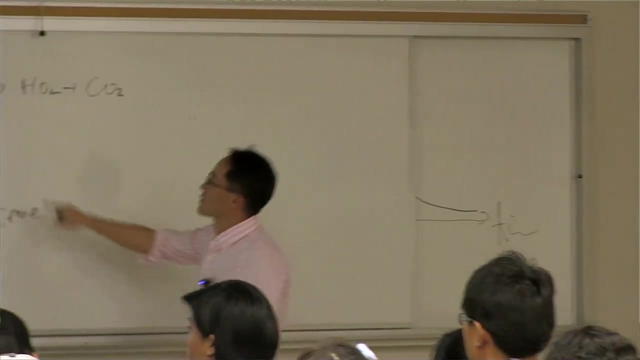 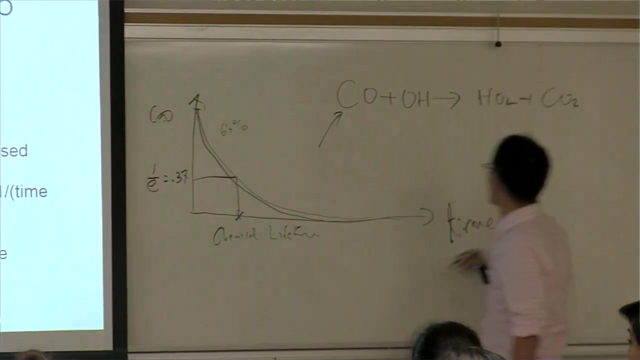 So in terms of the reaction dynamics also, let's assume this is CO. So this CO from the atmosphere, from this reaction. there's two things it's gonna determine the CO removal rate. One is again in given time. 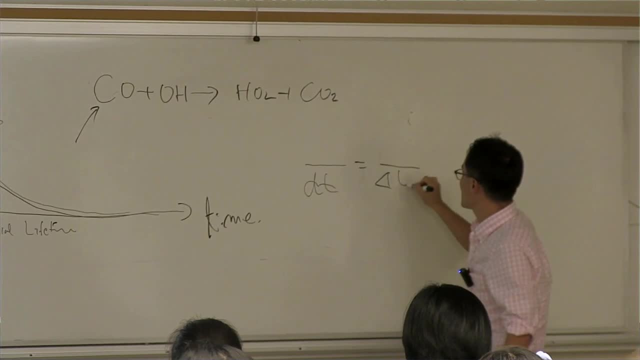 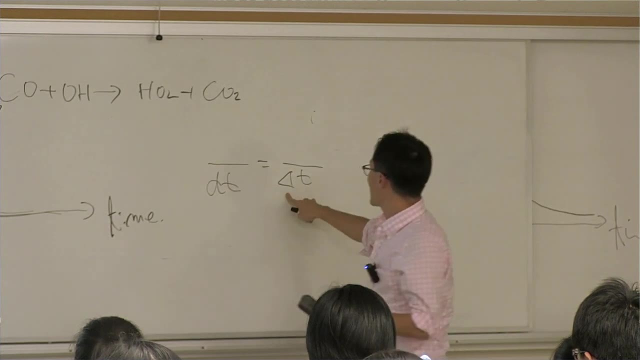 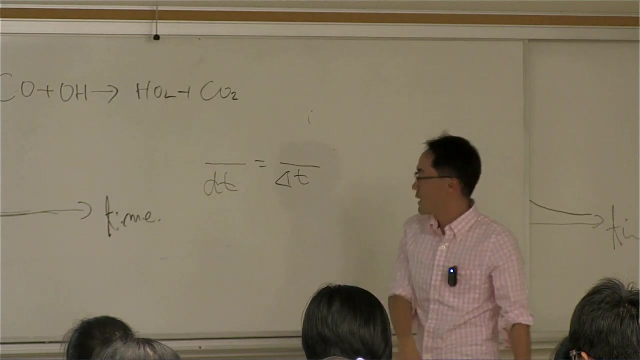 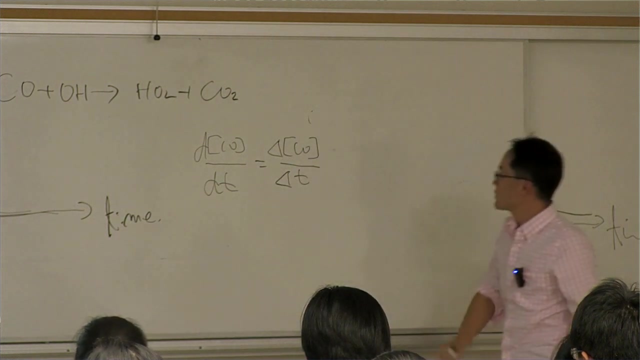 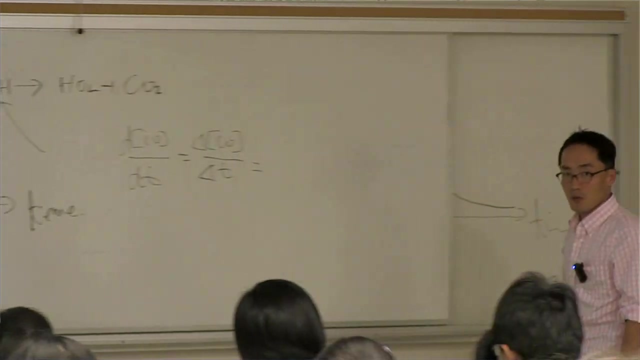 maybe if you haven't heard, haven't seen this notation, you may see this delta rotation. So delta is much more larger than the CO concentration. So this CO is kind of same thing. You can just use the delta also Again. 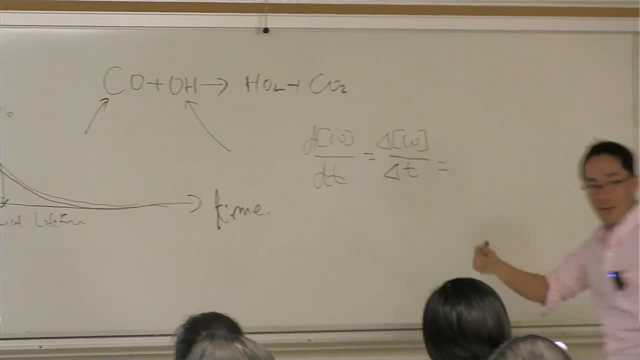 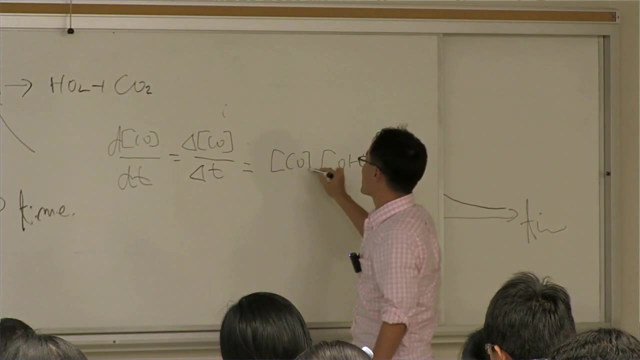 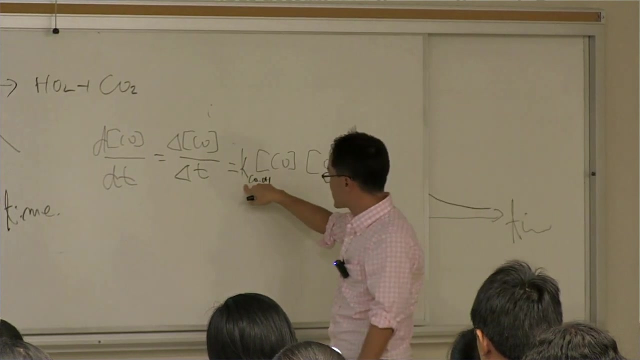 it's gonna depends on OH concentration, right? When OH concentration high, then just like the ozone, and then we call it reaction constant. So it depends on how reactive they are. So this reaction constant is determined. So 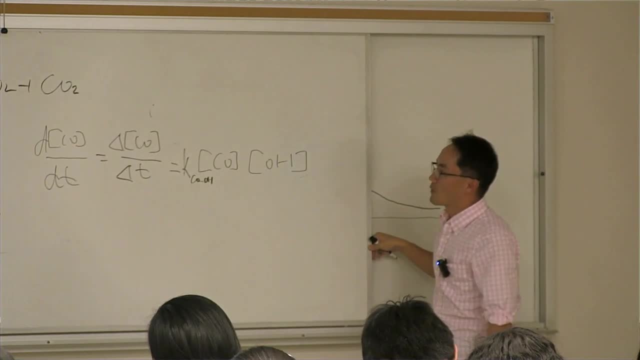 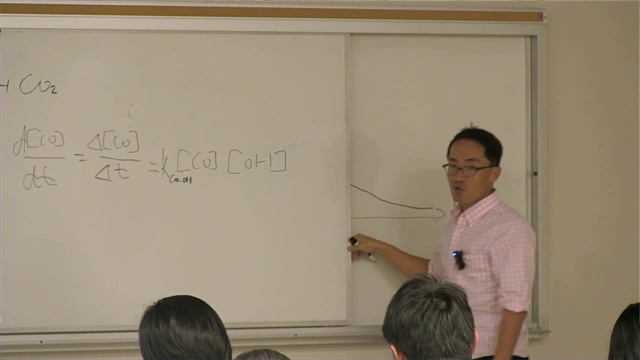 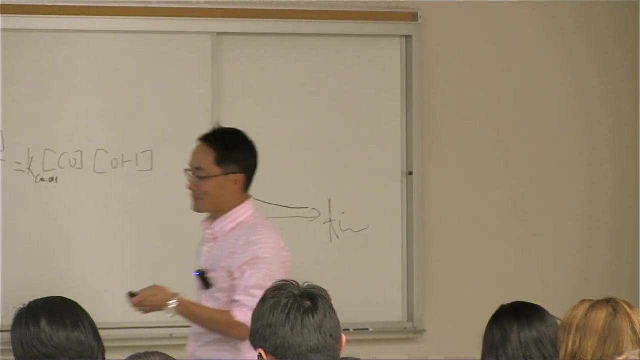 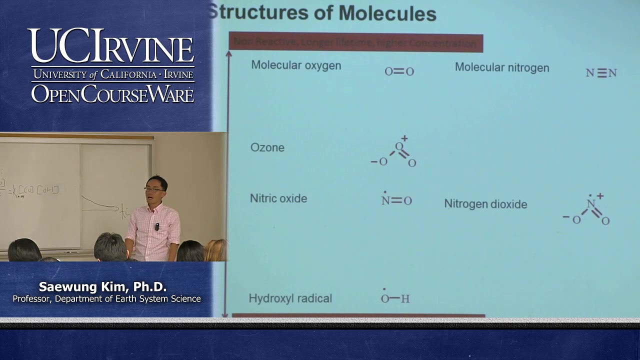 we're gonna talk about this thing a little later. So this is the definition and the mathematical formulation of how the molecular reaction and the patholysis, right, Okay? So again, this is kind of a summarize of the lifetime chemical reactivity. 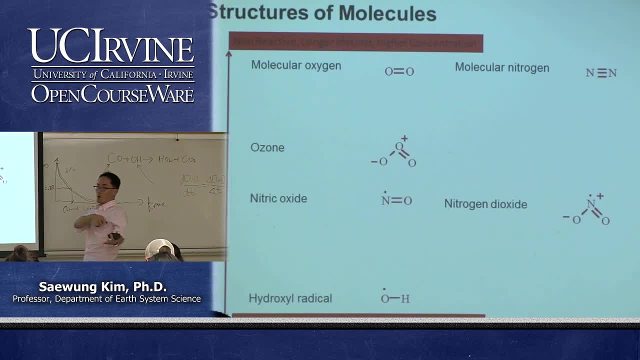 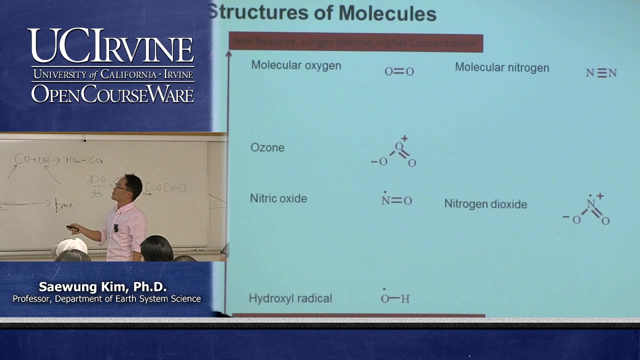 and then concentration. right How they are related. So molecular oxygen, which is 21% of the very high concentration, And then they are not reactive. That's probably why they have a high concentration and a long lifetime. So 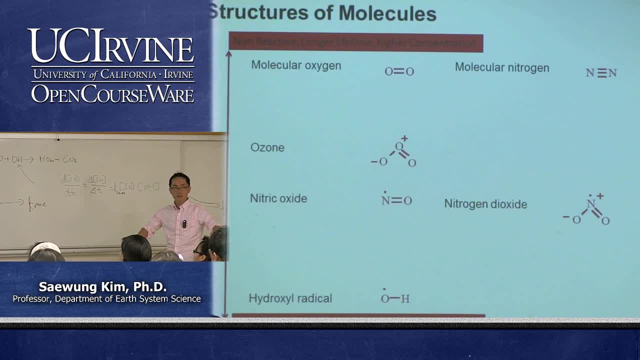 once it gets more reactive their concentration gets smaller and then lifetime getting shorter. So they are all the same right. So it's far less reactive in the atmosphere. So ozone concentration in the atmosphere is far much smaller than the molecular oxygen. 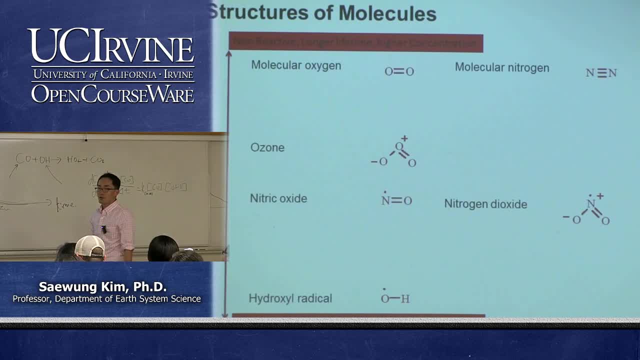 and nitrogen, And then we'll talk about NO and NO2 today, And then we already discussed a little bit about the OH And then infraction. we basically just look through about the OH concentration, which is about 10 to 6 molecules. 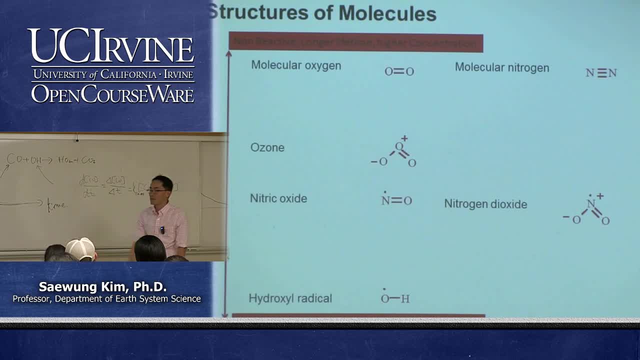 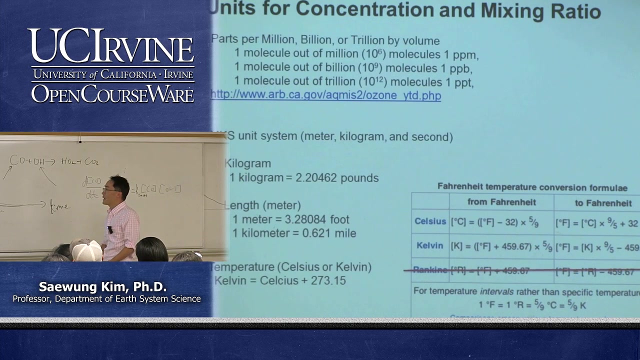 per cubic centimeter. So this basically, in the list of this molecule, OH has shortest lifetime and then most reactive and then lowest concentration. So we talked about concentration as PPM, PPB and PPT, And then actually, 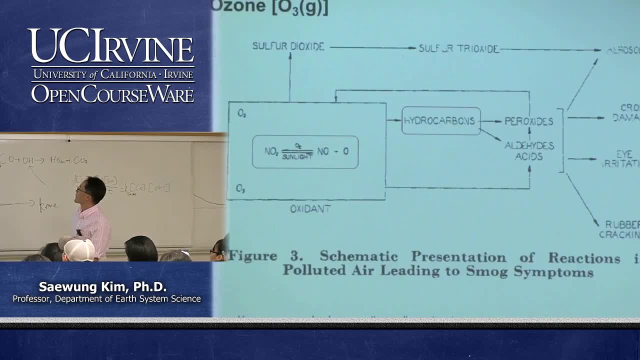 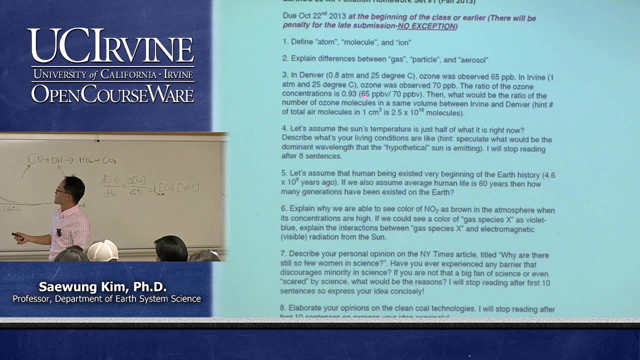 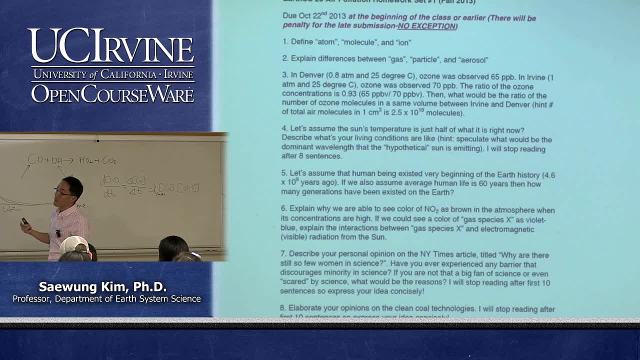 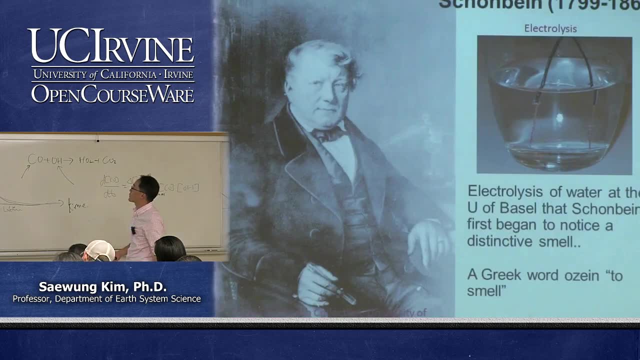 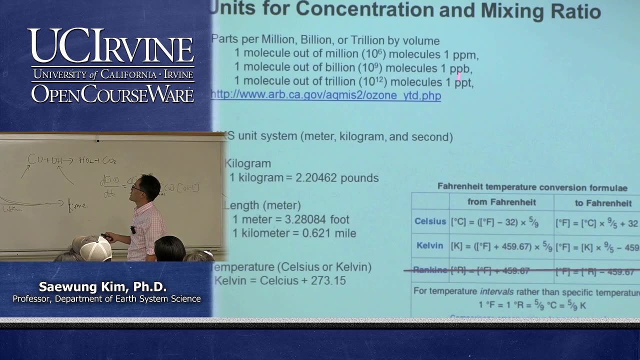 So parts per billion by volume. So PPB is basically same thing, Right? So let's go. So the question is asked about convert this PPB, PPM and PPT to number of molecules in given volume. 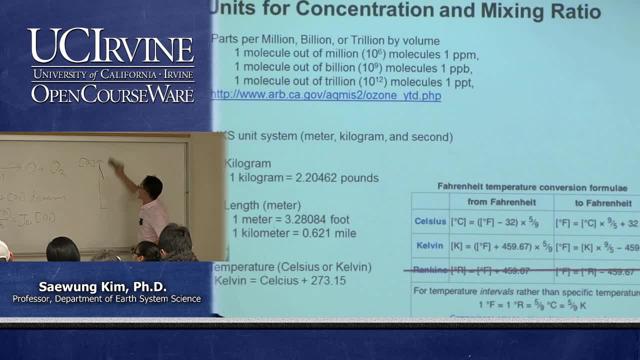 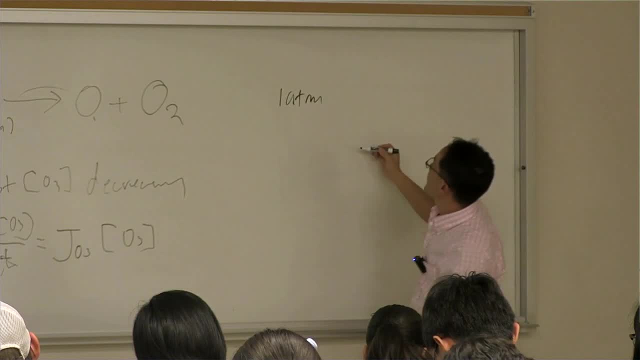 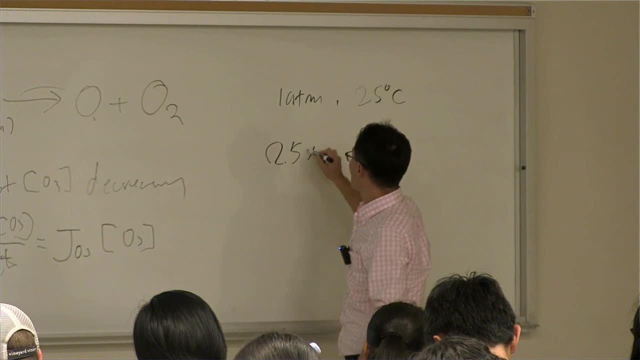 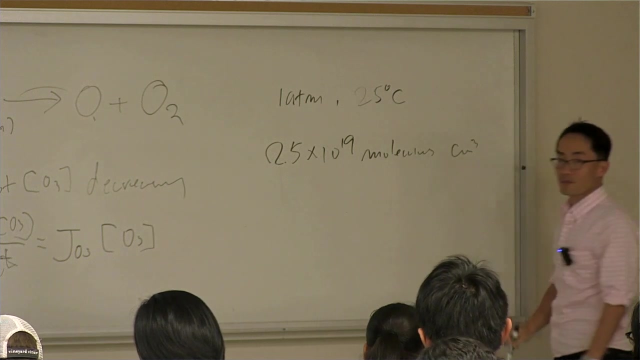 And where is it Probably? I explained that In one atmospheric pressure and then 25 degrees Celsius there's about 2.5 times 10 to 19 molecules in one cubic centimeter Right And then about 80 percent. 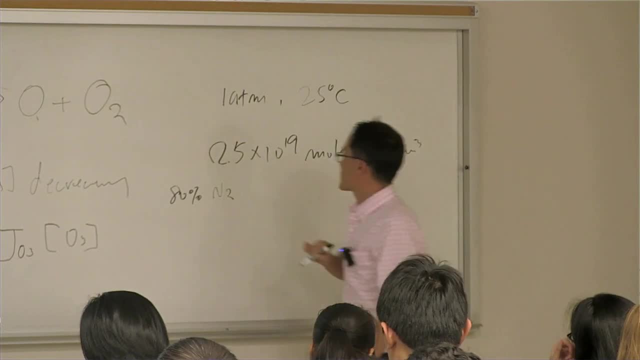 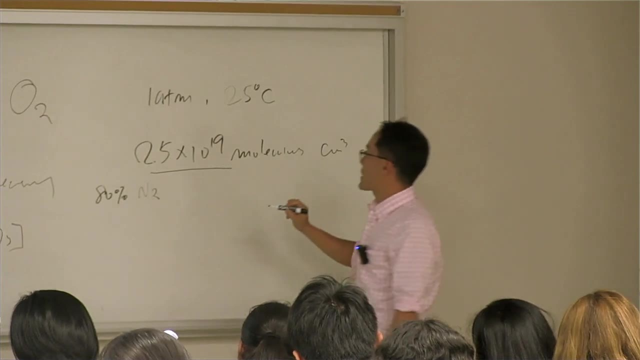 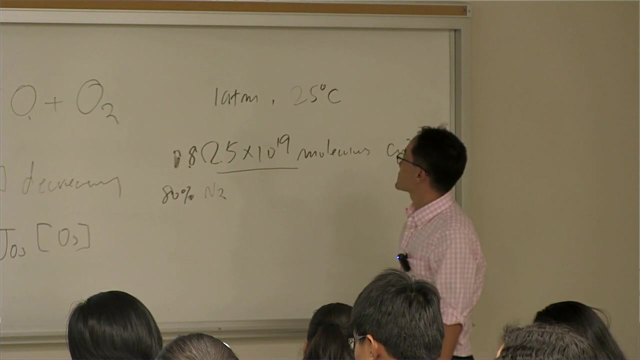 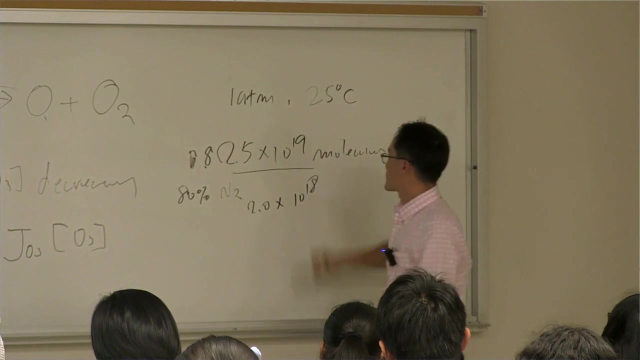 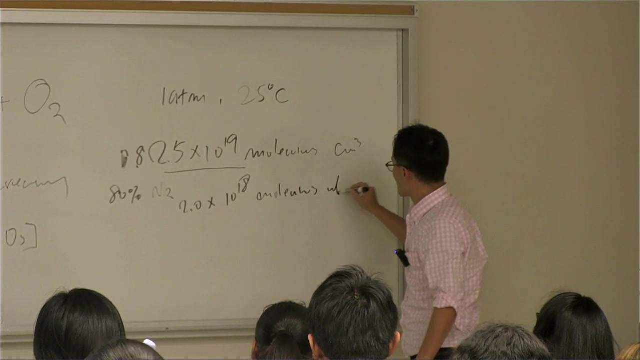 let's just say 80 percent. right Then, out of this, how many nitrogen? So this is about? so basically, 0.8, right, 0.8 is 10.. Should be nitrogen right In one. 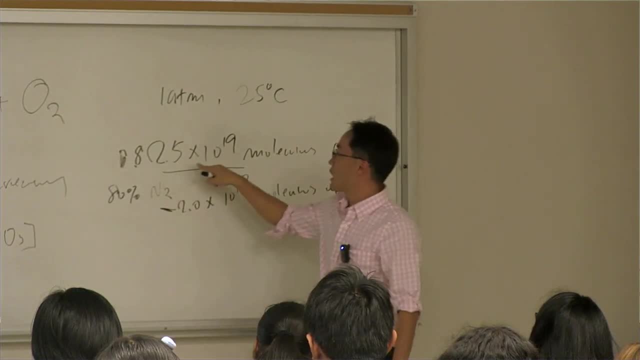 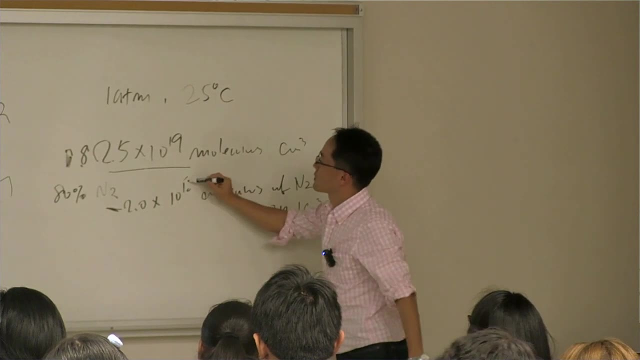 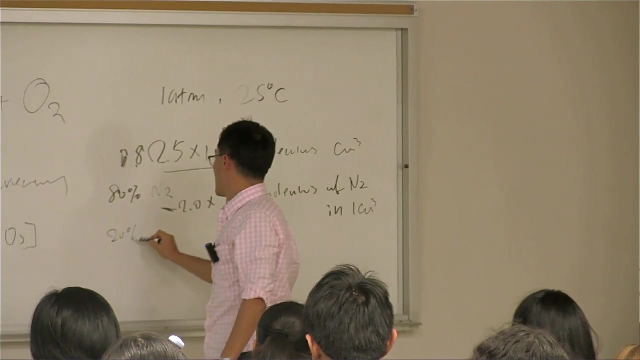 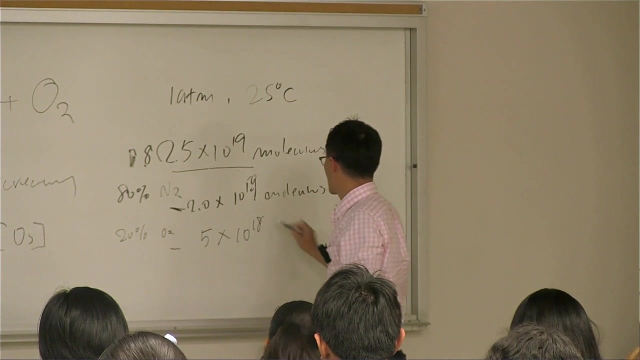 cubic centimeter, Because it's nitrogen. So out of this number of molecules, 80 percent is nitrogen. So that should be like this, right? No, this should be 19,. right, Okay, And then let's. 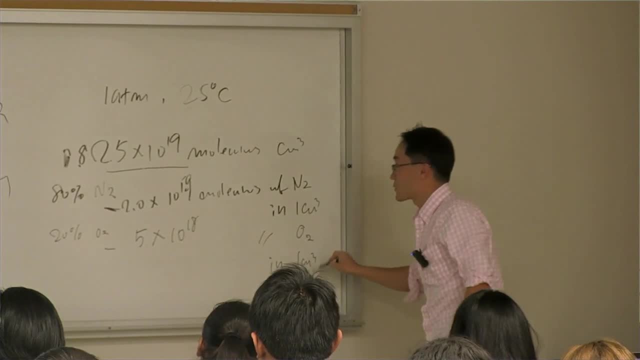 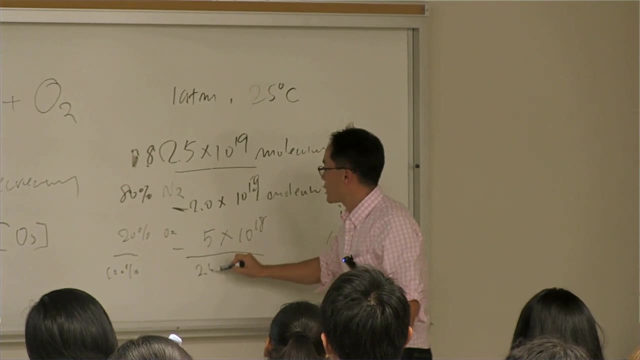 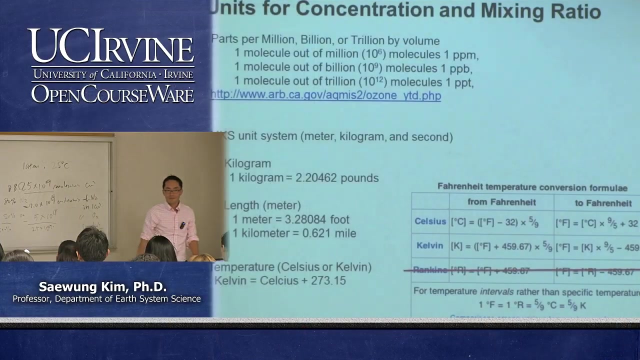 look at oxygen in one cubic centimeter, right, Basically, if you add these things up 100 percent, and then this is 2.5 times 10 to 19, right? So basically this whole thing Okay. 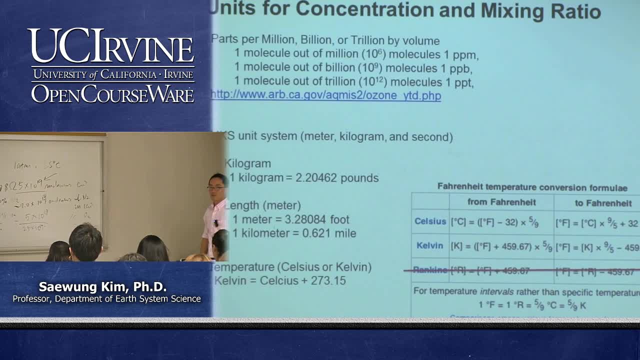 This is how you convert number of molecules from percentage of the number of molecules. Too many numbers? You don't get it. Eh, Eh, Okay, Let's. So maybe you're just overwhelmed by this 19 thing, right, It's? 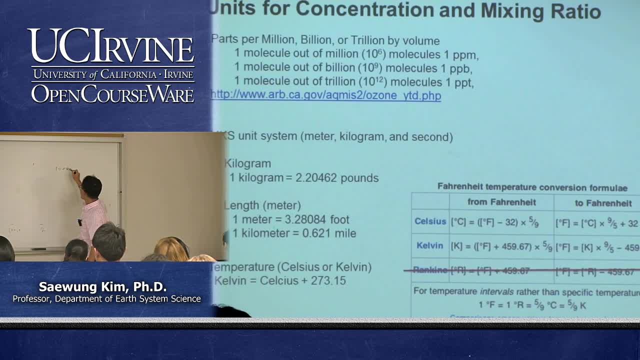 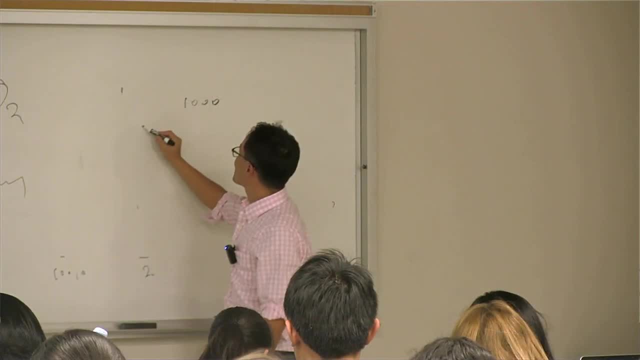 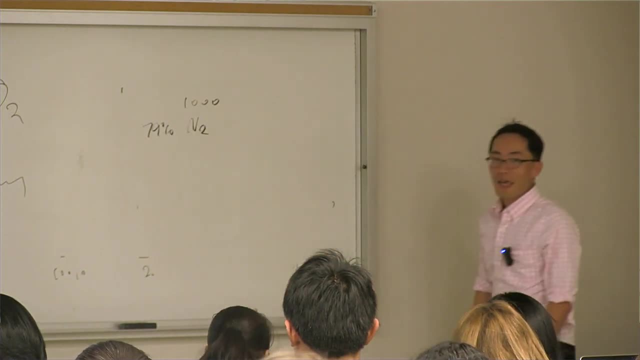 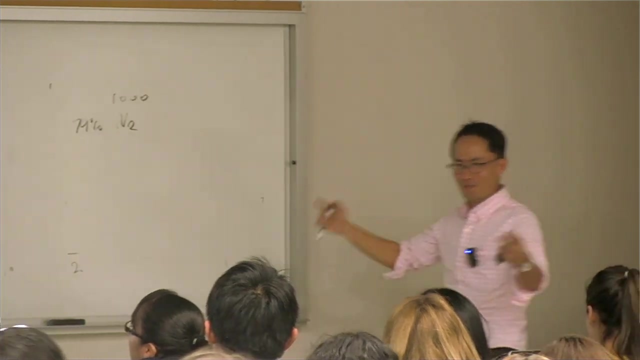 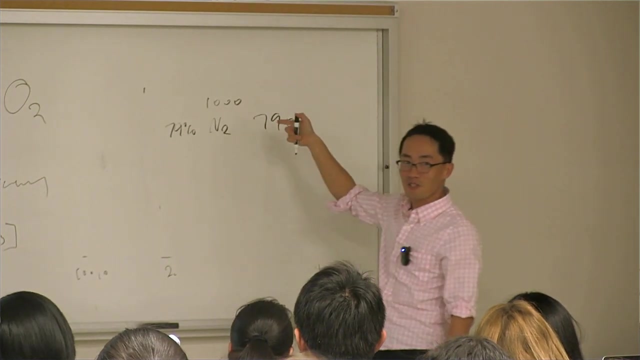 too many? Okay, Then let's go much, much further. Then let's say 79 percent are nitrogen, Then how many molecules in this number of molecules of air are nitrogen? How many? 790, right, Okay. 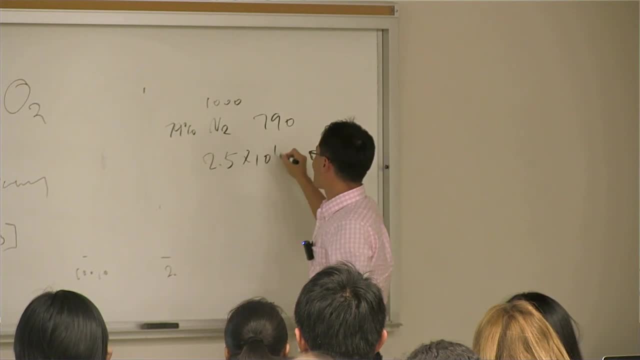 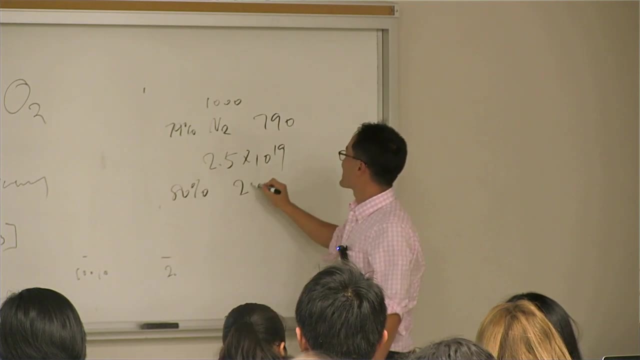 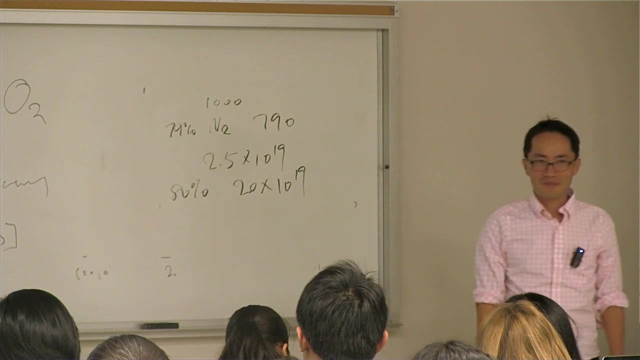 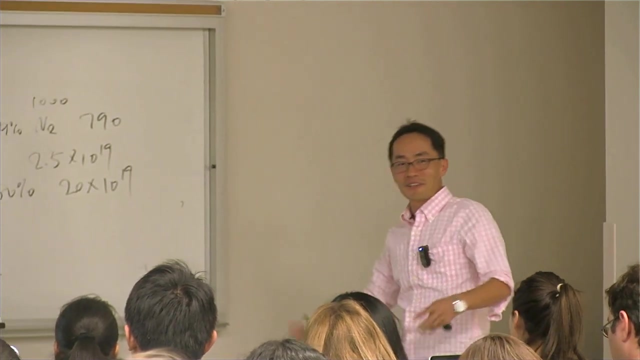 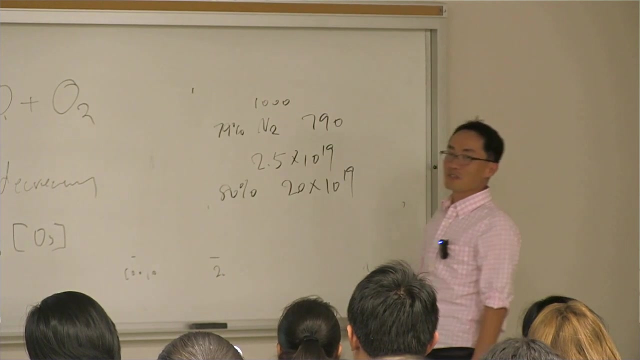 And I will just put some zero in this number. All right, Let's say just 80 percent, And then it's 2 point. So what's the difference between this calculation and that calculation Numbers? obviously It's a large number. 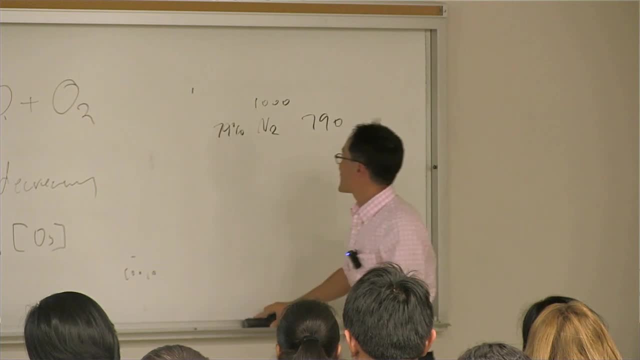 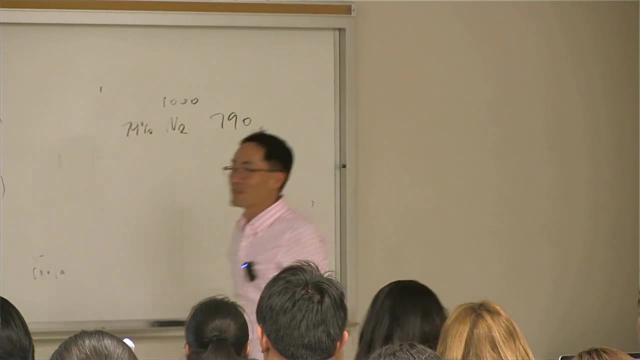 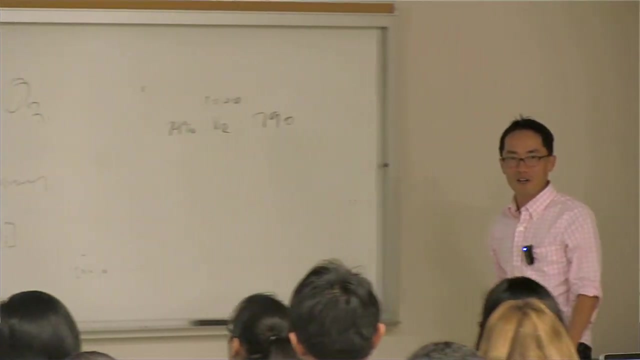 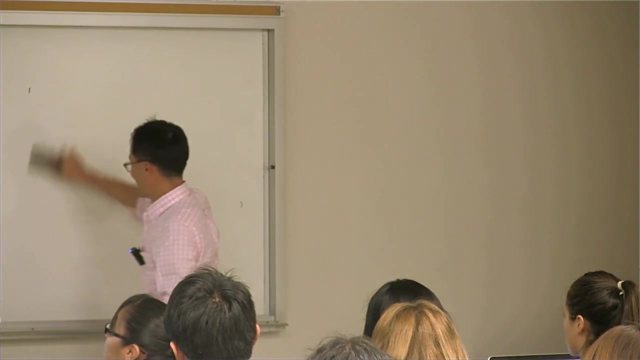 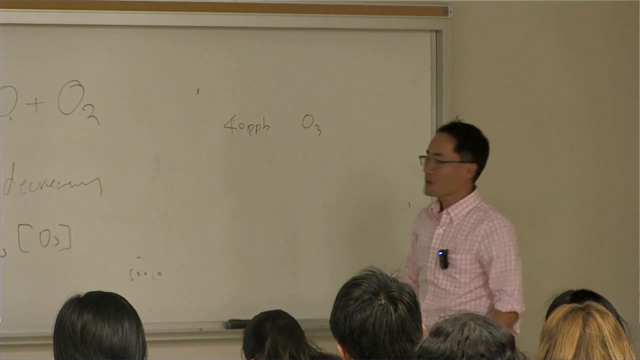 All right, Then just let's stick with this, then All right. So basically you can. now you can convert that number of molecules, scale in given volume, And let's assume 40 ppb of ozone. So what's the definition? 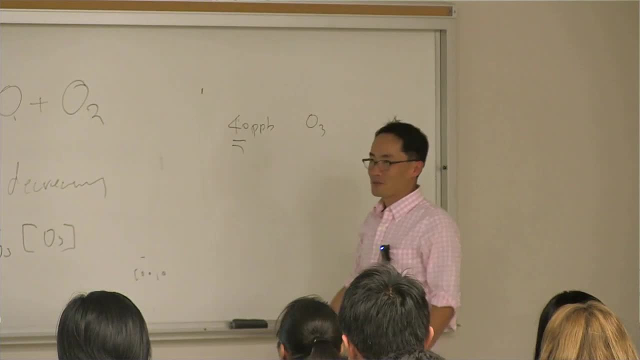 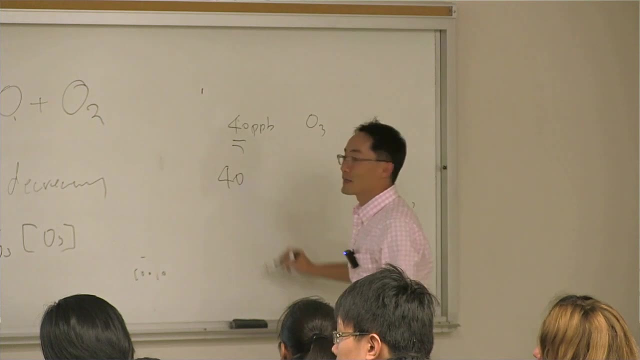 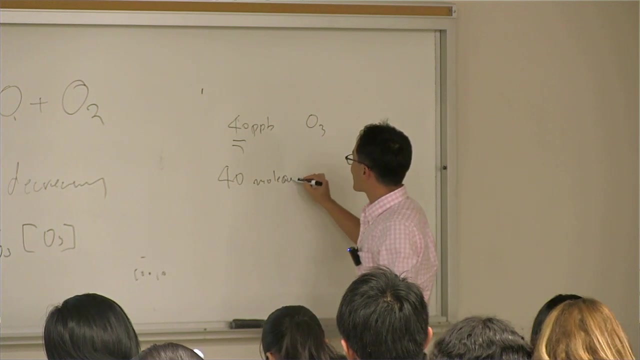 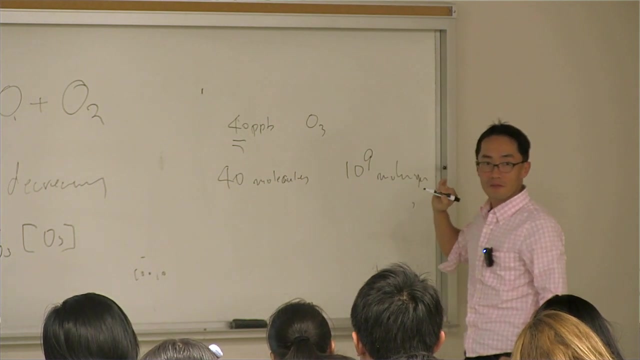 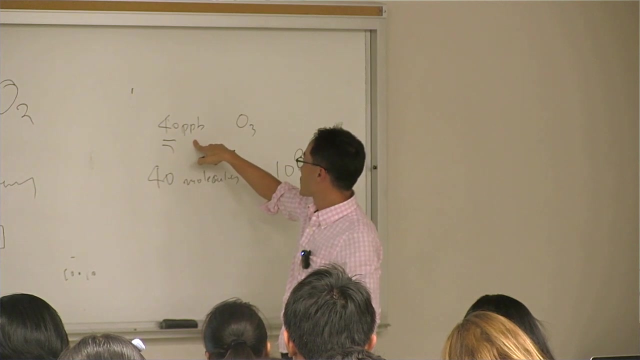 of this thing. Yeah, that's basically reading, So let's go a little more deeper than that. Go for it. There's 40 particles of ozone, molecules of gas, right, Is that right? So this is kind of fraction. 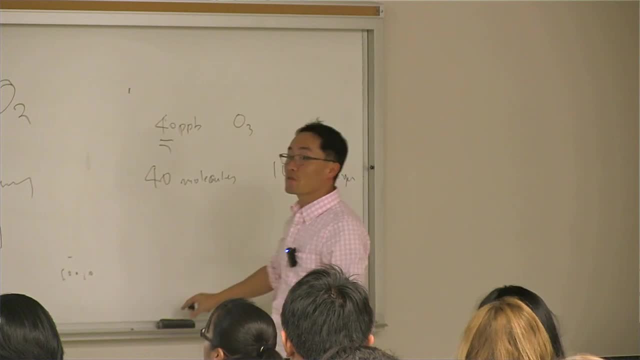 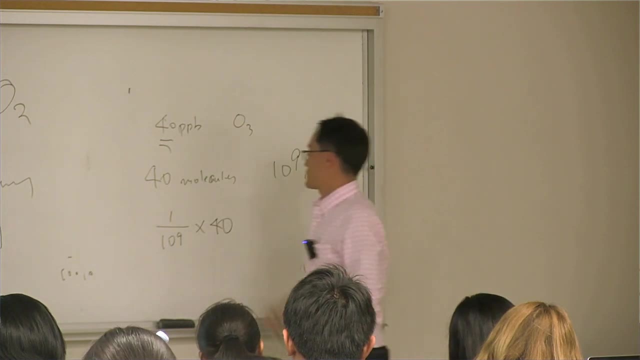 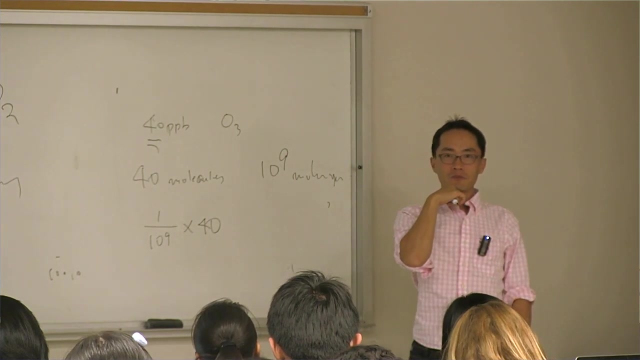 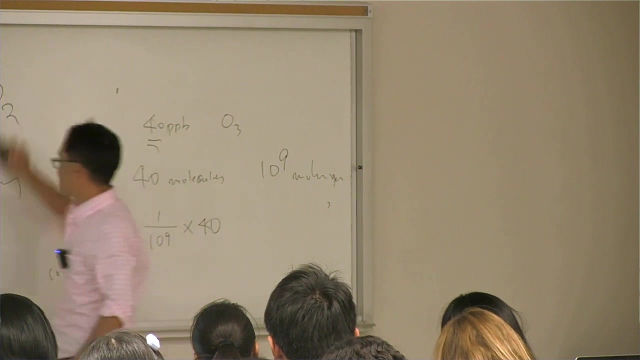 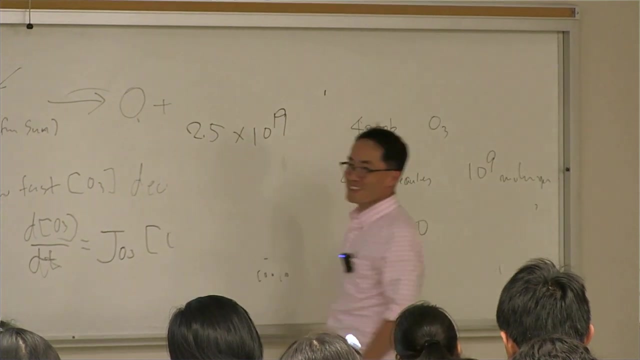 And although we call it this ppb, so this is basic scalar right. So in terms of the atmosphere, Is that right? Everybody's with me, All right. And then let's bring that big number here which is: 2.5, 10 to 19 molecules per cubic centimeter. This is the number of molecules that are actually ozone in this number of molecules. okay, Then what are you gonna do? You gotta just multiply this thing into this 10 to. 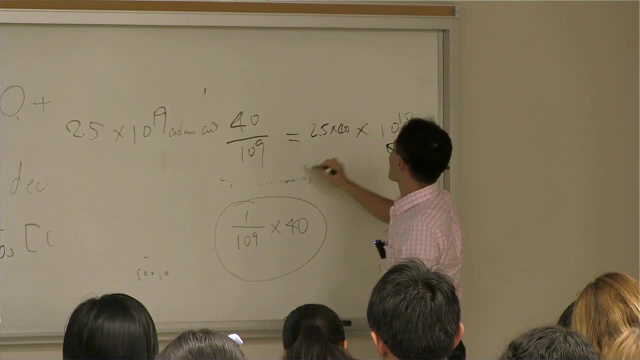 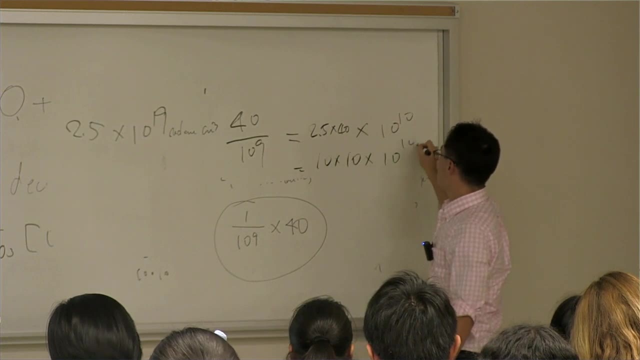 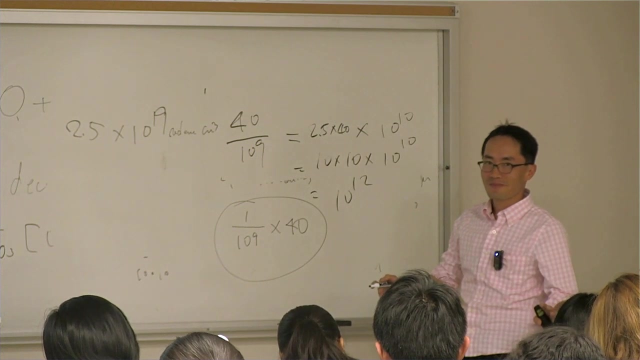 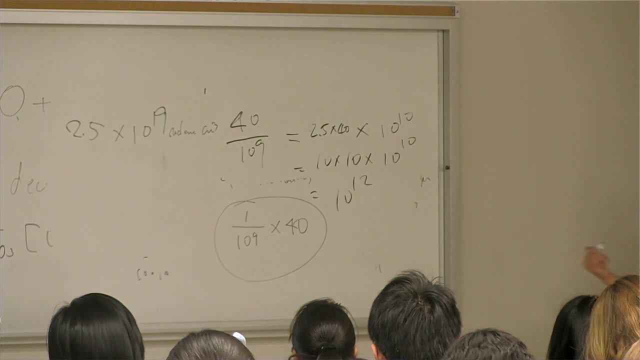 10,, 2.5 times 40, right? So 4 times 2.5 is gonna be 10, and then you have another 10,, 10,, 10,. wow, the sum of 10 molecules. 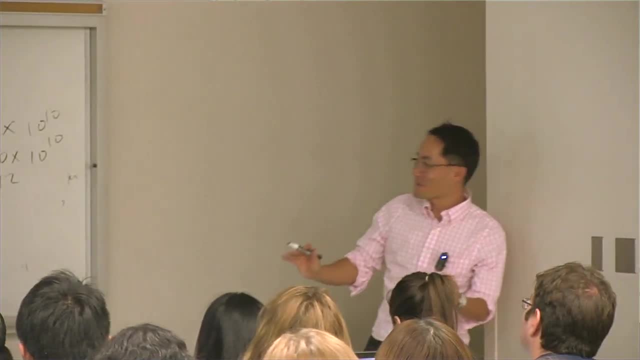 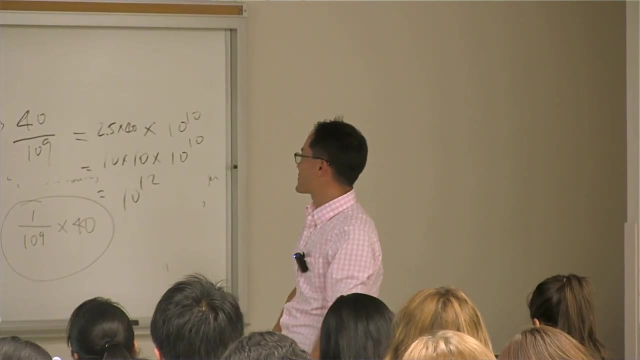 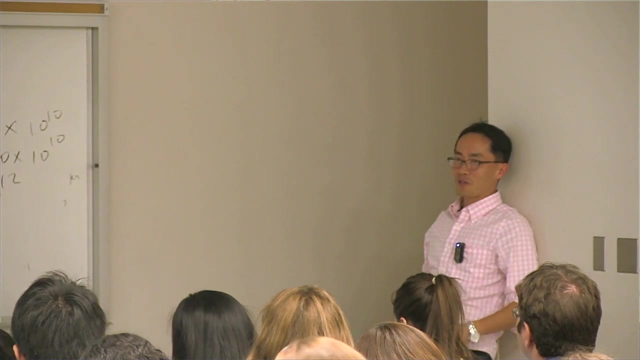 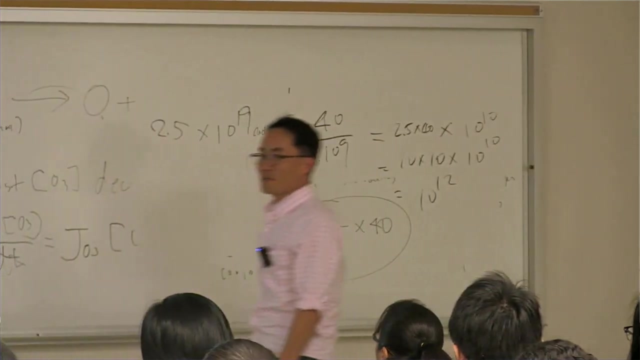 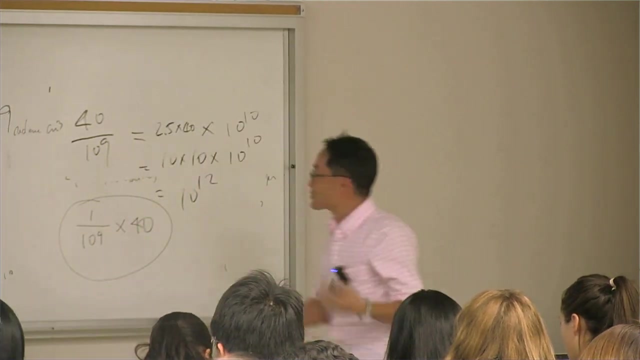 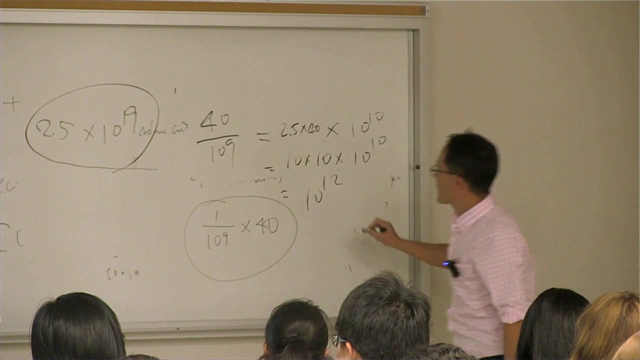 in the atom. Just don't get freaked out the big number, because there's simply there's too many molecules in the air, so we need to deal with a lot of molecules in the atmosphere. That's all I just try to do out here. 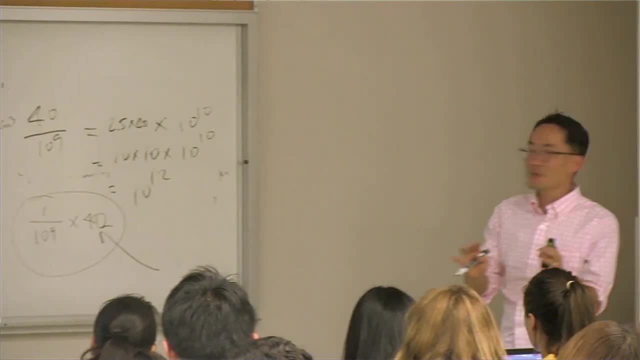 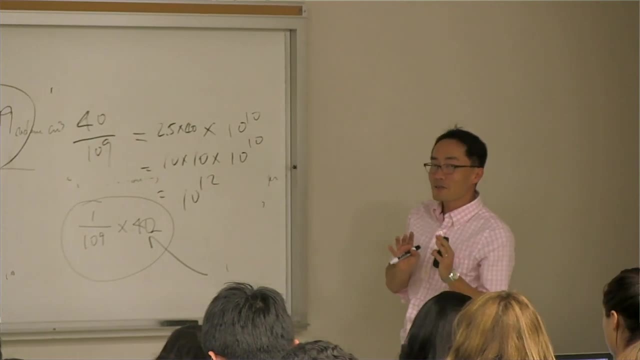 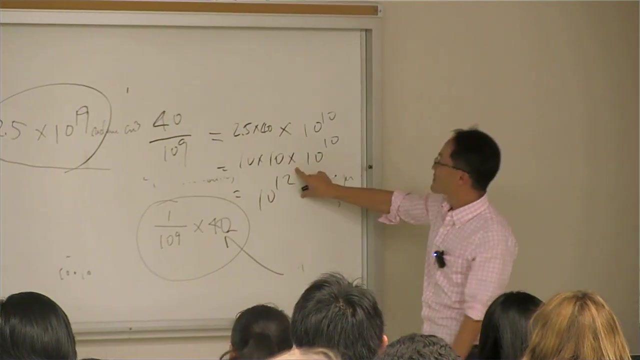 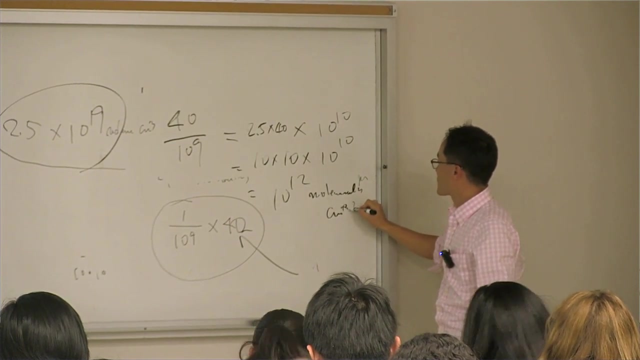 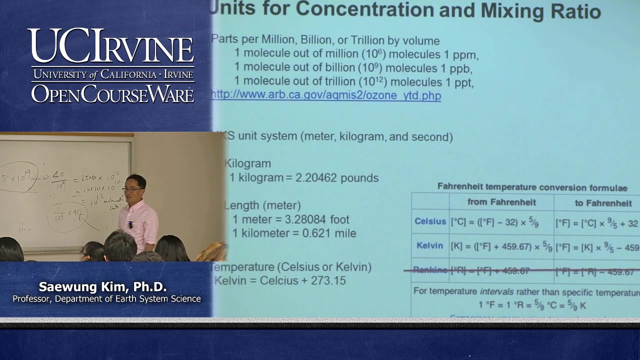 right. So this is number of molecules in the one cubic centimeter, and then the pollutants we are dealing with are very large number of molecules. molecules cubic centimeter. Okay, But it's fine, it's, it can be very. 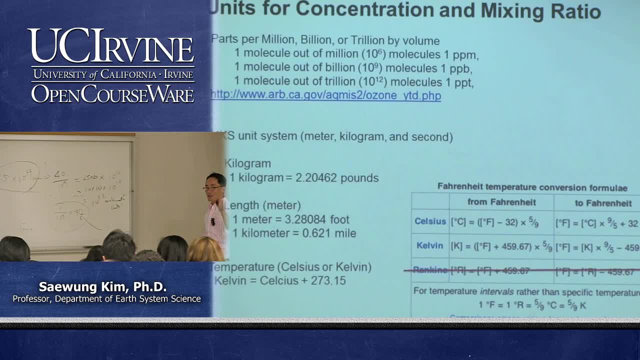 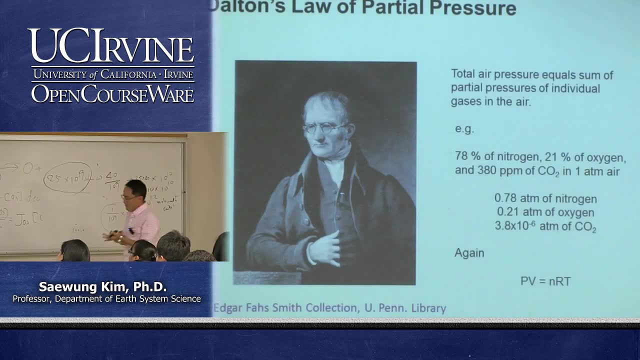 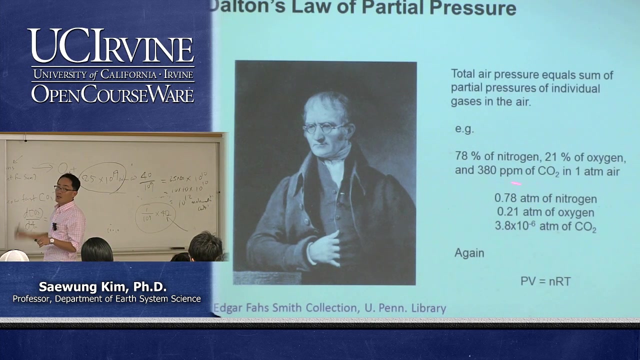 confused, but we will go over this thing over and over again. so, and then Ian is back there. he's going to talk about the momentum of the atmospheric atmosphere and then the atmospheric pressure ratio, which is the ratio of the atmospheric atmosphere. with the atmospheric pressure ratio, fraction of their gas into a pressure which is 78,, 0.78 ATMs are coming from nitrogen, then 0.21 ATMs are coming from oxygen. Therefore, in terms of CO2 is 360 ppm parts per million. 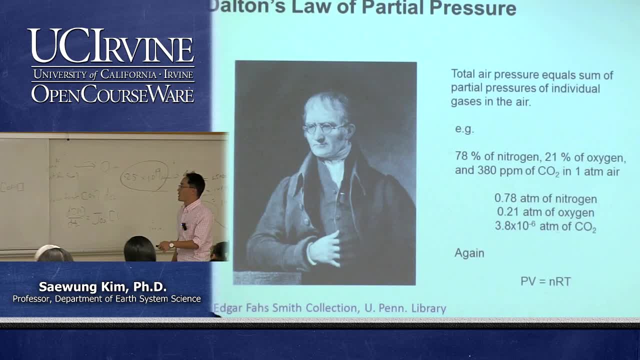 So 3.8 times 10 to the minus 6 ATM, the pressure are coming from CO2, okay, So this is kind of how you can use this equation. So, okay, this is a lot of numbers. So basically this: 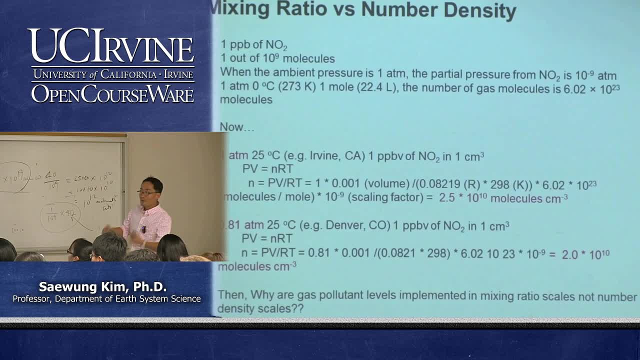 is what I try to explain here. So if you are confused while you are solving number three, you can take a look at this, or just you can simply come see me during the office hour that I will go over this thing over and over again until you understand this, all right. 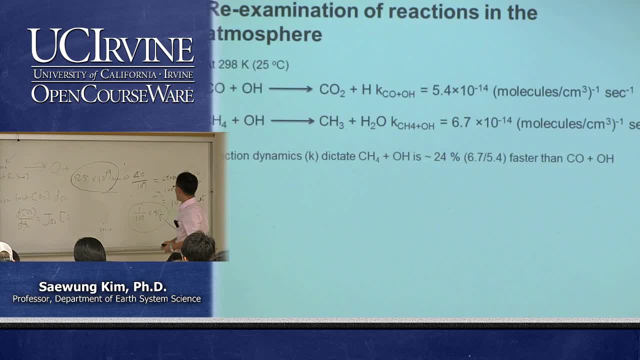 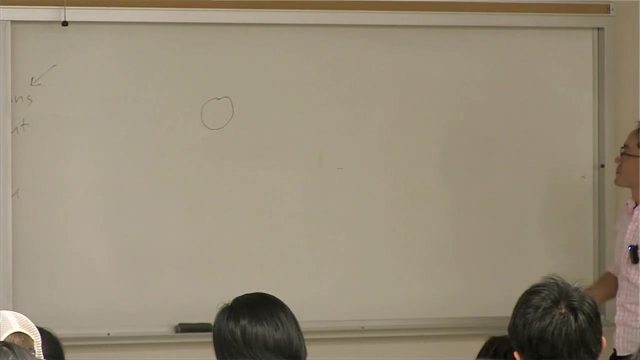 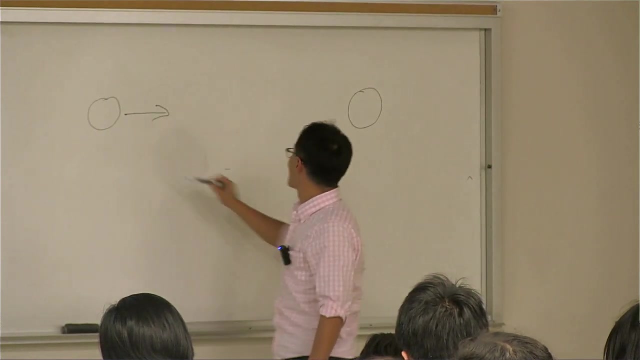 Or you can see your T8 back there. So let's go back to the reaction in the atmosphere. all right, So let's imagine the gas molecule- gas molecule here, and then what's the speed of the gas molecule It's about 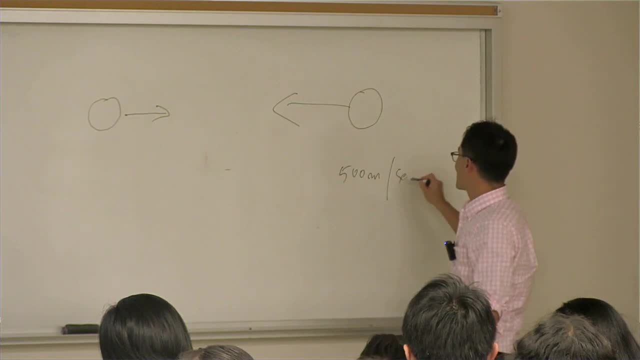 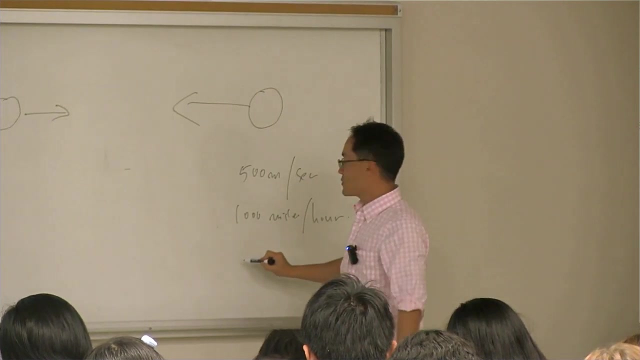 500 meters per second. 500 meters per second in the room temperature, which is about 1,000 miles per hour. right, And there's how many molecules in one centimeter cubic centimeter? 2.5 times 10 to 19 molecules. 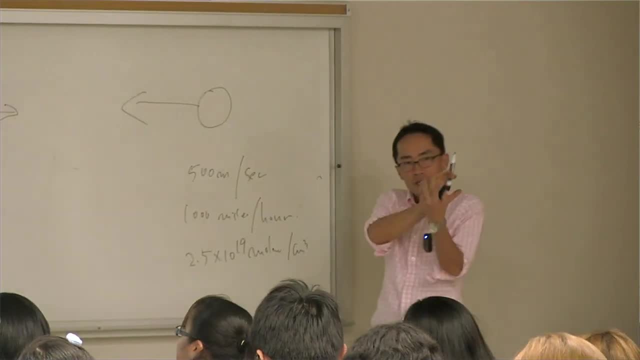 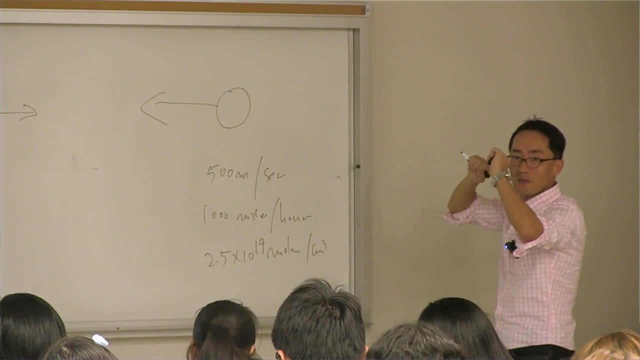 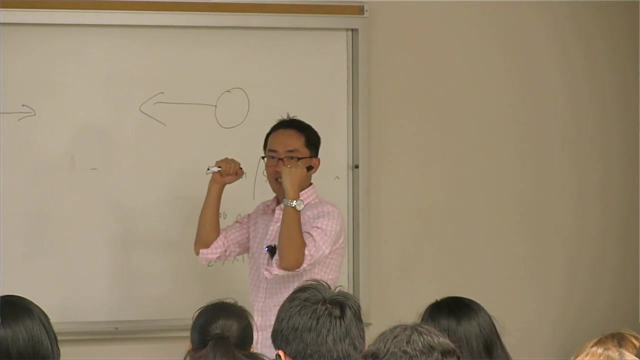 in one cubic centimeter right There's a lot of molecule in the atmosphere and then they are traveling very fast. And then what's going to happen? if they are traveling very fast and then there are that many molecules in the atmosphere, Then they tend to hit each other right In very fast. 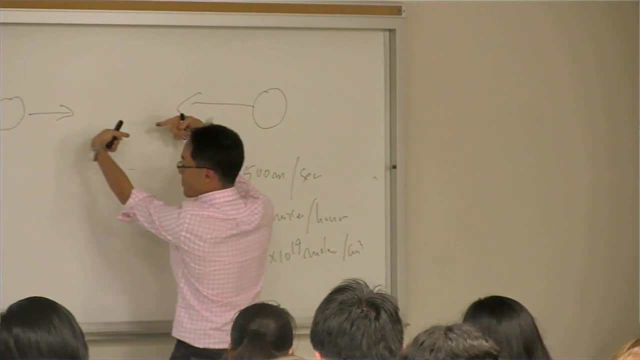 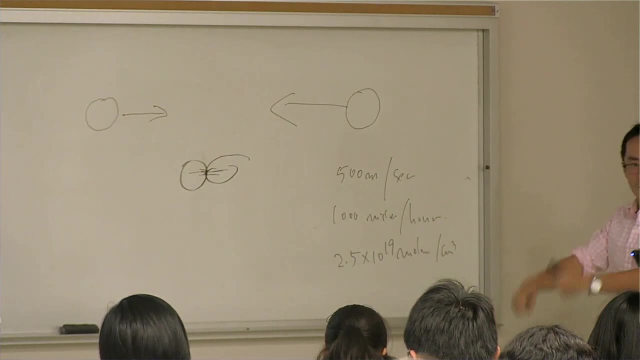 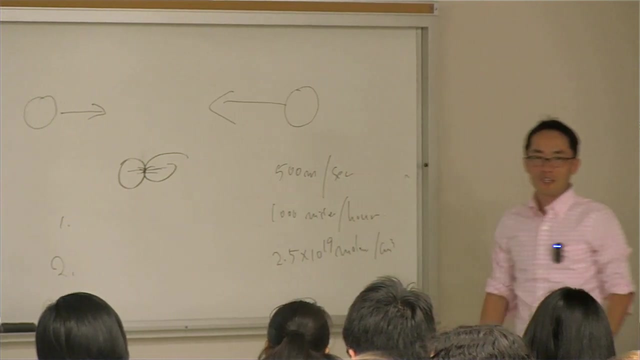 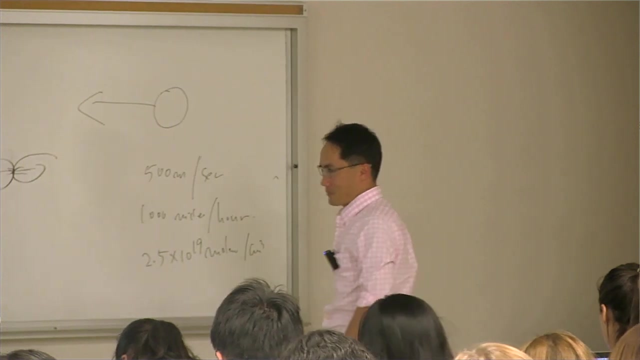 speed. So they are going to come across and they are going to hit each other. Collision is happening. Then there's two possibilities. What's going to be the two possibilities? Anybody? Yes, They react and combine, or they just knock each other off. right? 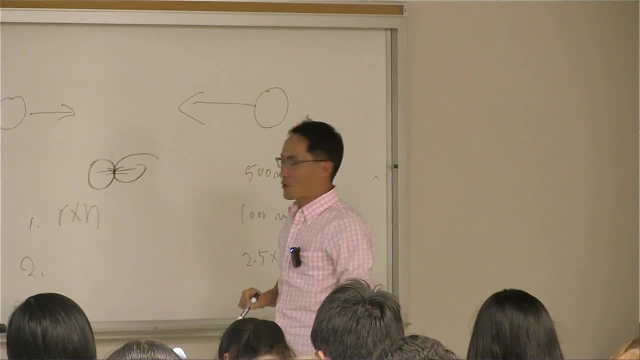 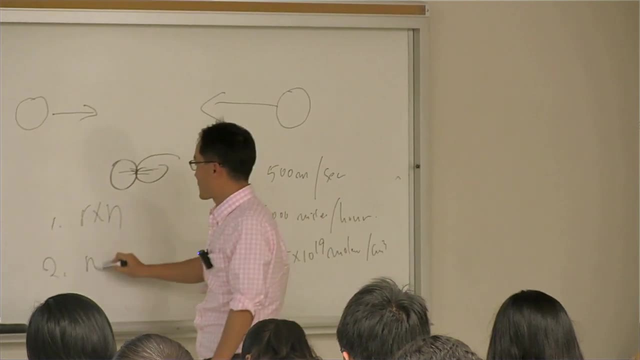 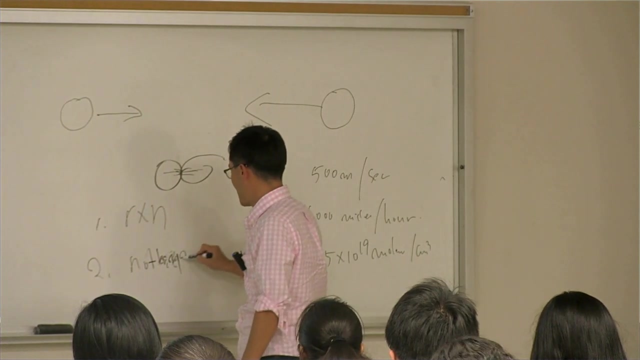 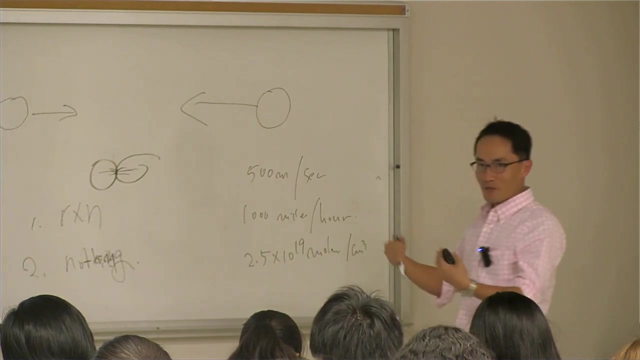 Yes, They can make reaction, or they just bounce, beg each other and then nothing happens. Okay, Okay, Okay, Okay, Okay, Okay, Okay. in between There's two things: They do something or nothing happens. It just bounces back away. 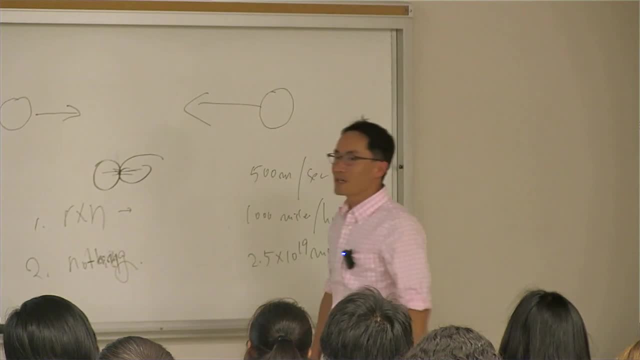 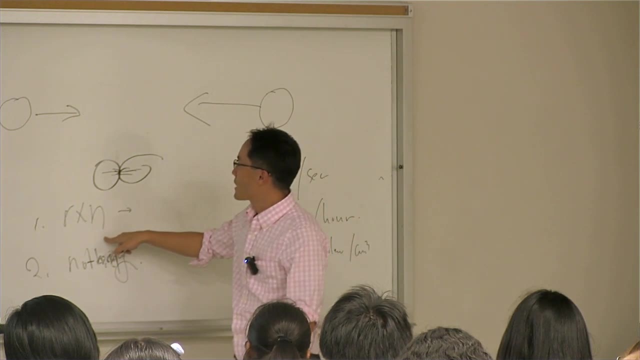 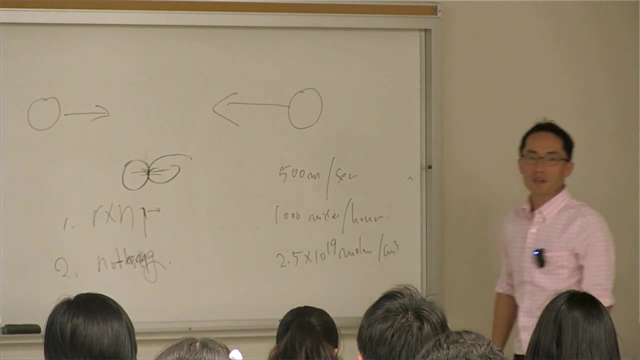 So some of the gas in the atmosphere happens to be very reactive, Then the possibility that reaction is going to be actually happening is going to be higher. But if it is not that reactive gas in the atmosphere, like nitrogen and oxygen, although they hit each other, 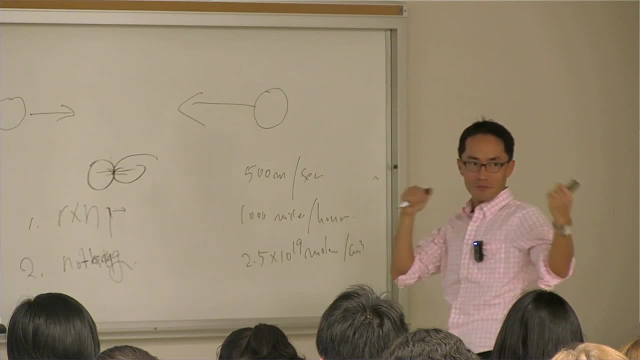 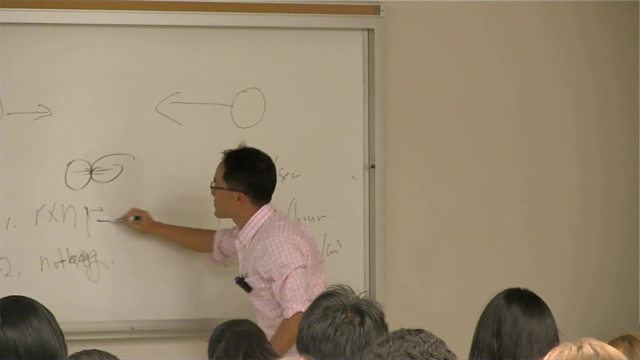 nothing is going to happen. It's going to be bounced back. That's the definition of their reactivity. If it is very reactive once they hit each other, then reaction is going to be happening. If it is not reactive, then nothing is going to happen. It's going. 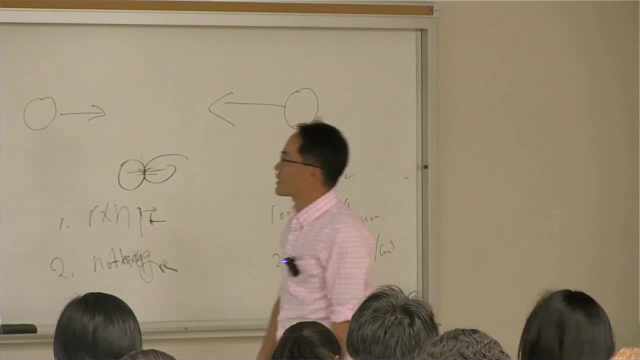 to be bounced back. That's the definition of the chemical reaction in the atmosphere. So this is basically again the reaction. Subtitles by the Amaraorg community. Subtitles by the Amaraorg community. Subtitles by the Amaraorg community. 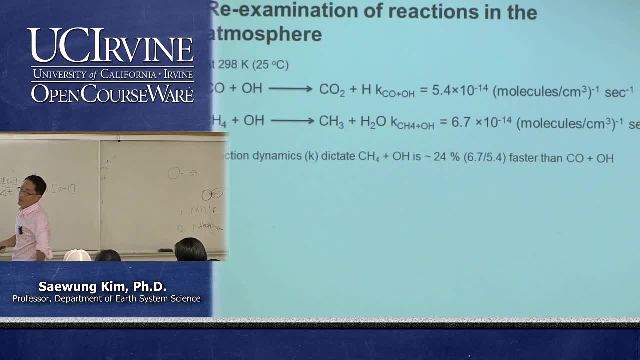 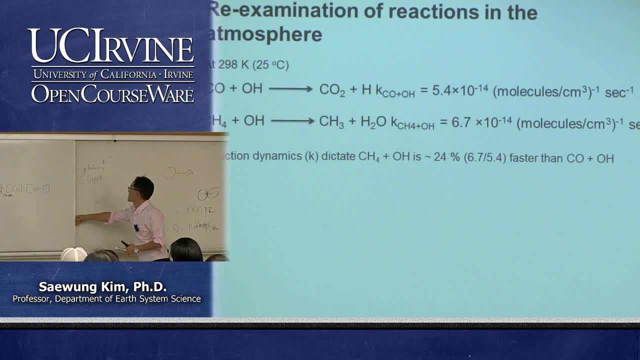 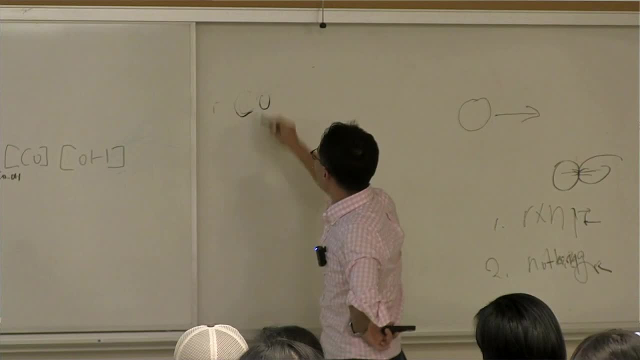 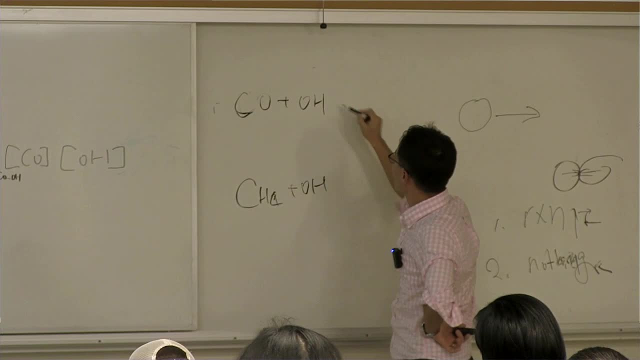 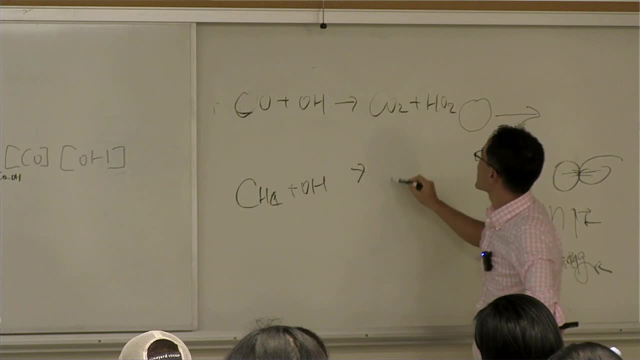 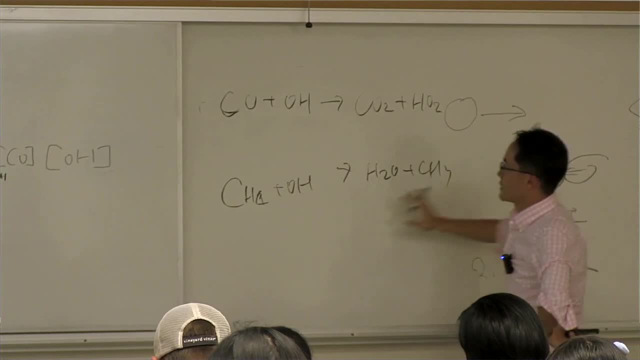 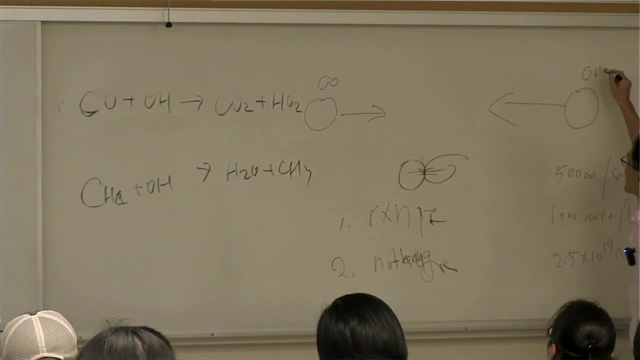 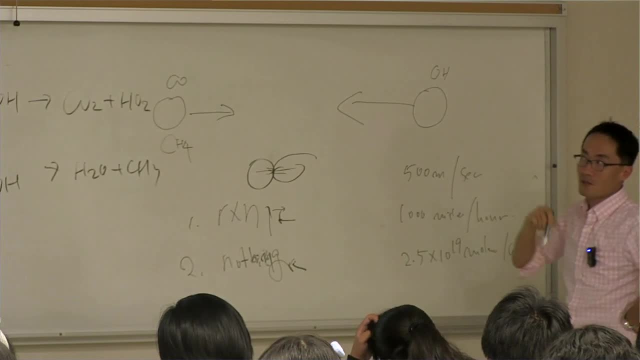 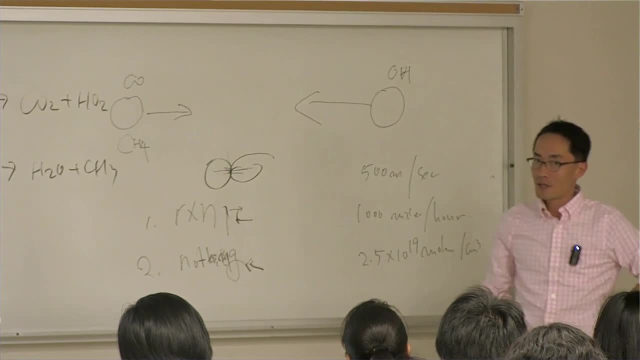 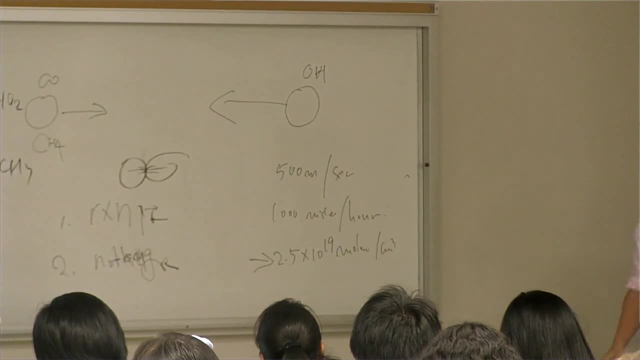 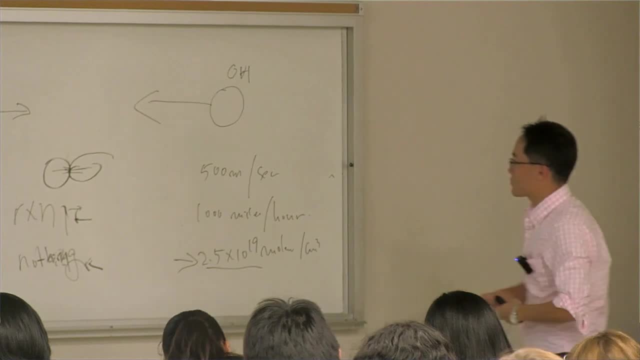 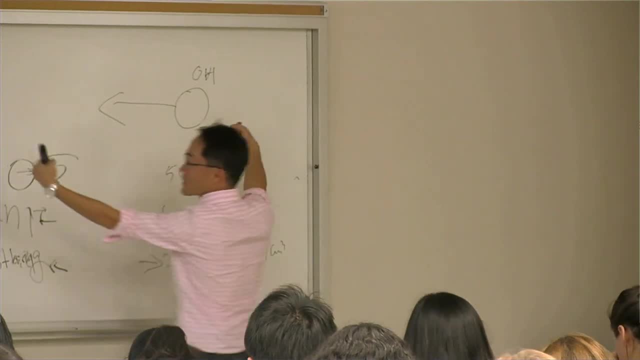 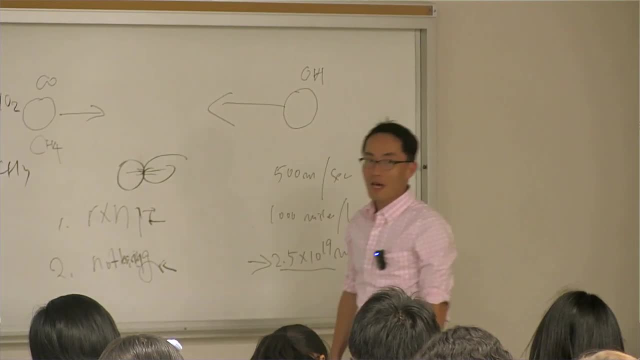 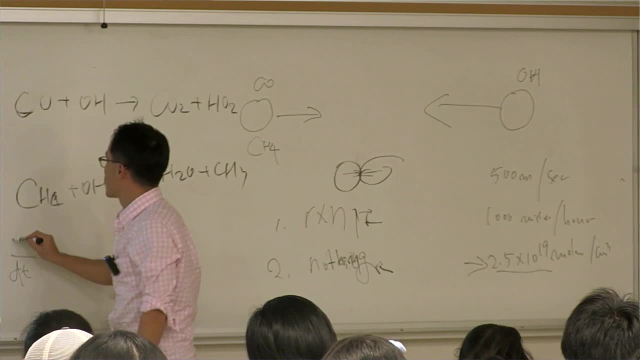 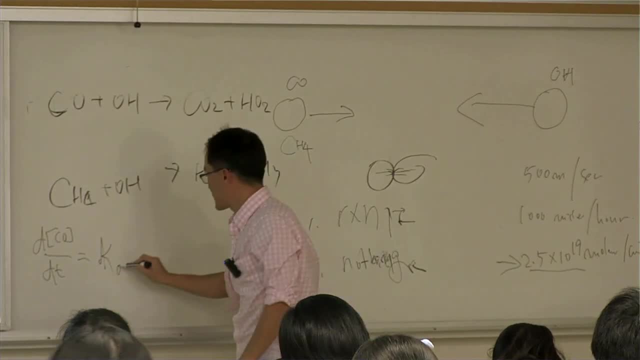 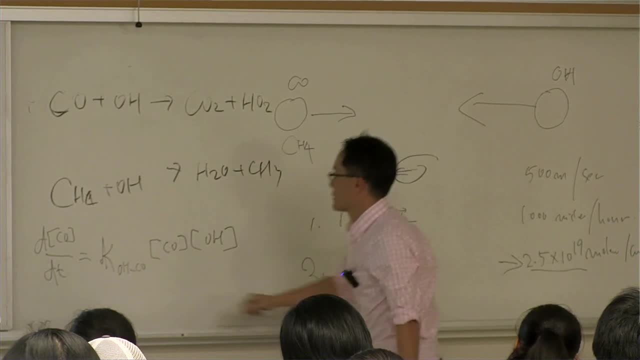 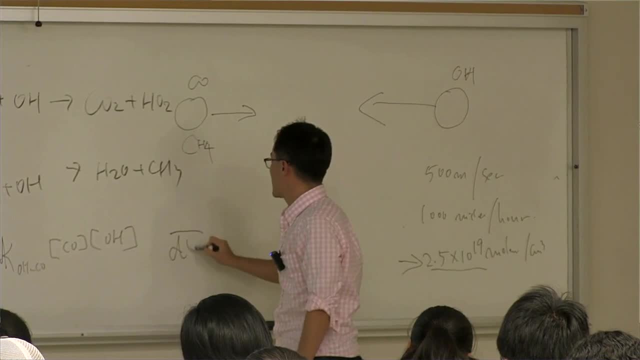 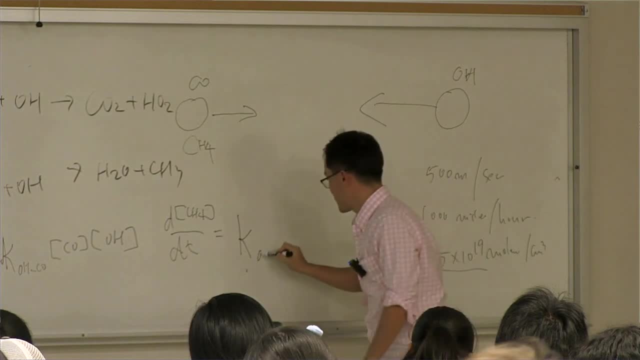 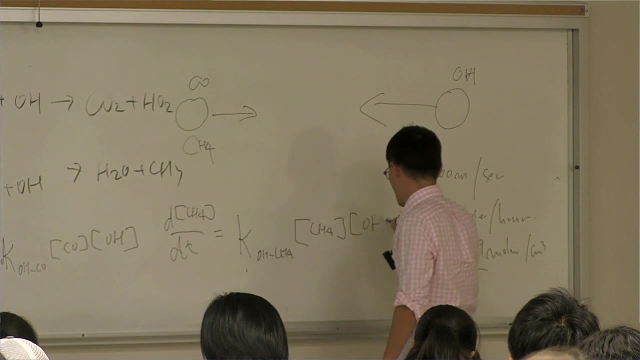 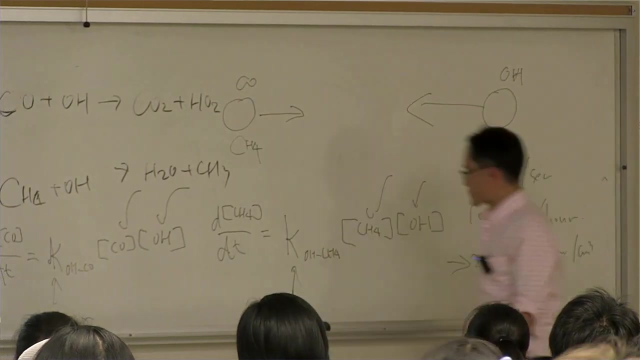 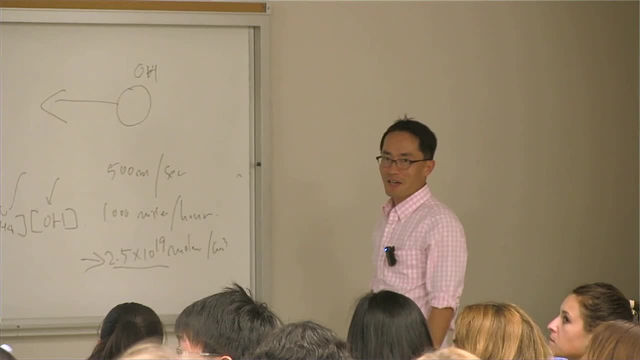 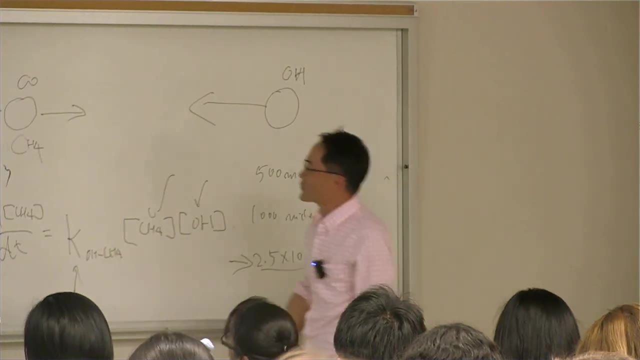 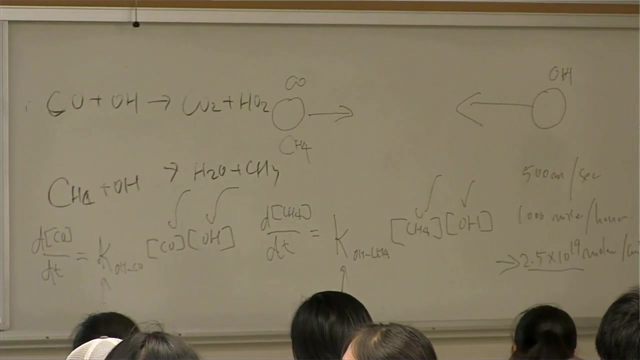 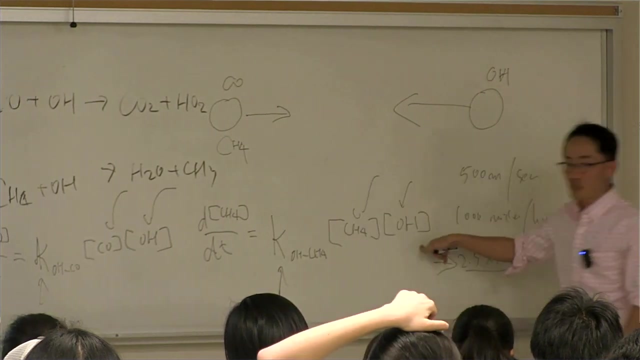 Why every classroom watches always five minutes faster than the actual time. I think probably intentionally. student did the thing. So basically, this concentration terms that determining this decreasing rate of the air pollutants. So why concentration term is here? Because if there's higher concentration of this molecule in the atmosphere, basically 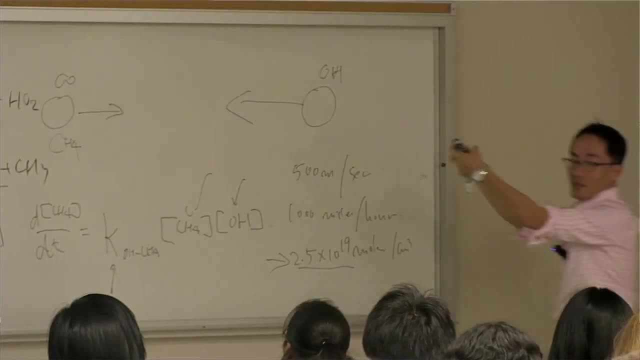 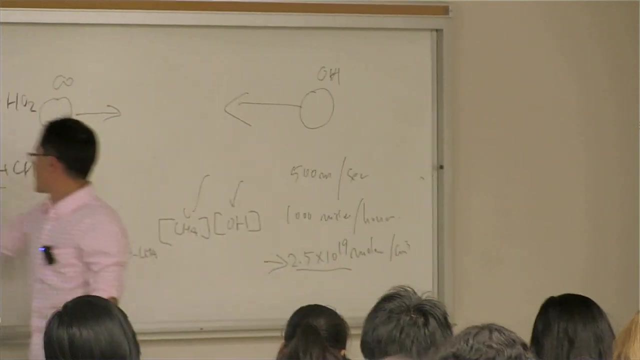 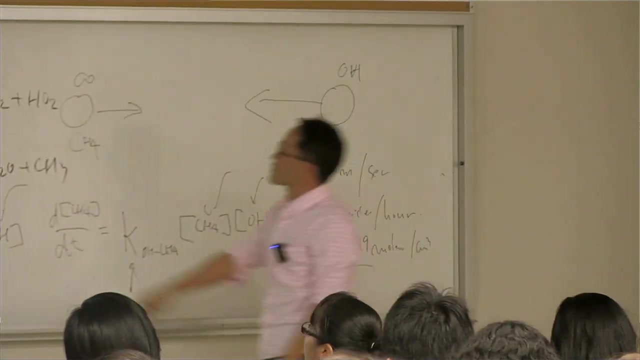 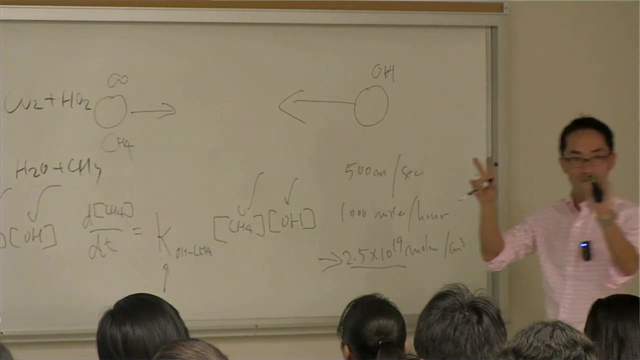 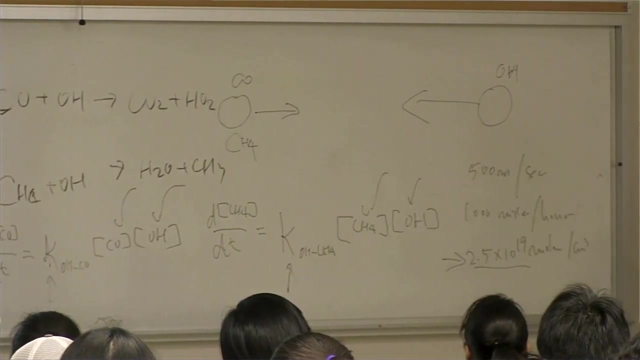 these molecules are more in the atmosphere and then there's high possibility they are going to hit each other right. So that's why this reaction rate- It correlates with the concentration of the molecule that actually participating the reaction Make sense, Because if there's more molecules there's a higher possibility they are going to hit. 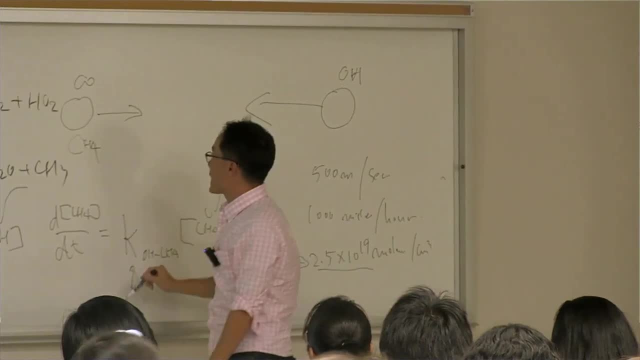 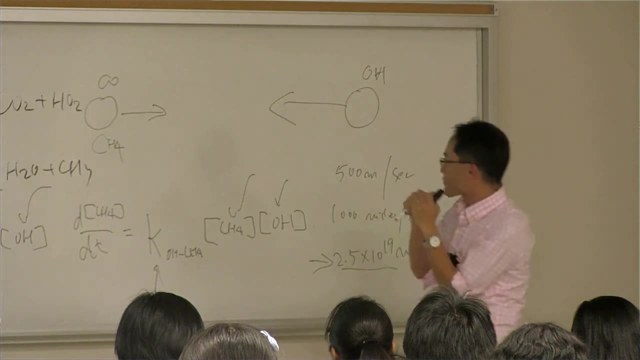 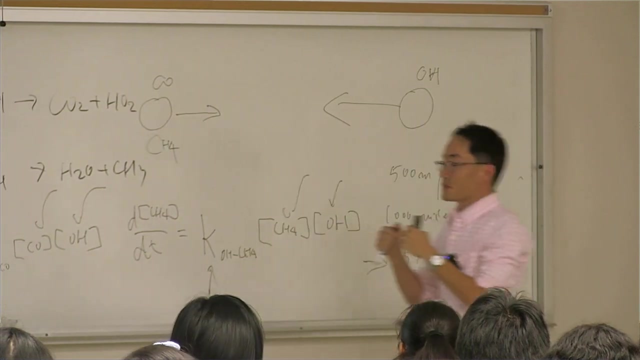 each other. right, That makes sense. And then I also explained that, although it hits each other, some fraction of the, the accidents of the, the hit each other, the molecule, it's going to actually lead to the reaction, or some fraction of the collision, it's going to be just ended. 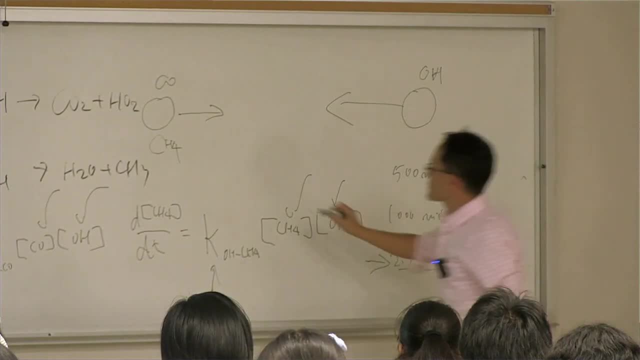 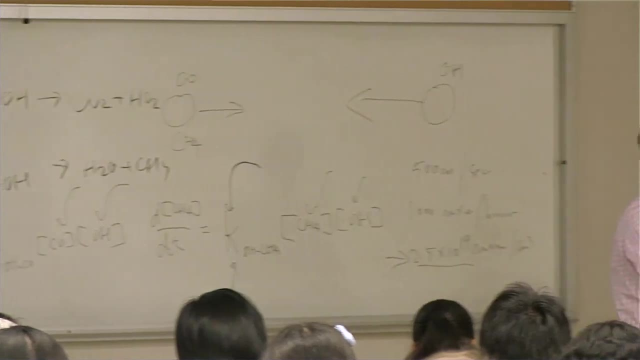 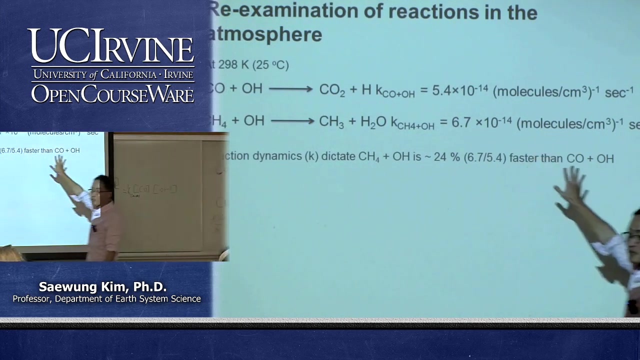 up bouncing back each other of the molecule right. That thing is determined by this reaction constant, basically possibility right of the reaction is going to actually happening or not happening. So for, in this case, just forget about this minus 14, that may confuse you, but if you 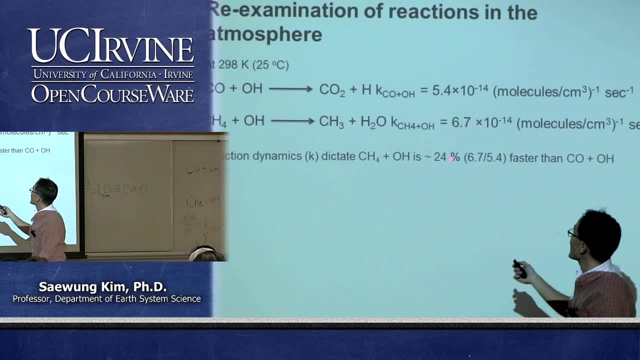 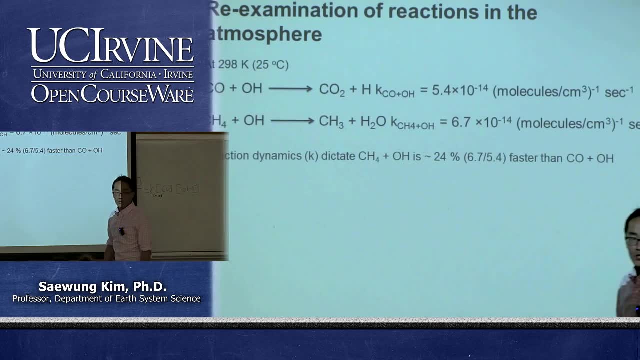 take a look at this: 5.4 and 6.7, so basically this indicate that that the methane in the atmosphere is more reactive than the CO, which means that if the CO and methane then happen to the hit with OH Between the atoms, pure the odds are that it's that, in terms of reaction, is actually 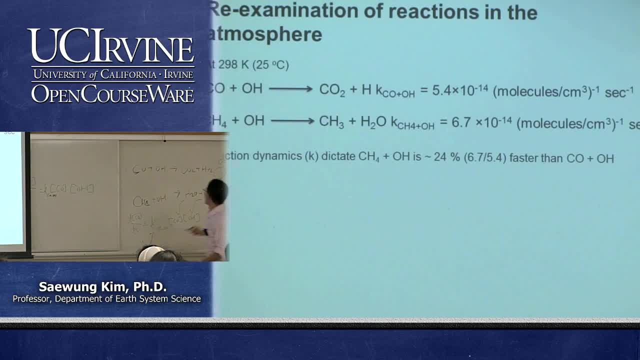 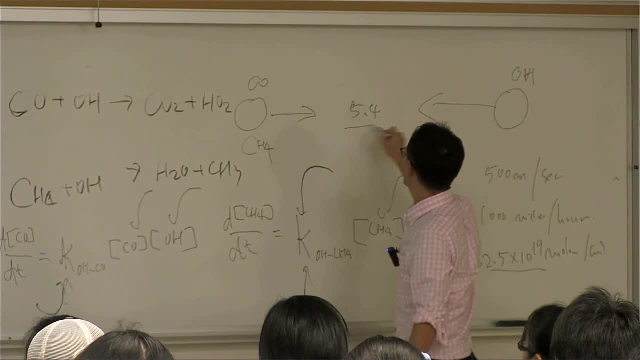 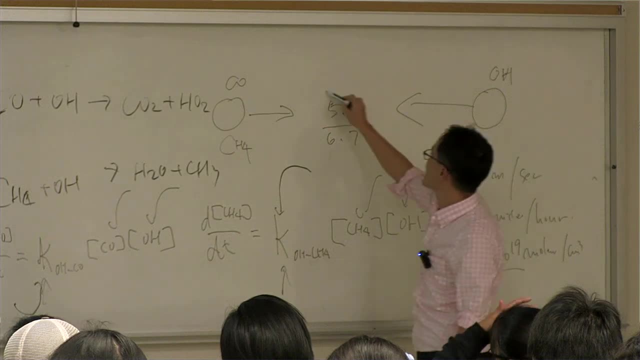 going to happening. it's about: so that's 4.4 and then the 6.7,. it is about, let's say it was 7.4, I don't know. So this is the difference between the reactivity of the CO and the OH. 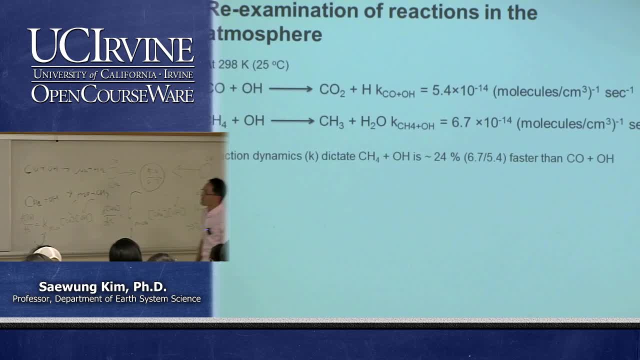 And methane, which means that actually the methane is going to be more reactive in the atmosphere towards the OH, which means that if same concentration of CO and methane in the atmosphere, then methane is going to be more fastly removed from the atmosphere. Basically that is determined by this reaction constant, okay. 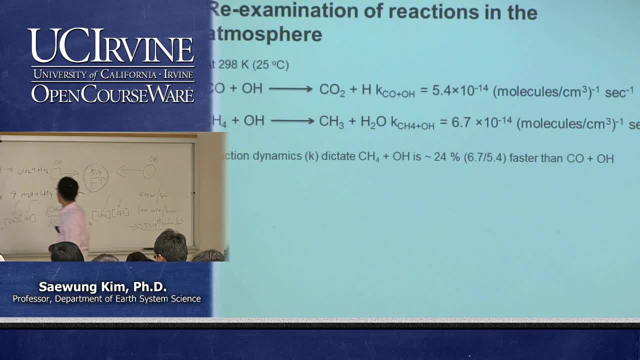 Maybe that's a little too far, But all you need to know is that. So reaction dynamics: there are two important things out there. One is they need to hit each other right, And then the reaction is actually whether reaction is going to be happening or not happening. 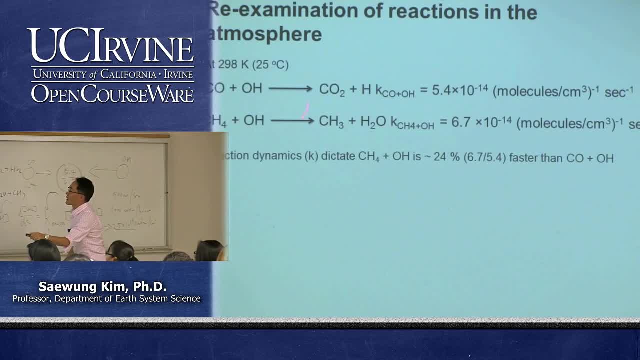 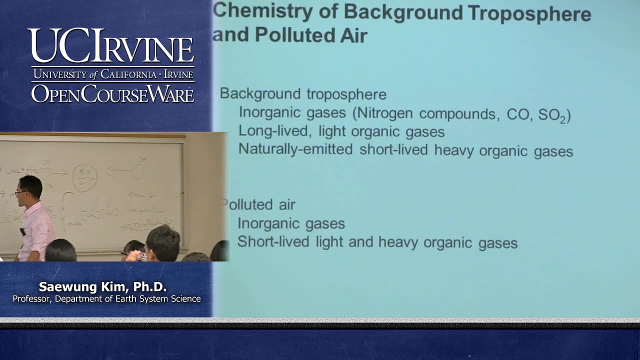 so pretty much determined by the reactivity of the gas molecule, And then that is mathematically expressed by this reaction: constant, okay, So that's physical meaning. Let's skip this thing. So you just learned that most difficult stuff during this whole class. you will refine after. 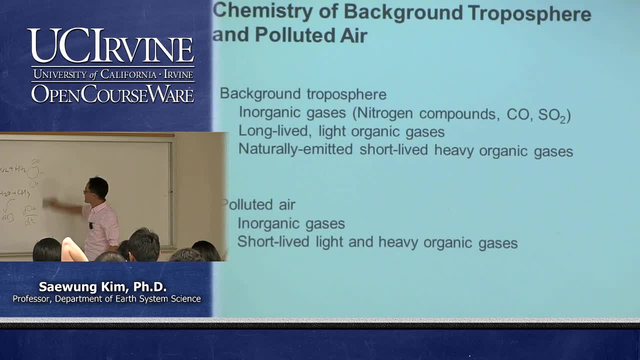 this. So let's talk about real air pollution now. all right, We talked about a little different thing past an hour or so, So we will talk about background air, which is before the air pollution, And then polluted air. So even in the background air there is a tiny, very low concentration of the nitrogen. 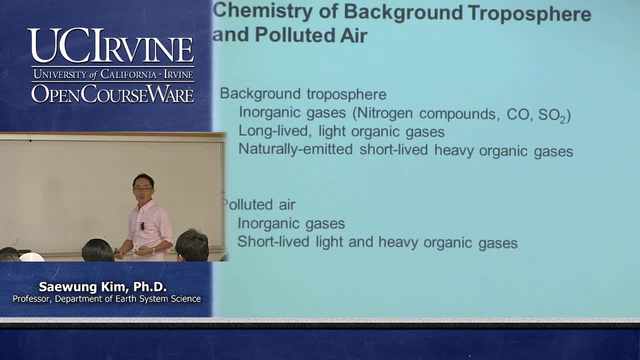 compound which is NO and NO2.. And then CO can be coming from wildfire, things like that, actually caused by natural reason. There's CO, there's a little concentration of CO out there, And then SO2 can be coming from natural processes, which is most important one that actually 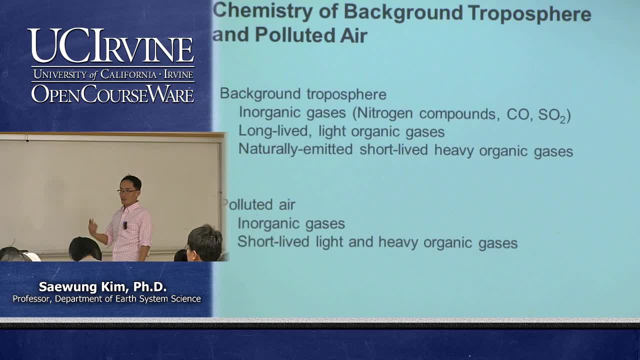 the natural process that emits SO2.. We talked about it: volcano. volcano emits a lot of SO2.. And then CO can be coming from the wildfire. Actually, NO and NO is also coming from the wildfire. And then there are some background organic gases also coming from the trees, things like 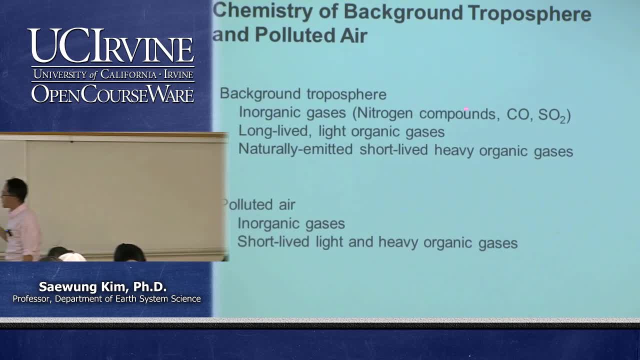 that. But the problem is we add more higher concentration of this nitrogen compound and CO and then VOCs, volatile organic compound, Actually, it's CO, Actually that cause excess production of ozone and then that make the building up. 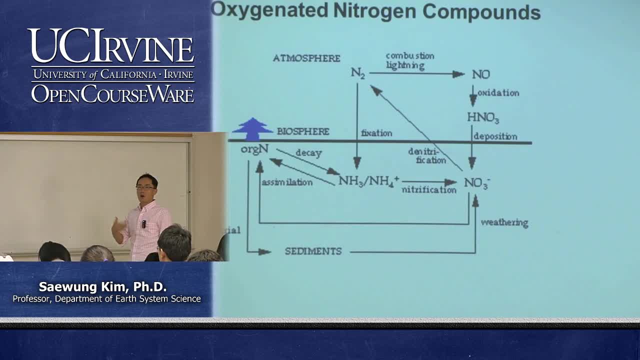 the ozone in the atmosphere. So we will talk about today, we will talk about the background atmosphere, And then next class, we will talk about how people can- people's pollutants can- produce excess amount of ozone that can be actually harmful to the human health. 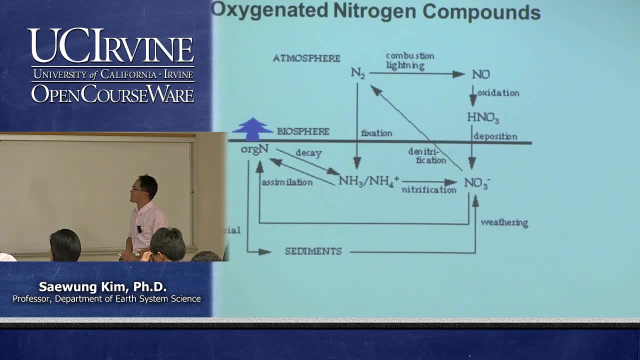 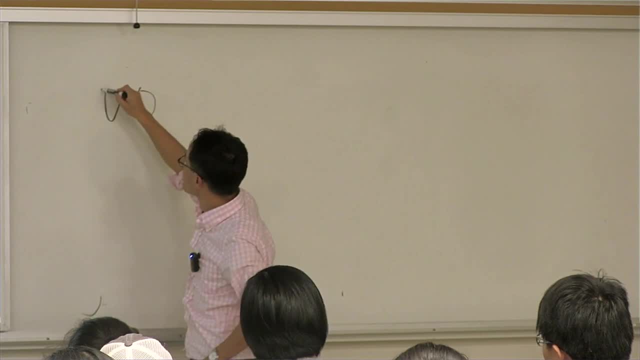 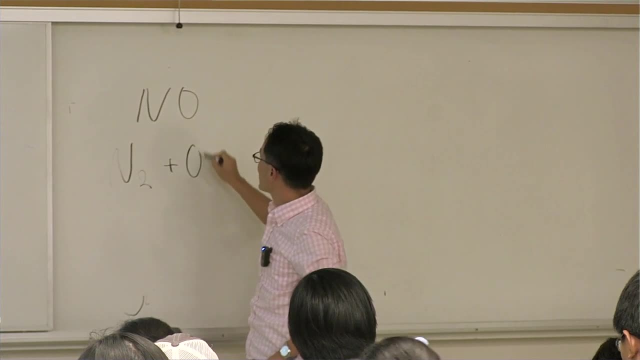 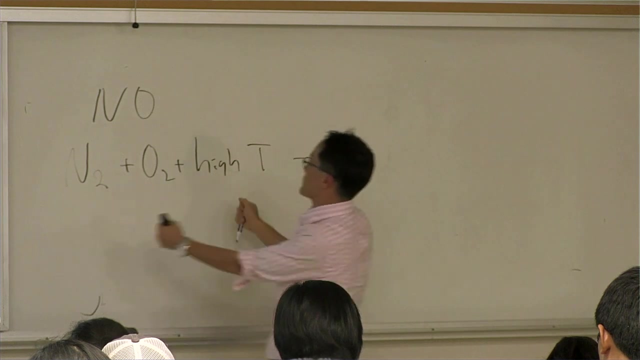 So this is the nitrogen oxide compounds formation: Nitrogen oxide, which is NO. I explained that NO is coming from N2, NO2, then very high temperature, that's bonding, got broken nitrogen and oxygen molecule and then produce NO. 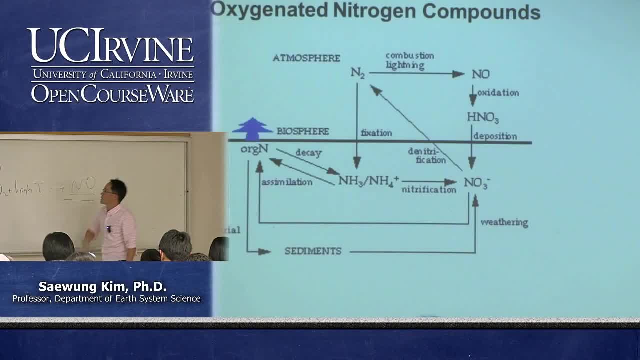 Right. So there's many different ways Actually: nitrogen oxide which is NO, Nitrogen oxide which is NO, Nitrogen oxide which is NO Right, So naturally NO can produce. One is combustion, wildfire and lightning. So lightning in the atmosphere. that is very high energy actually kind of eliminating in the atmosphere so that bonding between nitrogen and oxygen can broken up. So naturally there can be NO it's coming from, can come out from those reaction And then also in the soil. 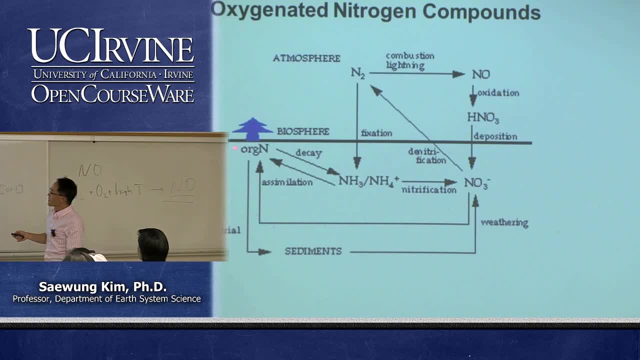 Actually there's a small bacteria thing. it's decaying the organic nitrogen and then they, just by breaking up this chemical bonding, they actually produce the energy they need, and then they actually emit a small trace amount of NO to the atmosphere too. 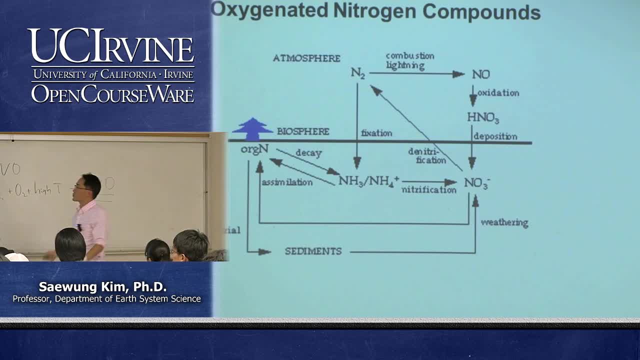 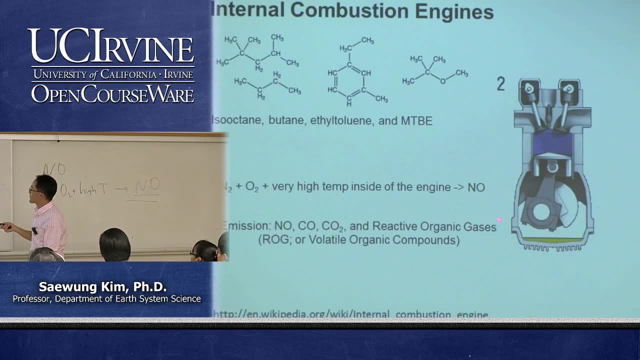 So they are a natural source of the NO in the atmosphere. Now again, the problem of the ozone pollution are mainly coming from this internal combustion. Now again, the problem of the ozone pollution are mainly coming from this internal combustion engine. So I explained in the last class that. so most of your cars, unless you drive the Tesla. 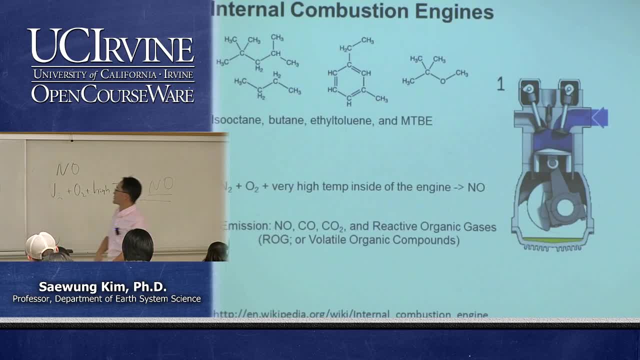 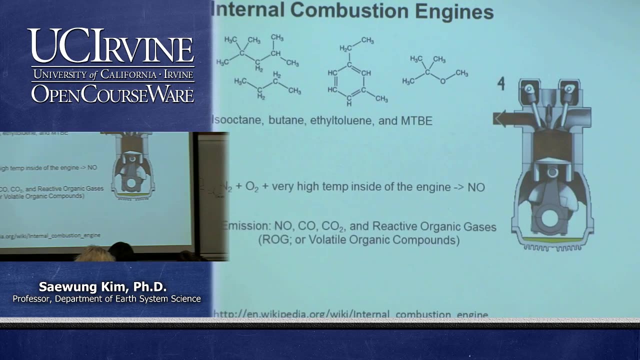 then you have this thing. Even a Prius has this thing, right, Hybrid car has this thing. Then temperature inside is so high it can produce a lot of NO in the atmosphere, right. So probably I just too much confuse you. 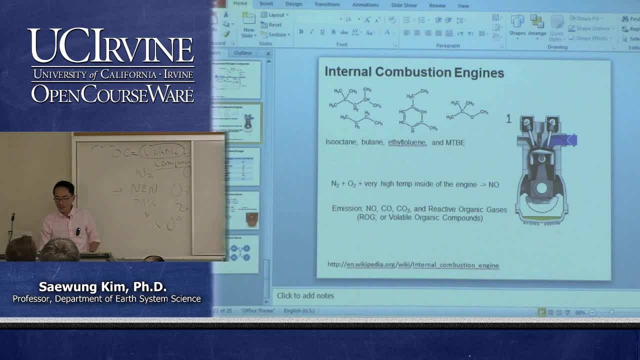 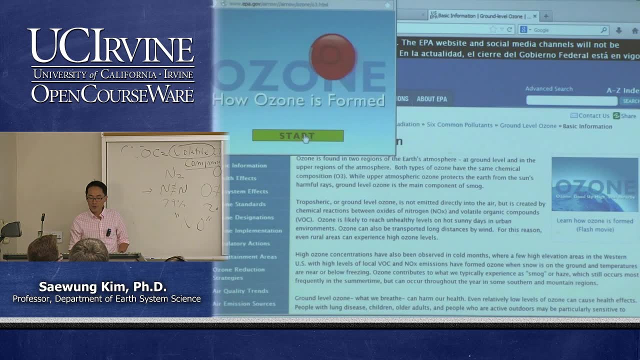 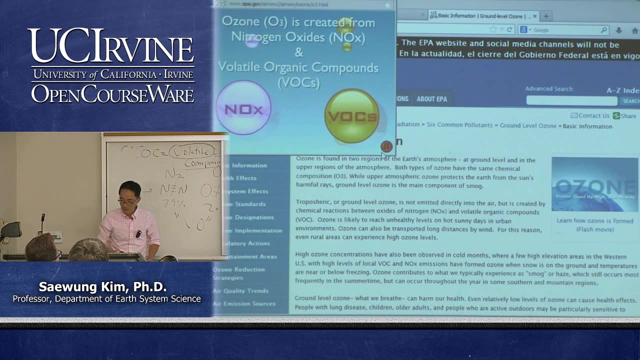 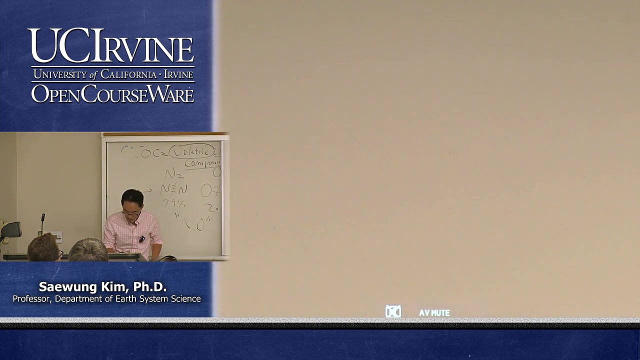 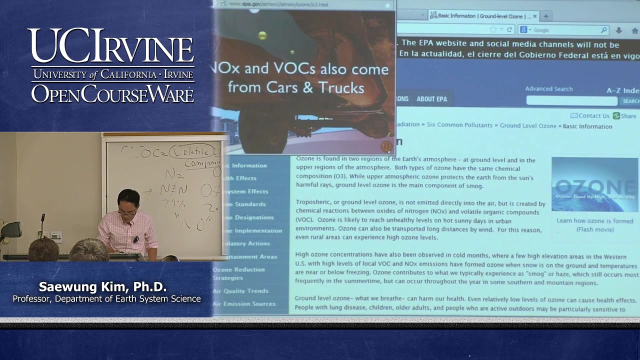 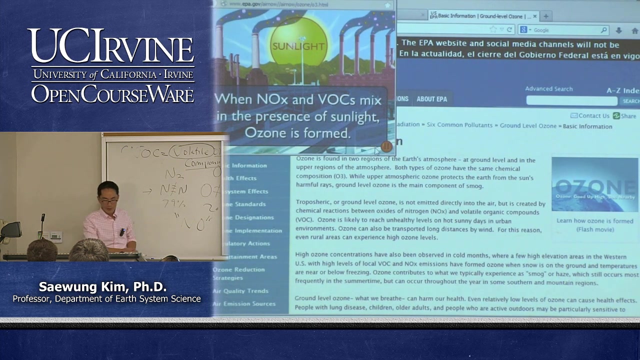 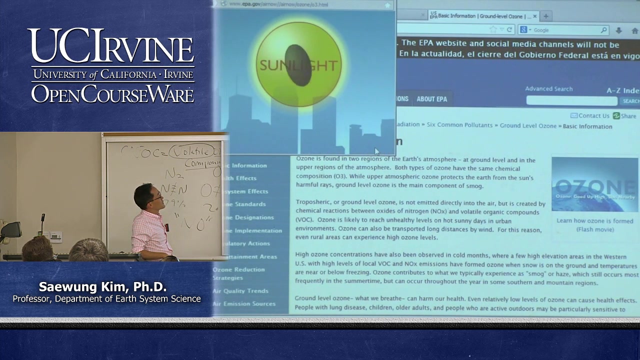 Thank you Today. So let me tell you this. so this is EPA website and they are explaining about the tropospheric ozone. It's there. I'll put some So you have a link on your lecture note, right? You kind of? there's a little voice in there. 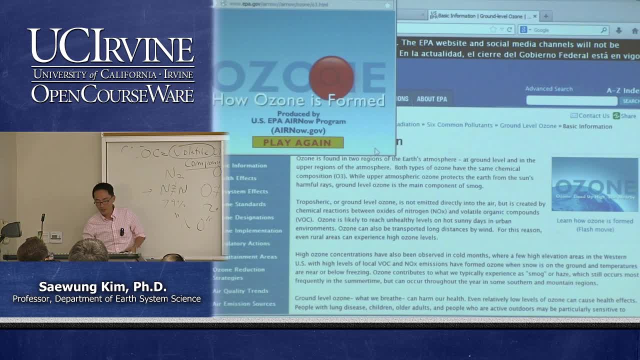 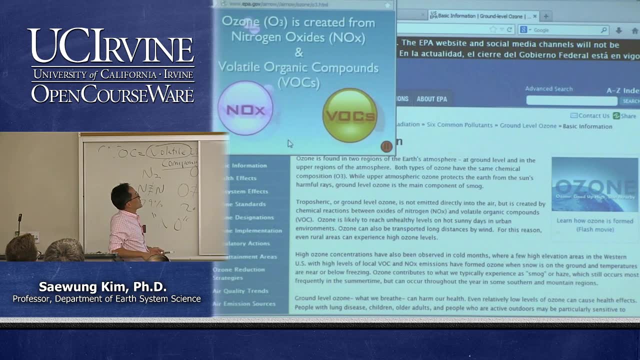 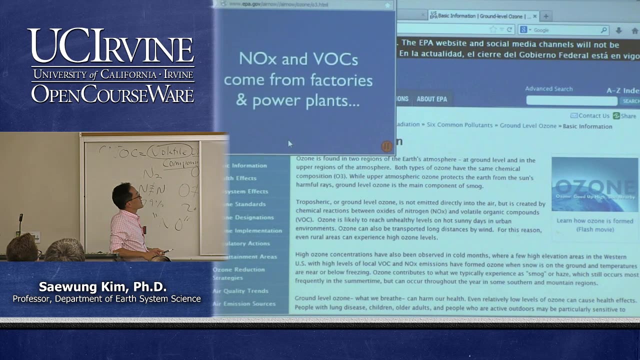 So this is how ozone is made. Let's do it again. It's fairly short, So there's a natural process of the ozone formation, but the problem. so again the NO and NO2 and VOCs are problem. The factories are emitting VOCs, NOx and VOCs. 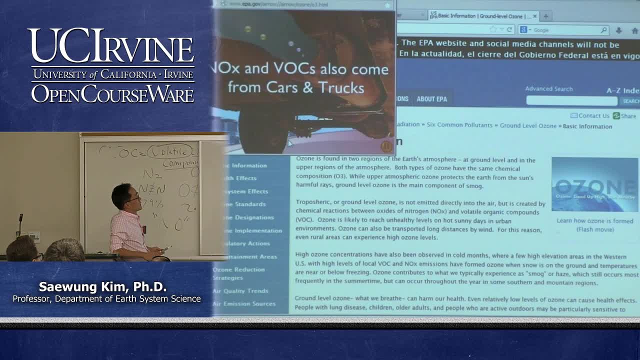 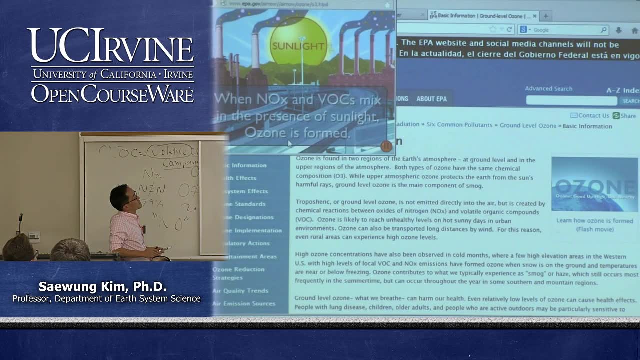 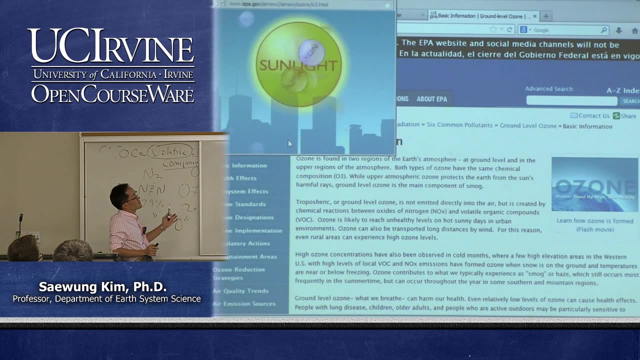 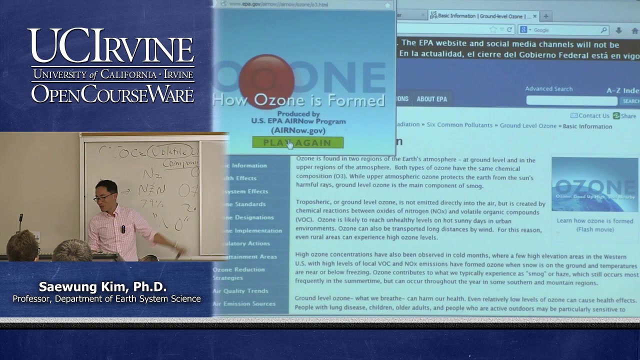 And then cars are emitting NOx and VOC. And then, on the sunlight, ozone is formed by chemical reactions. sun and NOx, VOC, boom, That's the reaction. right, Then make ozone. If you go this far, there's no problem, you are getting B okay. 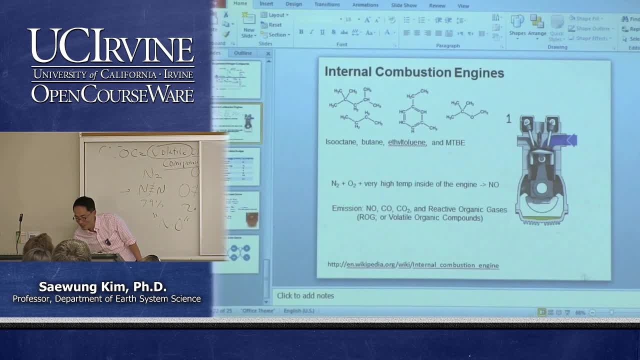 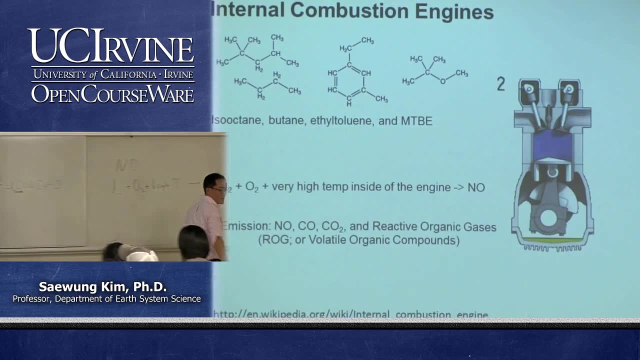 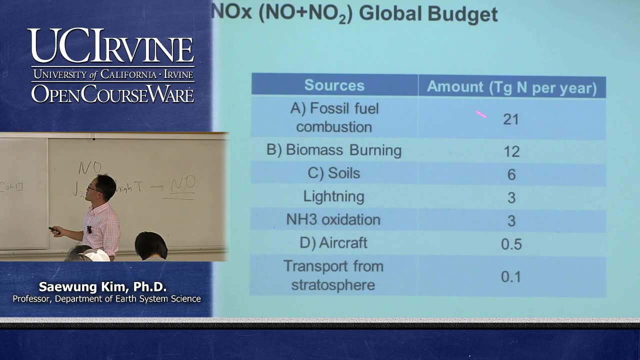 So this is peace in your mind before we dive into the chemical reaction. So the problem is the excess amount of NO and NO2 coming from the car engine, right? So this is a global budget, So a lot of NO and NO2, NOx, is coming from fossil fuel combustion, from the engine and 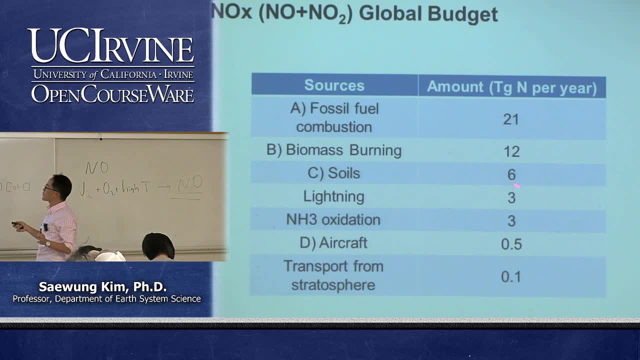 factory things like that. So there's some amount of the NO, and NO2 is actually from soil, but the micro-BR activity And then biomass is burning. It is real tricky if the biomass burning is caused by the human activity, that can be pollution. 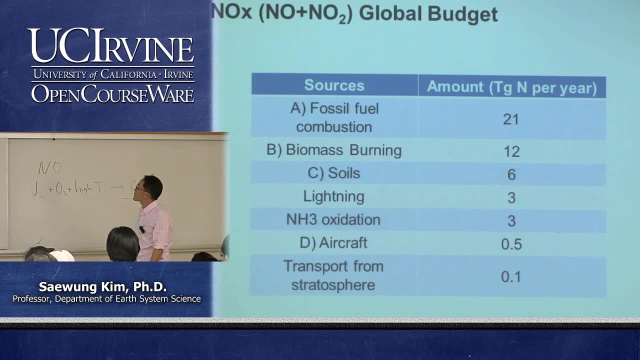 but there's a natural biomass burning such as lightning can cause the biomass burning. So in this case that's the natural processes, Also lightning, making the some NO and NO2.. So there are natural base of the NO and NO2 concentration there. 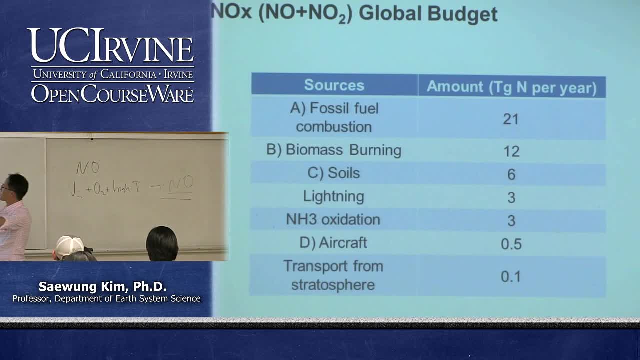 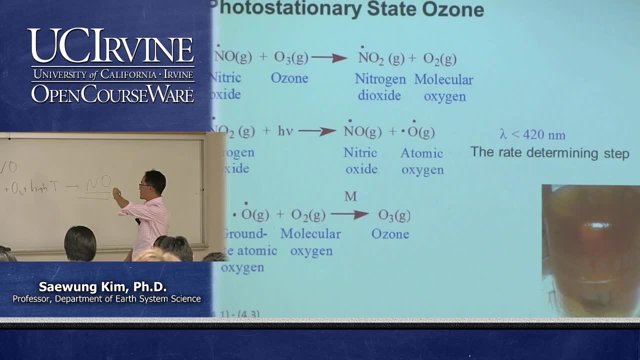 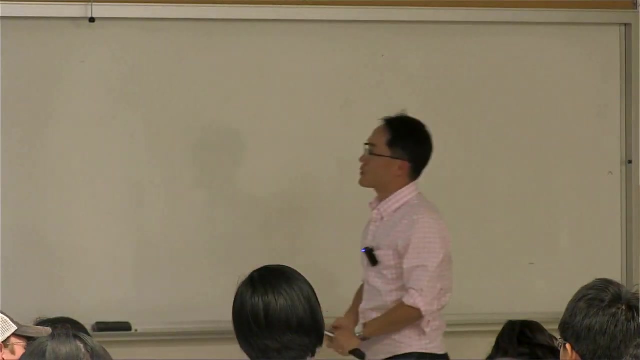 But the problem we have, the excess amount of ozone, is actually coming from this fossil fuel combustion. So I have 15 minutes to explain this thing. So these are main chemical reaction of ozone formation in the air that we breathe, what we call a troposphere. 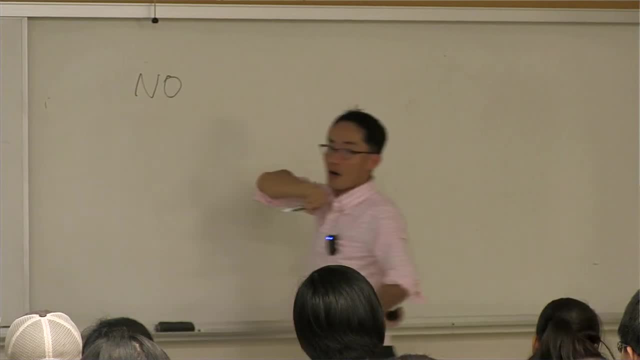 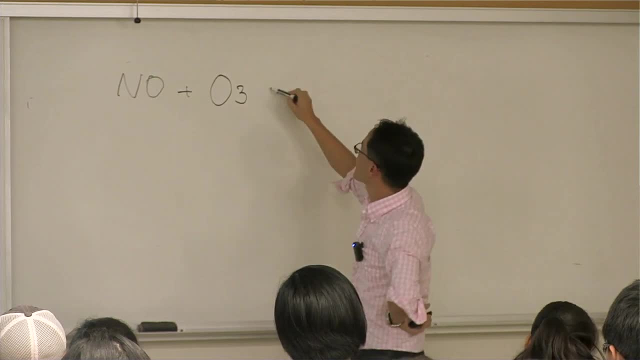 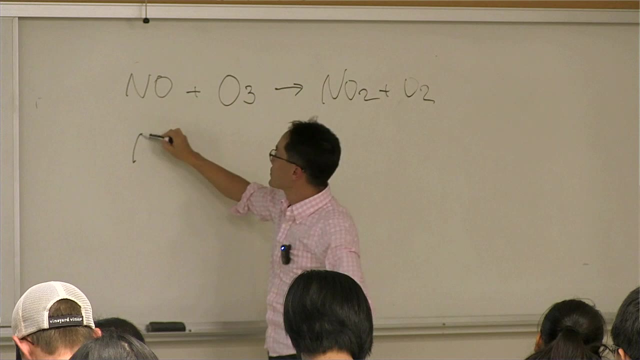 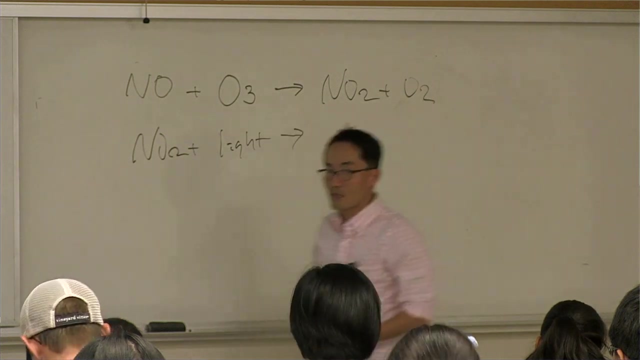 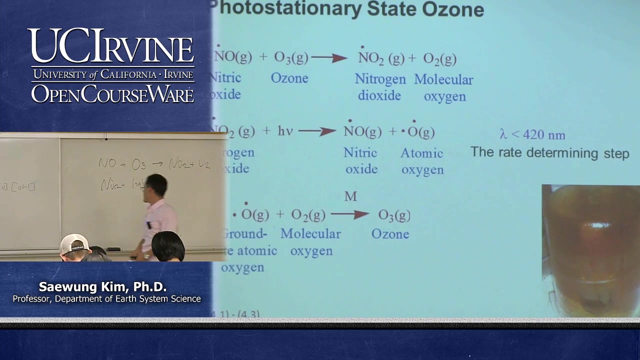 NO2.. NO2.. REACTED WITH OZONE, THEN MAKE NO2 PLUS O2. NO2.. IT'S LIGHT. SO WE DISCUSSED ABOUT NO2, COLOR OF NO2 IS BROWN RIGHT, AND THEN IN A VISIBLE WAVE. 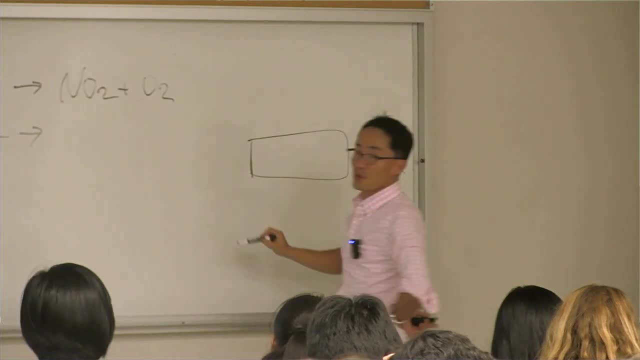 LENGTH. ONE OF QUICKLY, ONE OF QUICKLY, ONE OF QUICKLY. ANOTHER QUESTION WAS ABOUT THIS. ANOTHER QUESTION WAS ABOUT THIS. ANOTHER QUESTION WAS ABOUT THIS: SO VISIBLE WAVE LENGTH REGION. SO VISIBLE WAVE LENGTH REGION. 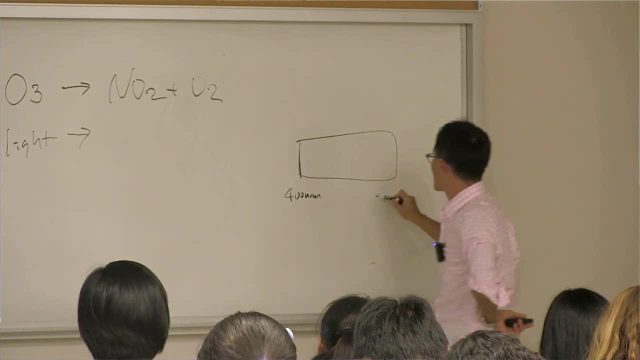 SO VISIBLE WAVE LENGTH REGION IS ABOUT 400. NANOMETER IS ABOUT 400. NANOMETER IS ABOUT 400. NANOMETER TO ABOUT 750 NANOMETER TO ABOUT 750 NANOMETER TO ABOUT 750 NANOMETER, THEN NO2 ACTUALLY OBSERVED. 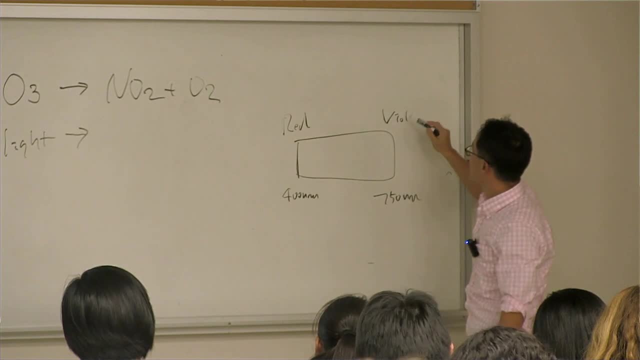 THEN NO2 ACTUALLY OBSERVED, THEN NO2 ACTUALLY OBSERVED. SO THIS IS RED, SO THIS IS RED, SO THIS IS RED, AND THEN THIS IS VIOLET, AND THEN THIS IS VIOLET AND THEN THIS IS VIOLET. NO, NO, NO, THE OTHER WAY AROUND. 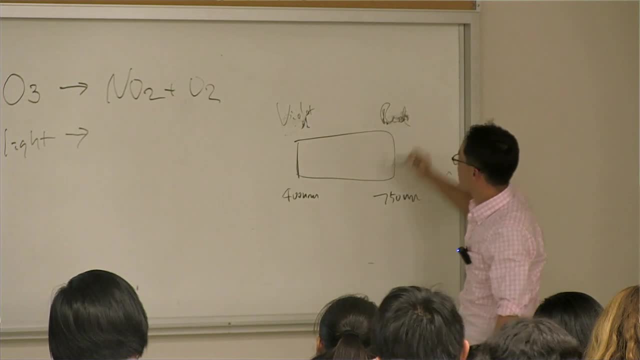 NO, NO, NO, THE OTHER WAY AROUND. NO, NO, NO, THE OTHER WAY AROUND. VIOLET AND RED, VIOLET AND RED, VIOLET AND RED, AND THEN NO2 IS OBSERVING, AND THEN NO2 IS OBSERVING. 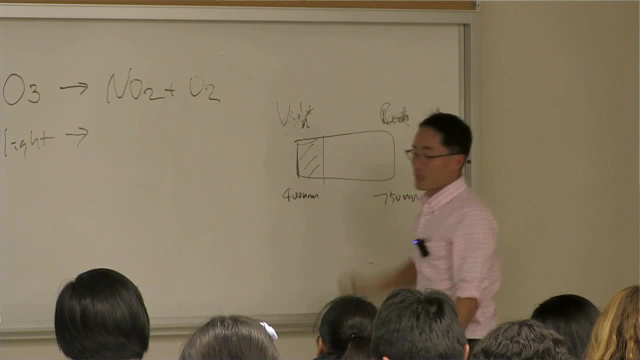 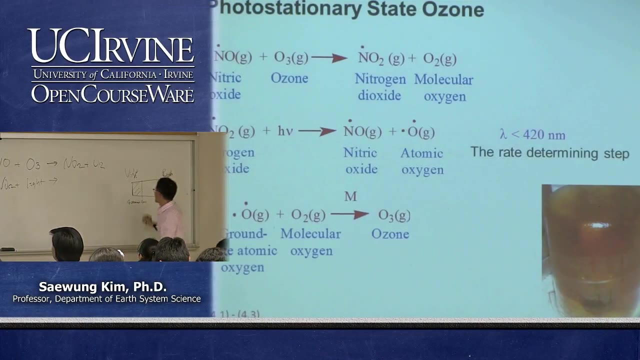 AND THEN NO2 IS OBSERVING. WAVE LENGTH BELOW 420.. WAVE LENGTH BELOW 420.. WAVE LENGTH BELOW 420.. THE REASON THIS LOOKS BROWN, THE REASON THIS LOOKS BROWN, THE REASON THIS LOOKS BROWN IS THAT BASICALLY THE LIGHT 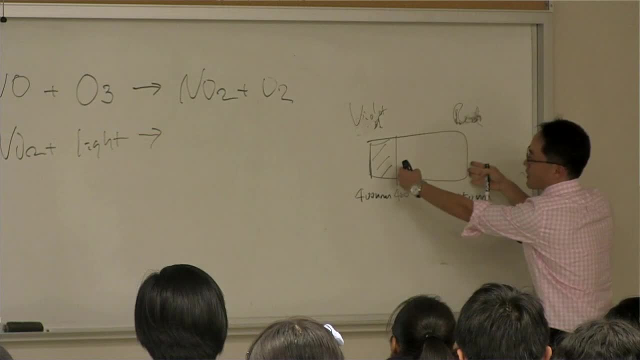 IS THAT BASICALLY THE LIGHT IS THAT BASICALLY THE LIGHT IS OBSERVED BY NO2 AND THEN IS OBSERVED BY NO2, AND THEN IS OBSERVED BY NO2, AND THEN, IF YOU JUST MIX THE OTHER, IF YOU JUST MIX THE OTHER, IF YOU JUST MIX THE OTHER WAVE. LENGTH LEFT OVER WAVE. 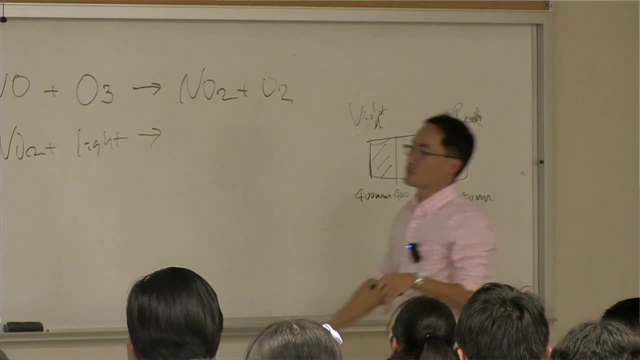 WAVE LENGTH LEFT OVER WAVE. WAVE LENGTH LEFT OVER WAVE. LENGTH FROM 420 TO 750, LENGTH FROM 420 TO 750, LENGTH FROM 420 TO 750,. IT JUST LOOKS LIKE BROWN RIGHT. IT JUST LOOKS LIKE BROWN RIGHT. 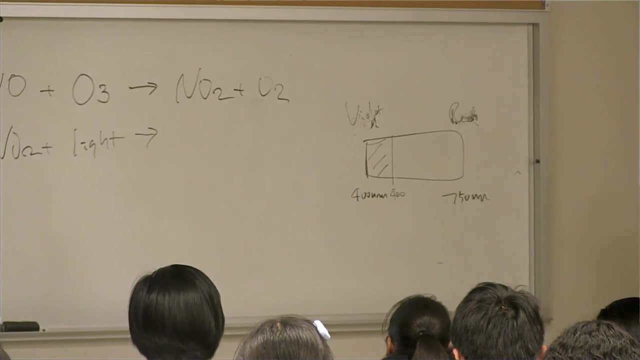 IT JUST LOOKS LIKE BROWN. RIGHT, IF YOU GET NEED OF THE VIOLET. IF YOU GET NEED OF THE VIOLET, IF YOU GET NEED OF THE VIOLET AND BLUE, THEN IT WILL LOOK, AND BLUE, THEN IT WILL LOOK. 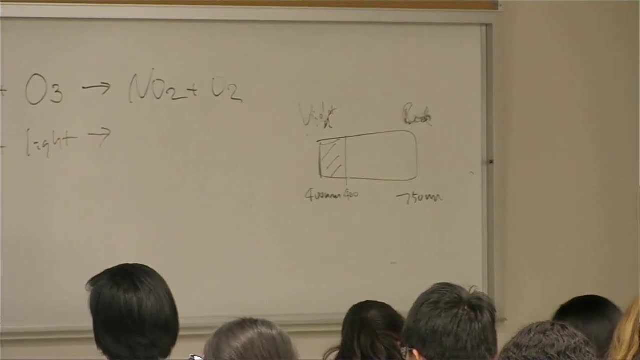 AND BLUE, THEN IT WILL LOOK LIKE BROWN, LIKE BROWN, LIKE BROWN. SO WHAT THAT WHAT IS HAPPENING. SO WHAT THAT? WHAT IS HAPPENING. SO WHAT THAT? WHAT IS HAPPENING? ONCE THAT NO2 MOLECULE OBSERVES. 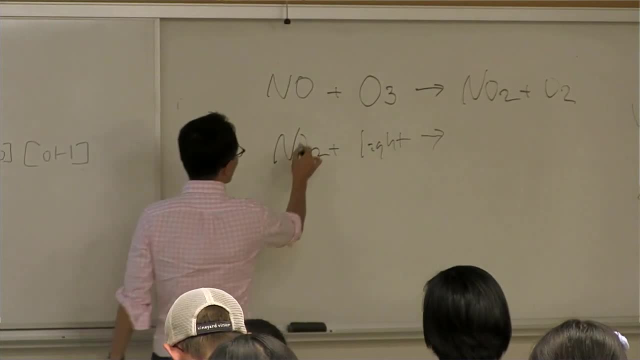 ONCE THAT NO2 MOLECULE OBSERVES, ONCE THAT NO2 MOLECULE OBSERVES THE LIGHT WAVE LENGTH BELOW 420, THE LIGHT WAVE LENGTH BELOW 420, THE LIGHT WAVE LENGTH BELOW 420, IT'S GOING TO BE DECOMPOSED. 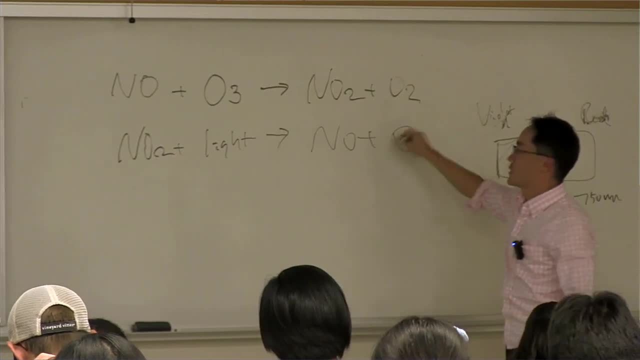 IT'S GOING TO BE DECOMPOSED. IT'S GOING TO BE DECOMPOSED INTO: NO PLUS OXYGENATUM. INTO NO PLUS OXYGENATUM. INTO- NO PLUS OXYGENATUM. ALL RIGHT, ALL RIGHT. 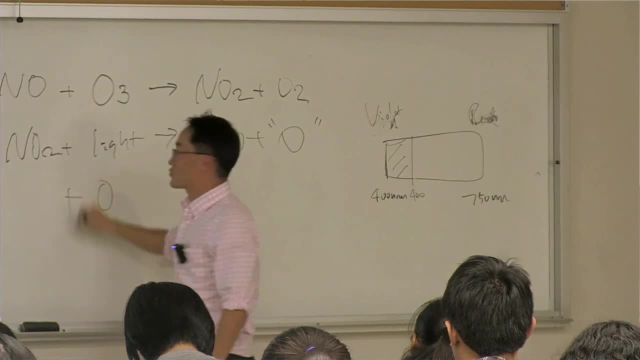 ALL RIGHT, THEN WHAT THIS THING IS GOING, THEN WHAT THIS THING IS GOING, THEN WHAT THIS THING IS GOING TO BE DOING THERE'S 20% TO BE DOING THERE'S 20% TO BE DOING THERE'S 20% OF MOLECULAR OXYGEN. 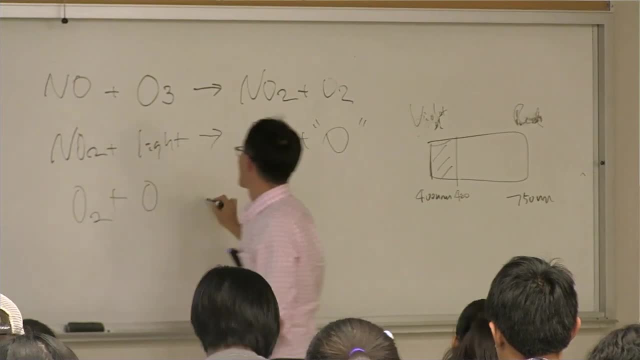 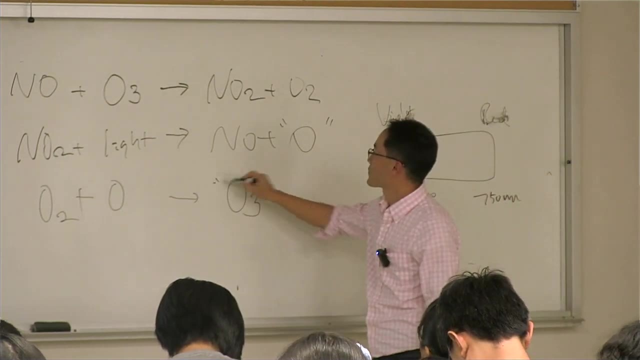 OF MOLECULAR OXYGEN, OF MOLECULAR OXYGEN IN THE ATOM SPHERE, IN THE ATOM SPHERE, IN THE ATOM SPHERE, IT'S MAKING OZONE, IT'S MAKING OZONE, IT'S MAKING OZONE, SO THERE'S OZONE. 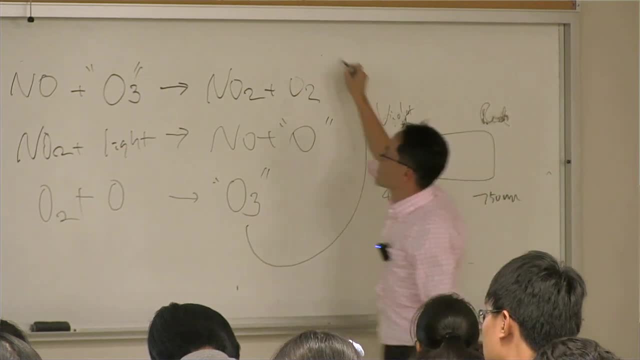 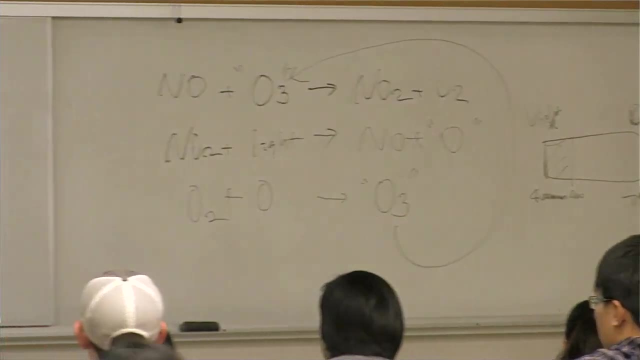 SO THERE'S OZONE, SO THERE'S OZONE. THERE'S OZONE RIGHT. THERE'S OZONE RIGHT. THERE'S OZONE RIGHT. IT CAN GO BACK RIGHT. IT CAN GO BACK RIGHT. IT CAN GO BACK RIGHT. BUT IF YOU LIKE, PUZZLE. 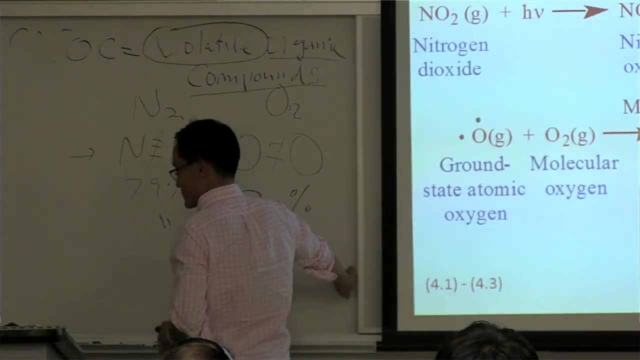 BUT IF YOU LIKE PUZZLE, BUT IF YOU LIKE PUZZLE, WHAT YOU CAN DO IS THAT A LITTLE TOO MUCH TODAY? IS THAT A LITTLE TOO MUCH TODAY? IS THAT A LITTLE TOO MUCH TODAY FOR ONE DAY? 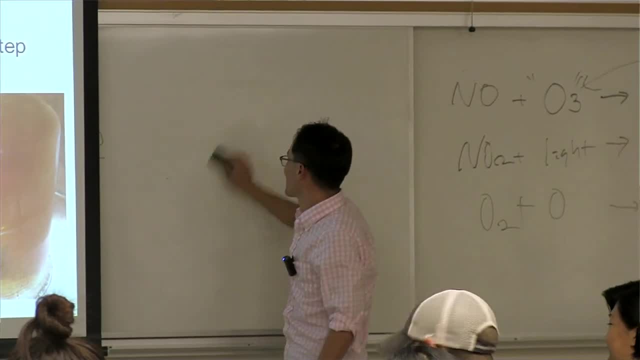 FOR ONE DAY. FOR ONE DAY. THIS IS THE LAST SLIDE THOUGH. THIS IS THE LAST SLIDE. THOUGH. THIS IS THE LAST SLIDE THOUGH. IS THAT OVERWHELMING? IS THAT OVERWHELMING? 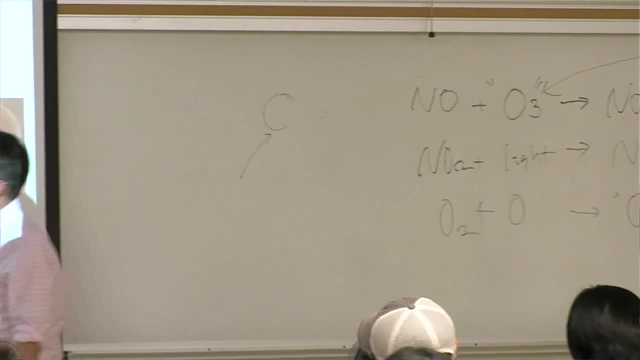 IS THAT OVERWHELMING- IT'S VERY QUIET AGAIN. THIS IS GOING TO BE AGAIN. THIS IS GOING TO BE AGAIN. THIS IS GOING TO BE THE MOST DIFFICULT STUFF. THE MOST DIFFICULT STUFF. 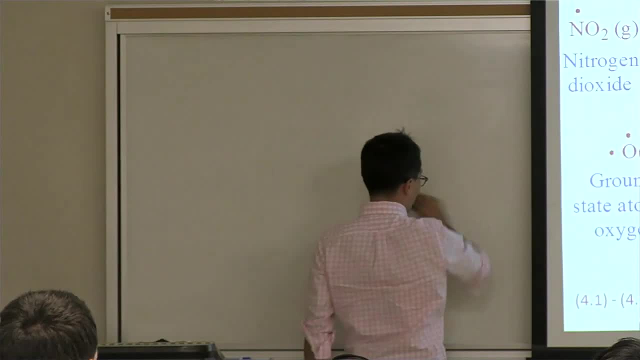 THE MOST DIFFICULT STUFF DURING THE WHOLE CLASS. DURING THE WHOLE CLASS, DURING THE WHOLE CLASS. SO DON'T GET FREAKED OUT. SO DON'T GET FREAKED OUT. SO DON'T GET FREAKED OUT, IT WILL BE NATURAL. 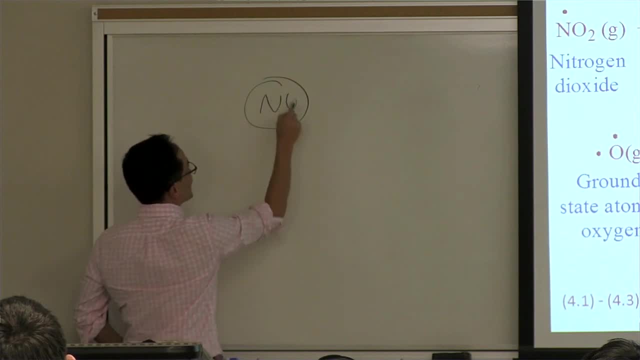 AGAIN. THIS ALL STARTS WITH NO. AGAIN. THIS ALL STARTS WITH NO AGAIN. THIS ALL STARTS WITH NO. THAT LITTLE VIDEO- THINGY THAT LITTLE VIDEO- THINGY THAT LITTLE VIDEO THINGY THAT I SHOWED YOU FROM THE EPA. 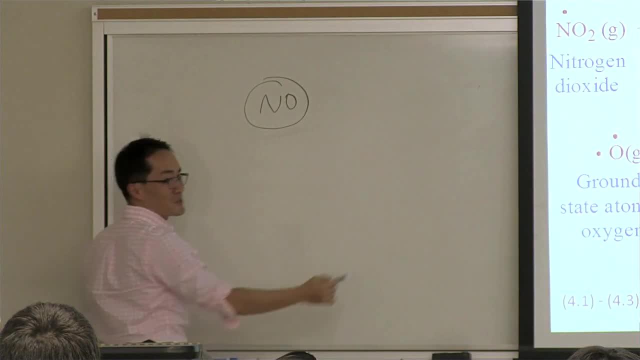 THAT I SHOWED YOU FROM THE EPA, THAT I SHOWED YOU FROM THE EPA: WEBSITE BOOM, WEBSITE BOOM, WEBSITE BOOM. AND THAT'S THE ORIGIN RIGHT. AND THAT'S THE ORIGIN RIGHT. 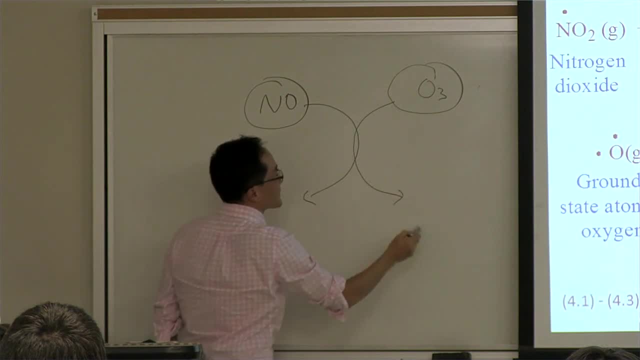 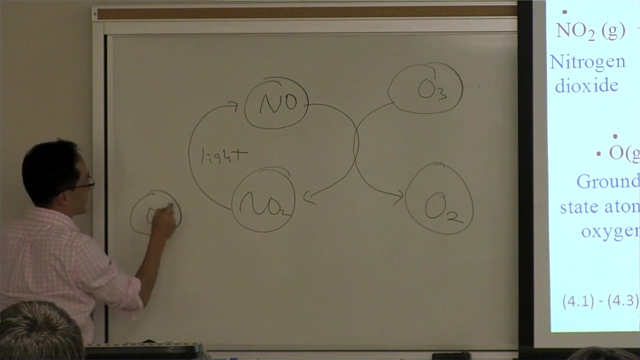 AND THAT'S THE ORIGIN, RIGHT. AND THEY ARE REACTING, AND THEY ARE REACTING, AND THEY ARE REACTING. EACH OTHER IN THE ATMOSPHERE, EACH OTHER IN THE ATMOSPHERE, EACH OTHER IN THE ATMOSPHERE, ALL RIGHT. 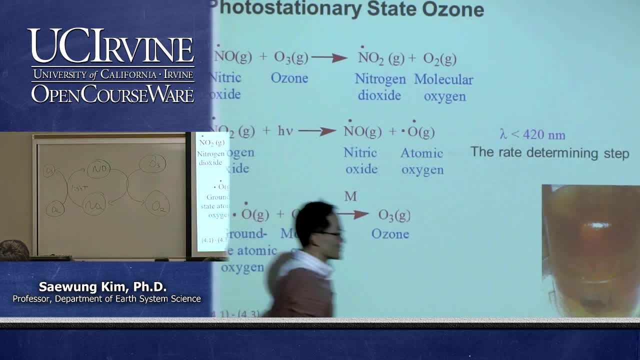 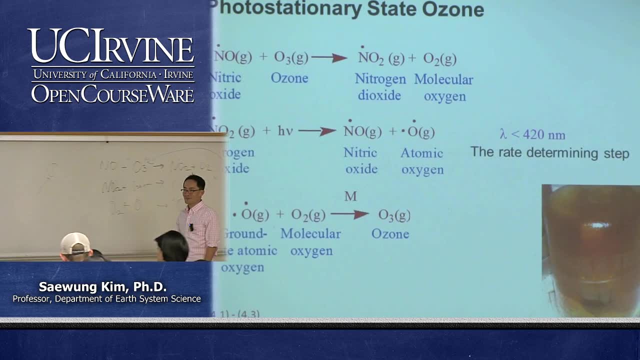 ALL RIGHT, ALL RIGHT. IF YOU DON'T LIKE THIS NOTATION. IF YOU DON'T LIKE THIS NOTATION, IF YOU DON'T LIKE THIS NOTATION, YOU CAN REMEMBER LIKE THIS. YOU CAN REMEMBER LIKE THIS. YOU CAN REMEMBER LIKE THIS, RIGHT. 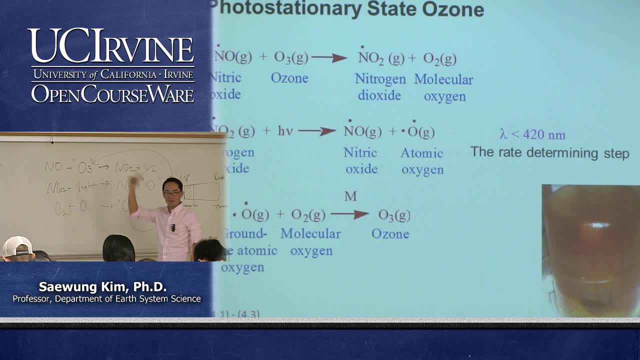 RIGHT, RIGHT, IF YOU HATE THE NOTATION, IF YOU HATE THE NOTATION, IF YOU HATE THE NOTATION, JUST WATCH THAT EPA, JUST WATCH THAT EPA, JUST WATCH THAT EPA, THAT BOOM, BOOM THING. OKAY, 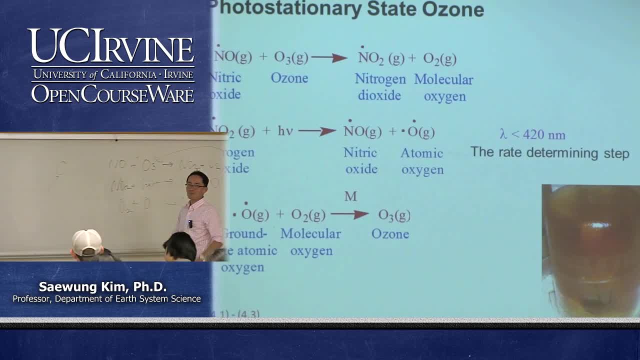 THAT BOOM BOOM THING. OKAY, THAT BOOM BOOM THING. OKAY, THAT'S ALL INSIDE, BUT, THAT'S ALL INSIDE, BUT. THAT'S ALL INSIDE. BUT DEPENDS ON YOUR UNDERSTANDING. DEPENDS ON YOUR UNDERSTANDING. DEPENDS ON YOUR UNDERSTANDING. I'M FINE WITH ANY UNDERSTANDING. I'M FINE WITH ANY UNDERSTANDING. I'M FINE WITH ANY UNDERSTANDING THAT YOU WILL HAVE. THAT YOU WILL HAVE. 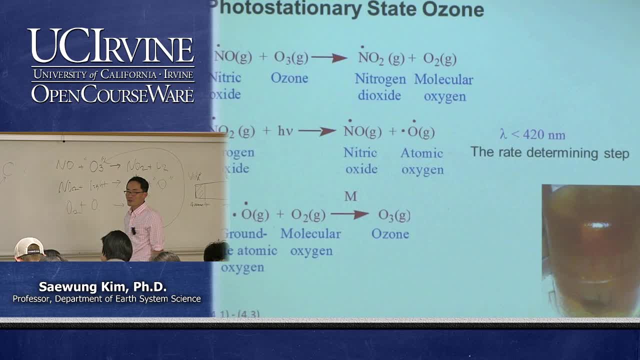 THAT YOU WILL HAVE, BUT THIS IS ACTUAL CHEMISTRY. BUT THIS IS ACTUAL CHEMISTRY. BUT THIS IS ACTUAL CHEMISTRY. THAT'S GOING ON IN THE ATOMOSPHERE. THAT'S GOING ON IN THE ATOMOSPHERE. 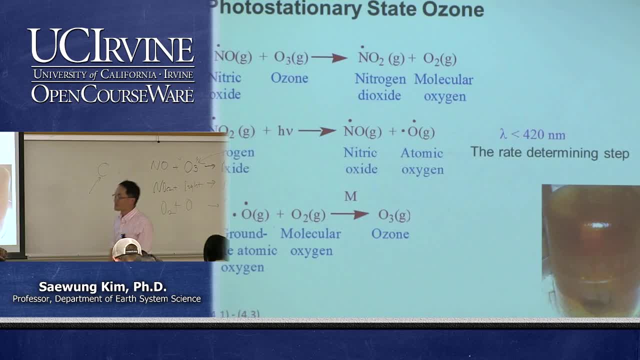 THAT'S GOING ON IN THE ATOMOSPHERE. BUT YOU CAN JUST UNDERSTAND, BUT YOU CAN JUST UNDERSTAND. BUT YOU CAN JUST UNDERSTAND. THIS BUBBLE DIAGRAM, ALL RIGHT. THIS BUBBLE DIAGRAM, ALL RIGHT. 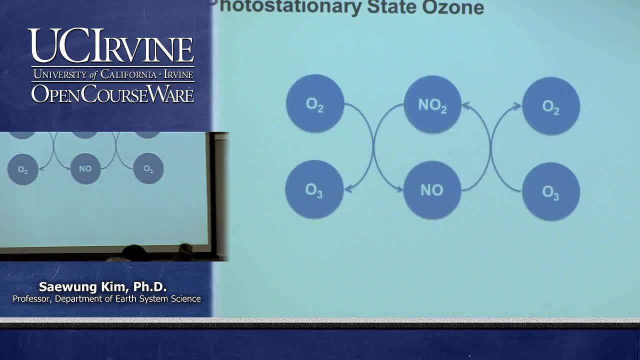 THIS BUBBLE DIAGRAM, ALL RIGHT. SO IF YOU TAKE A LOOK AT, SO, IF YOU TAKE A LOOK AT, SO, IF YOU TAKE A LOOK AT THIS THING, SO THAT'S BASICALLY THIS THING, SO THAT'S BASICALLY THIS THING, SO THAT'S BASICALLY THE LAST SLIDE HERE. THE LAST SLIDE HERE. THE LAST SLIDE HERE. SO IF YOU TAKE A LOOK AT, SO, IF YOU TAKE A LOOK AT SO, IF YOU TAKE A LOOK AT THIS THING, WHAT'S ACTUALLY, THIS THING, WHAT'S ACTUALLY. 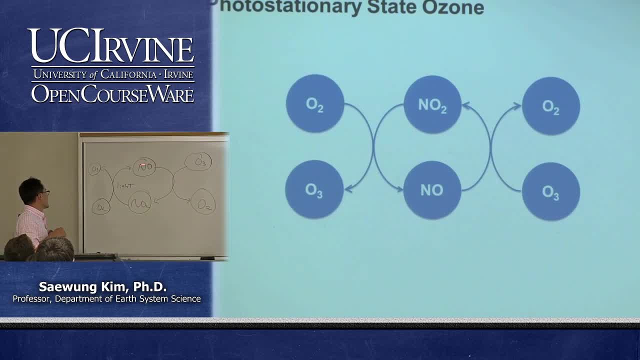 THIS THING WHAT'S ACTUALLY GOING ON? IS THAT THERE'S ANO GOING ON? IS THAT THERE'S ANO GOING ON? IS THAT THERE'S ANO IN THE ATOMOSPHERE, IN THE ATOMOSPHERE, IN THE ATOMOSPHERE, IT JUST KEEPS CYCLING RIGHT. 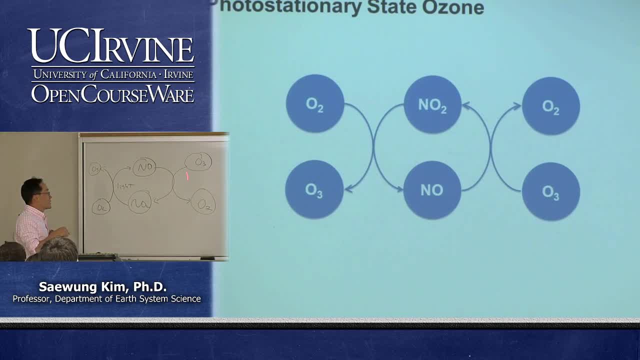 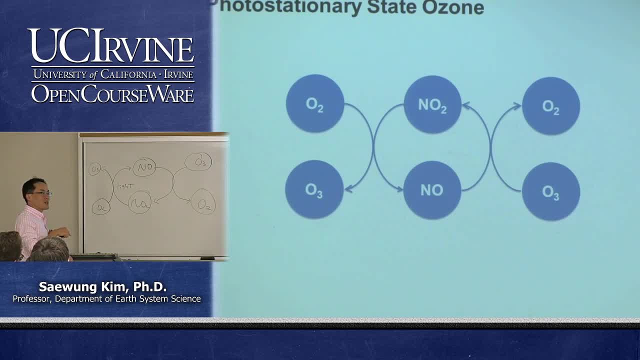 CYCLE IS DOING IS THAT PRODUCING OZONE AND THEN PRODUCING OZONE AND THEN PRODUCING OZONE, AND THEN DESTROYING OZONE AT THE SAME. DESTROYING OZONE AT THE SAME, DESTROYING OZONE AT THE SAME TIME. 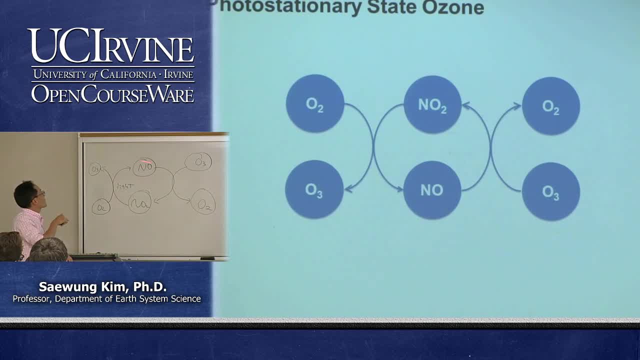 TIME, TIME. SO THIS IS THE MAIN CYCLE. SO THIS IS THE MAIN CYCLE. SO THIS IS THE MAIN CYCLE. SO KEEP JUST KIND OF ROLLING ON, SO KEEP JUST KIND OF ROLLING ON. SO KEEP JUST KIND OF ROLLING ON THEN IN THIS PART OF THE CYCLE. 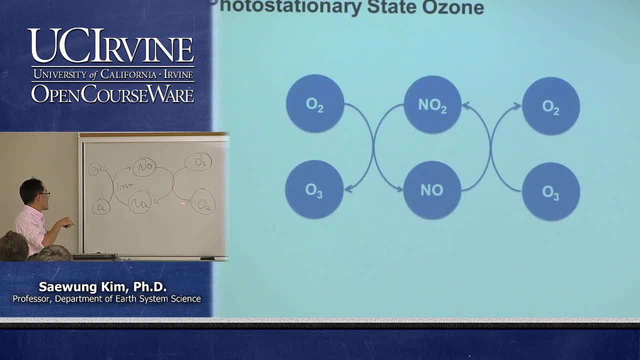 THEN IN THIS PART OF THE CYCLE, THEN IN THIS PART OF THE CYCLE OZONE GETS PRODUCED, OZONE GETS PRODUCED, OZONE GETS PRODUCED, AND THEN IN THIS SIDE OF CYCLE. 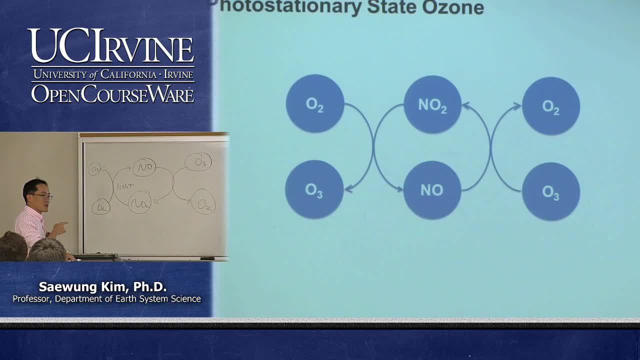 AND THEN IN THIS SIDE OF CYCLE, AND THEN IN THIS SIDE OF CYCLE. OZONE IS REMOVED- RIGHT. OZONE IS REMOVED- RIGHT. OZONE IS REMOVED- RIGHT. THAT'S WHAT'S GOING ON. 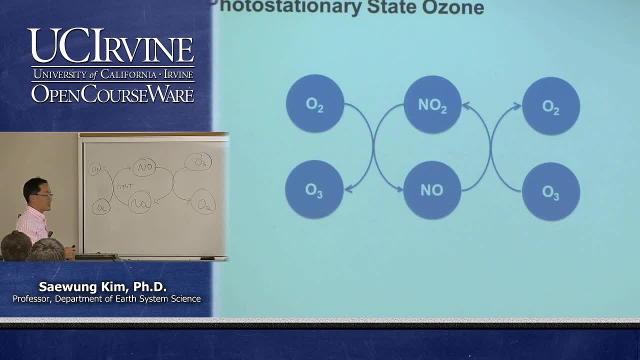 THAT'S WHAT'S GOING ON. THAT'S WHAT'S GOING ON. SO, OH, BOY, SO, OH, BOY, SO, OH, BOY, SO DEPRESSING THIS, SO DEPRESSING THIS, SO DEPRESSING THIS. IF YOU LOOK AT YOUR FACE. 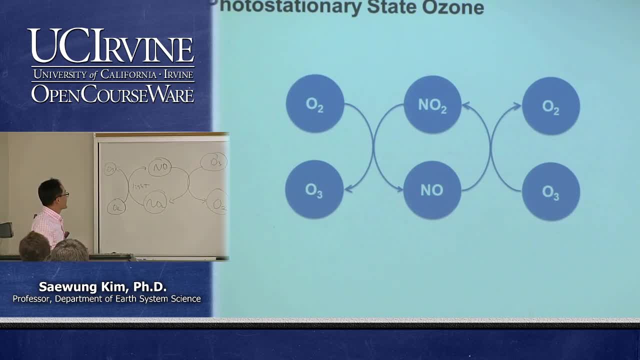 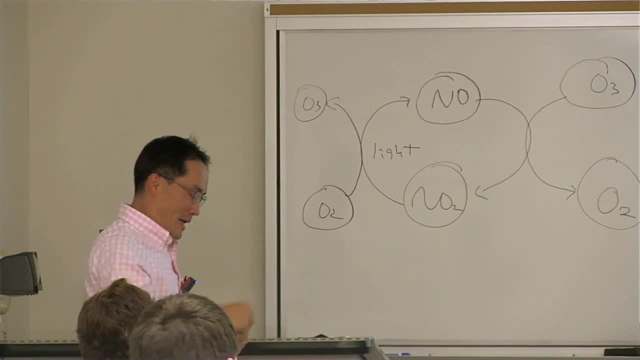 IF YOU LOOK AT YOUR FACE? IF YOU LOOK AT YOUR FACE, EVERYBODY'S SO, EVERYBODY'S SO, EVERYBODY'S SO. SO, LET'S JUST TAKE A LOOK. SO, LET'S JUST TAKE A LOOK. SO, LET'S JUST TAKE A LOOK AT THIS THING, OKAY? 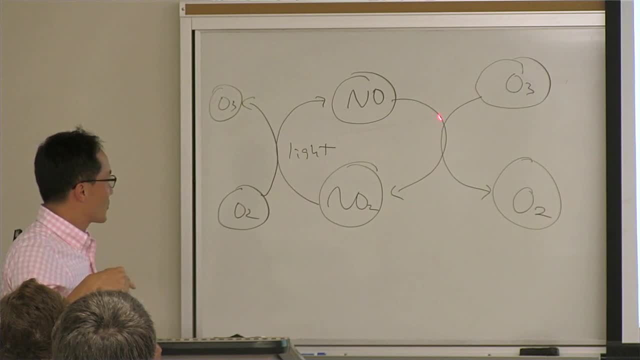 AT THIS THING, OKAY. AT THIS THING, OKAY. SO THIS CYCLING IS GOING TO KEEP. SO THIS CYCLING IS GOING TO KEEP. SO THIS CYCLING IS GOING TO KEEP GOING. AND THEN THERE'S A RIGHT. 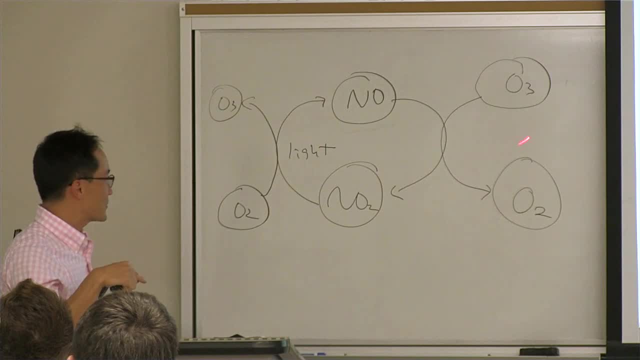 GOING, AND THEN THERE'S A RIGHT GOING, AND THEN THERE'S A RIGHT. SO OZONE IS GOING TO PRODUCE, SO OZONE IS GOING TO PRODUCE. SO OZONE IS GOING TO PRODUCE FROM THIS SIDE OF THE CYCLE. FROM THIS SIDE OF THE CYCLE, FROM THIS SIDE OF THE CYCLE, OZONE IS GOING TO BE. OZONE IS GOING TO BE. OZONE IS GOING TO BE DECOMPOSED BY THIS PART OF THE, DECOMPOSED BY THIS PART OF THE. 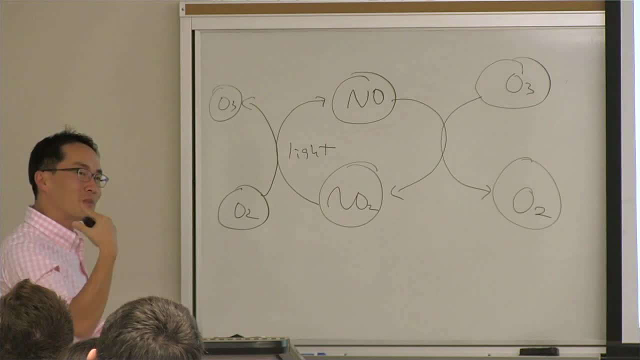 DECOMPOSED BY THIS PART OF THE CYCLE: RIGHT, CYCLE, RIGHT, CYCLE, RIGHT. SO WHICH MEANS THAT THERE IS A SO WHICH MEANS THAT THERE IS A SO WHICH MEANS THAT THERE IS A HAPPY MIDDLE GROUND OF THE OZONE. 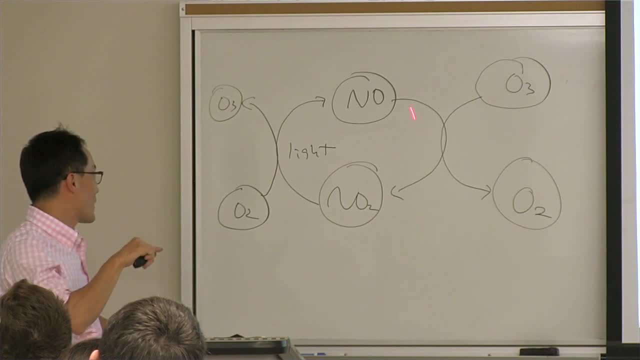 HAPPY MIDDLE GROUND OF THE OZONE. HAPPY MIDDLE GROUND OF THE OZONE. CONCENTRATION IN THE ATMOSPHERE. CONCENTRATION IN THE ATMOSPHERE. CONCENTRATION IN THE ATMOSPHERE. IF THERE IS THE RIGHT AMOUNT OF 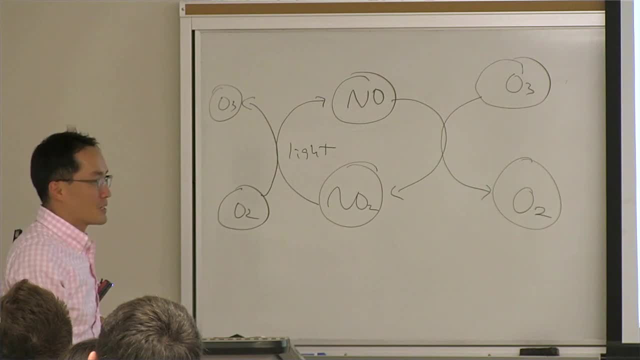 IF THERE IS THE RIGHT AMOUNT OF, IF THERE IS THE RIGHT AMOUNT OF NO AND NO2 IN THE ATMOSPHERE, NO AND NO2 IN THE ATMOSPHERE, NO AND NO2 IN THE ATMOSPHERE. SO I'M NOT GOING TO SOLVE THAT. 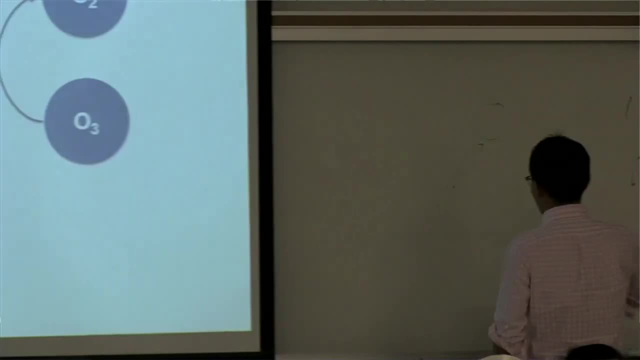 SO I'M NOT GOING TO SOLVE THAT. SO I'M NOT GOING TO SOLVE THAT. EQUATION OF THE HAPPY OZONE. EQUATION OF THE HAPPY OZONE. EQUATION OF THE HAPPY OZONE. CONCENTRATION TODAY OR NOT EVEN. 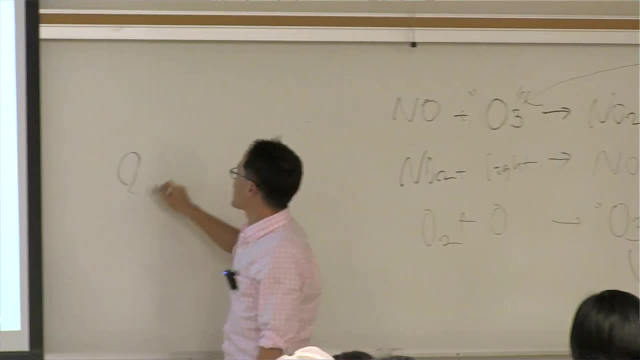 CONCENTRATION TODAY OR NOT EVEN. CONCENTRATION TODAY OR NOT EVEN, DURING THE WHOLE CLASS. DURING THE WHOLE CLASS, DURING THE WHOLE CLASS. THAT'S ABOUT 20 TO 40 ppb. THAT'S ABOUT 20 TO 40 ppb. 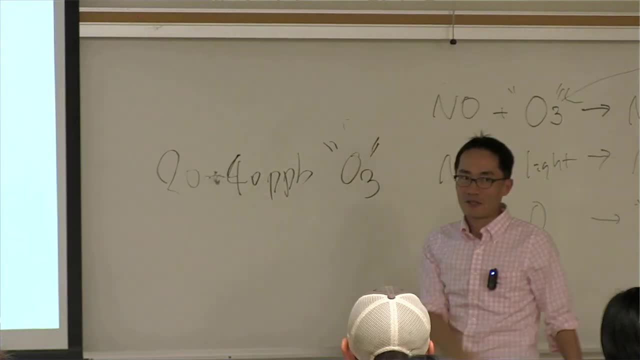 THAT'S ABOUT 20 TO 40 ppb OF OZONE, OF OZONE, OF OZONE. SO THIS IS HEALTHY LEVEL OF OZONE. SO THIS IS HEALTHY LEVEL OF OZONE. SO THIS IS HEALTHY LEVEL OF OZONE. BECAUSE, LET'S GO BACK ALL. 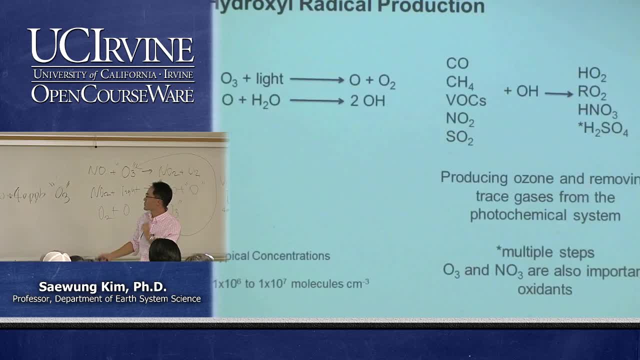 BECAUSE, LET'S GO BACK ALL BECAUSE, LET'S GO BACK ALL THE WAY, THE WAY, THE WAY WHY WE NEED OZONE IN THE WHY WE NEED OZONE IN THE WHY WE NEED OZONE IN THE ATMOSPHERE, ATMOSPHERE. 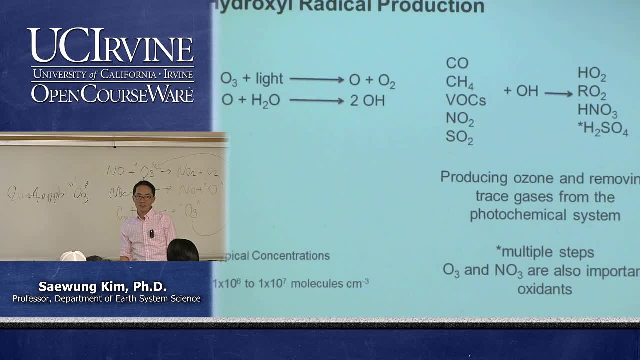 ATMOSPHERE. WE DON'T WANT TO HAVE THIS AIR. WE DON'T WANT TO HAVE THIS AIR. WE DON'T WANT TO HAVE THIS AIR. POLLUTANCE IN THE ATMOSPHERE. POLLUTANCE IN THE ATMOSPHERE. POLLUTANCE IN THE ATMOSPHERE. SO HOW WE CAN GET RID OF THIS. 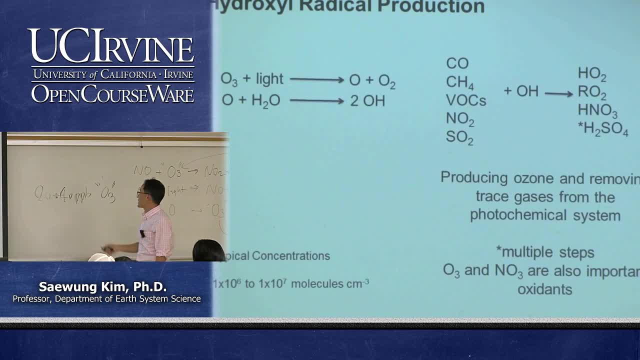 SO HOW WE CAN GET RID OF THIS. SO HOW WE CAN GET RID OF THIS. AIR POLLUTANCE IN THE ATMOSPHERE. AIR POLLUTANCE IN THE ATMOSPHERE. AIR POLLUTANCE IN THE ATMOSPHERE BY CHEMICAL REACTION WITH OH. 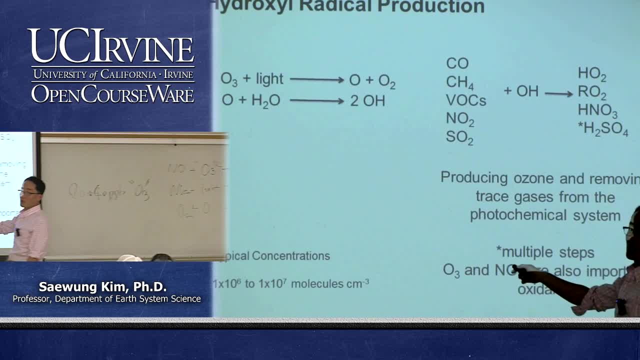 BY CHEMICAL REACTION WITH OH. BY CHEMICAL REACTION WITH OH. WHERE'S THE OH COMING FROM? WHERE'S THE OH COMING FROM? WHERE'S THE OH COMING FROM? IT'S FROM OZONE RIGHT. IT'S FROM OZONE RIGHT. 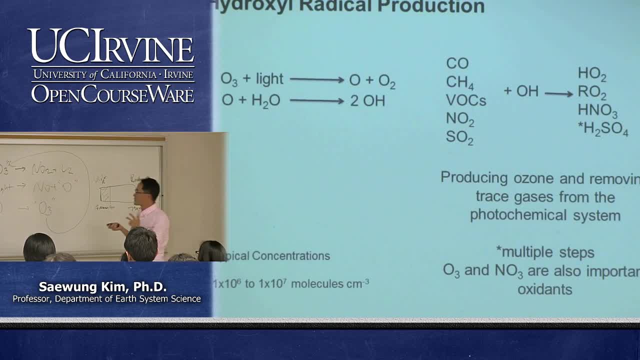 IT'S FROM OZONE RIGHT. SO WE WANT TO HAVE OZONE. SO WE WANT TO HAVE OZONE. SO WE WANT TO HAVE OZONE. RIGHT. AMOUNT OF OZONE. RIGHT. AMOUNT OF OZONE RIGHT. AMOUNT OF OZONE SOMEWHERE BETWEEN 20 TO 40 PPB. 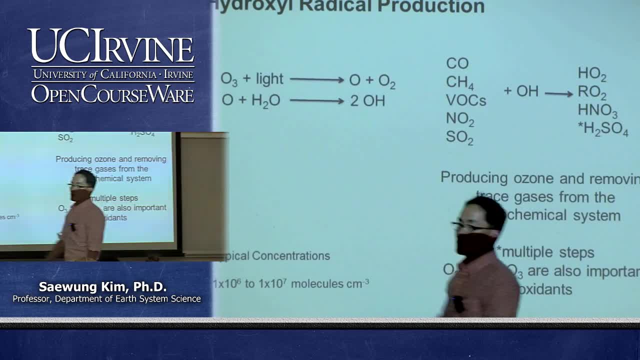 SOMEWHERE BETWEEN 20 TO 40 PPB, SOMEWHERE BETWEEN 20 TO 40 PPB, AND THEN THIS NATURAL CYCLE, AND THEN THIS NATURAL CYCLE, AND THEN THIS NATURAL CYCLE OF NON NO2.. OF NON NO2.. 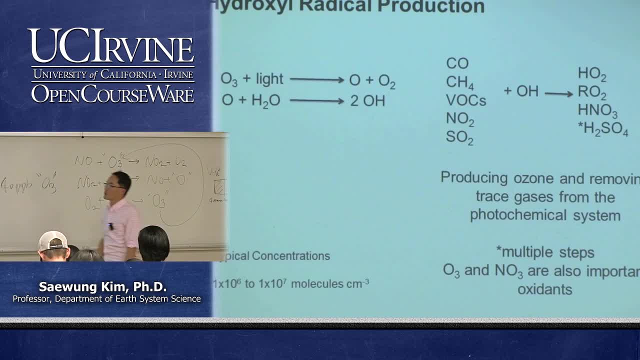 OF NON NO2.. AND THEN ALTHOUGH THERE'S NO EMISSION, AND THEN ALTHOUGH THERE'S NO EMISSION, AND THEN ALTHOUGH THERE'S NO EMISSION OF NON NO2 FROM CARS, OF NON NO2 FROM CARS. 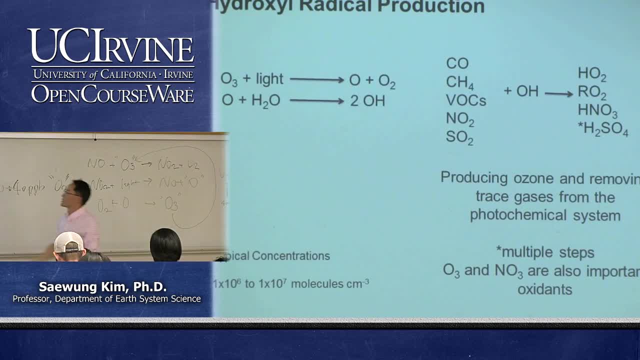 OF NON NO2 FROM CARS OR THE FACTORY EMISSION, OR THE FACTORY EMISSION OR THE FACTORY EMISSION THINGS LIKE THAT STILL THERE'S THINGS, LIKE THAT STILL THERE'S THINGS LIKE THAT STILL THERE'S A NATURAL EMISSION OF NON NO2. 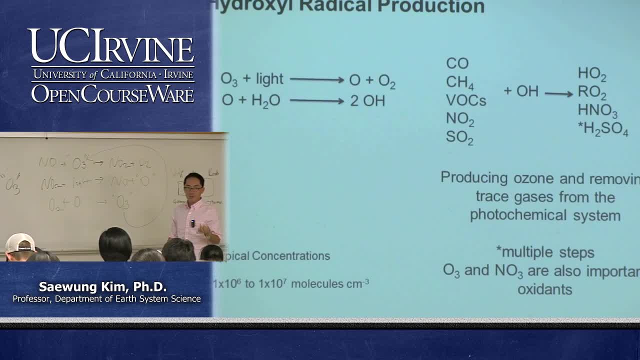 A NATURAL EMISSION OF NON NO2. A NATURAL EMISSION OF NON NO2 FROM LIGHTNING BIOMASS BURNING FROM LIGHTNING. BIOMASS BURNING FROM LIGHTNING BIOMASS BURNING CAUSED BY THEIR NATURAL CAUSE. CAUSED BY THEIR NATURAL CAUSE. CAUSED BY THEIR NATURAL CAUSE AND THEN SOIL EMISSION AND THEN SOIL EMISSION AND THEN SOIL EMISSION MAINTAINS HEALTHY LEVEL OF NO. MAINTAINS HEALTHY LEVEL OF NO. MAINTAINS HEALTHY LEVEL OF NO AND NO2 CONCENTRATION IN THE. 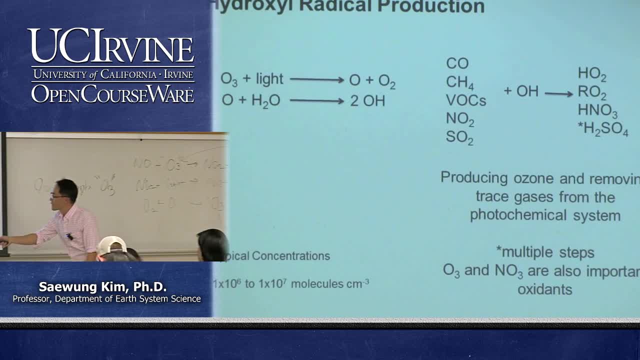 AND NO2 CONCENTRATION IN THE AND NO2 CONCENTRATION IN THE ATMOSPHERE. THAT DRIVES THIS ATMOSPHERE, THAT DRIVES THIS ATMOSPHERE, THAT DRIVES THIS CHEMICAL CYCLE, CHEMICAL CYCLE, CHEMICAL CYCLE AND THEN. I DON'T THINK THERE'S. 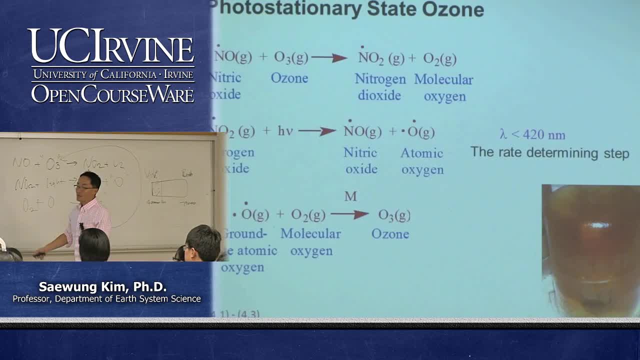 AND THEN I DON'T THINK THERE'S AND THEN I DON'T THINK THERE'S. MANY OF YOU ARE CHEMICALLY MANY OF YOU ARE CHEMICALLY MANY OF YOU ARE CHEMICALLY INCLINED PEOPLE BUT JUST IN: INCLINED PEOPLE, BUT JUST IN. INCLINED PEOPLE, BUT JUST IN CASE. THEN THERE'S A BUNCH OF CASE. THEN THERE'S A BUNCH OF CASE. THEN THERE'S A BUNCH OF REACTIONS GOING ON IN THE REACTIONS GOING ON IN THE. 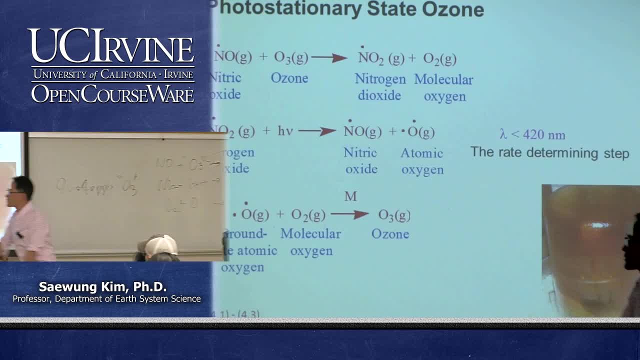 REACTIONS GOING ON IN THE ATMOSPHERE: ATMOSPHERE, ATMOSPHERE. YOU CAN SUMMARIZE THIS REACTION. YOU CAN SUMMARIZE THIS REACTION, YOU CAN SUMMARIZE THIS REACTION INTO THIS BUBBLE DIAGRAM, THAT'S. 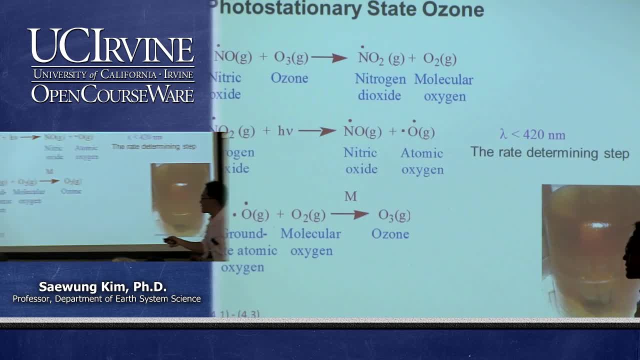 INTO THIS BUBBLE DIAGRAM THAT'S INTO THIS BUBBLE DIAGRAM THAT'S CYCLING OVER NNNO2, PRODUCING CYCLING OVER NNNO2, PRODUCING CYCLING OVER NNNO2, PRODUCING OZONE AND THEN DESTROYING. 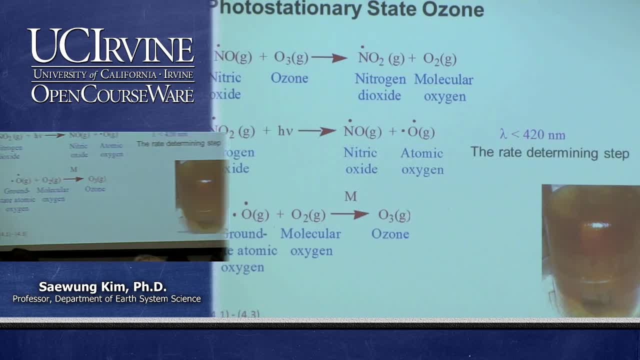 OZONE AND THEN DESTROYING OZONE, AND THEN DESTROYING OZONE, AND THEN IN THE NATURAL OZONE AND THEN IN THE NATURAL OZONE, AND THEN IN THE NATURAL CONDITION: THERE'S NO AIR. CONDITION: THERE'S NO AIR. 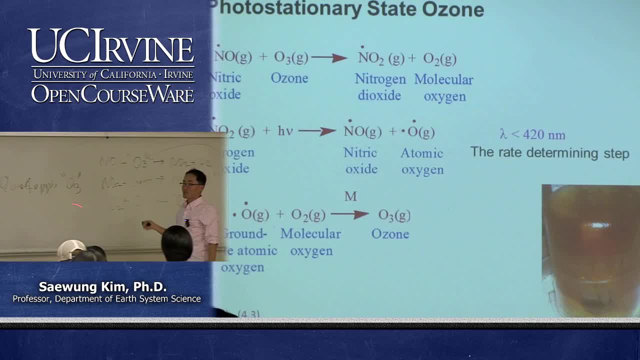 CONDITION: THERE'S NO AIR. POLLUTION IN THE ATMOSPHERE. POLLUTION IN THE ATMOSPHERE. POLLUTION IN THE ATMOSPHERE AND THEN OZONE CONCENTRATION AND THEN OZONE CONCENTRATION AND THEN OZONE CONCENTRATION IS GOING TO BE BETWEEN 20 TO 40. 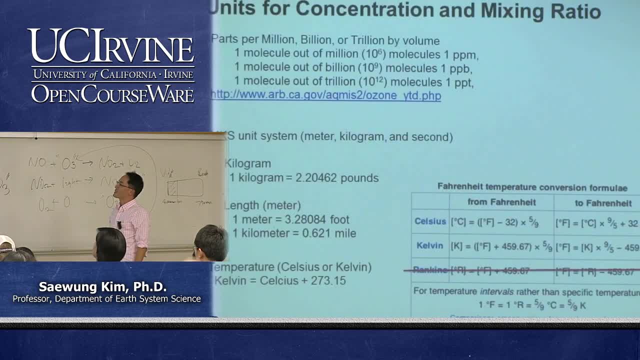 IS GOING TO BE BETWEEN 20 TO 40, IS GOING TO BE BETWEEN 20 TO 40 PPB, AND THEN THAT MAINTAINS PPB, AND THEN THAT MAINTAINS PPB, AND THEN THAT MAINTAINS HEALTHY LEVEL OF THE OH. 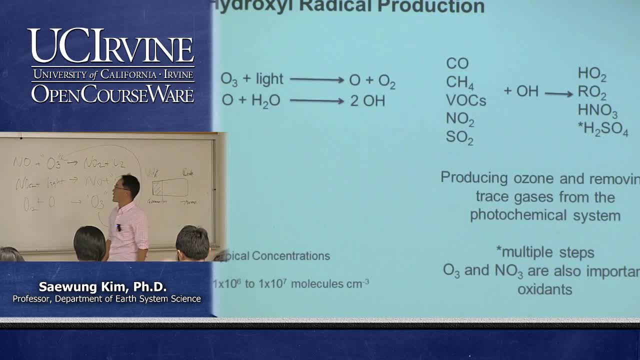 HEALTHY LEVEL OF THE OH. HEALTHY LEVEL OF THE OH. CONCENTRATION, CONCENTRATION, CONCENTRATION: WE CALL IT DETERGENT OF THE, WE CALL IT DETERGENT OF THE. WE CALL IT DETERGENT OF THE ATOMOSPHERE, OR CLEANER IN THE.